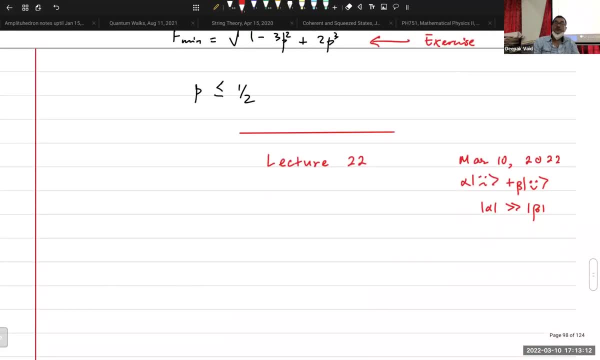 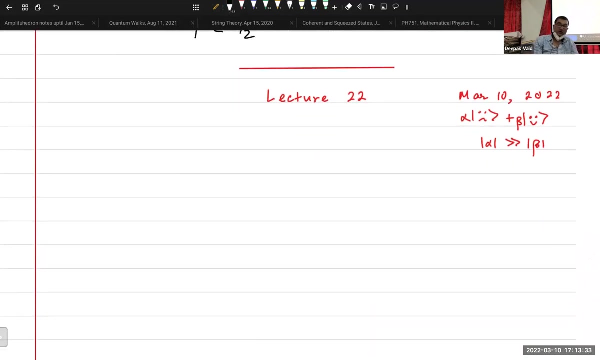 a description of how precisely do you measure these syndrome operators. right, In terms of a quantum circuit language. right, Because we want to have the precise circuit implementation of this error correcting code. right? So that is part of what I'll talk about today. 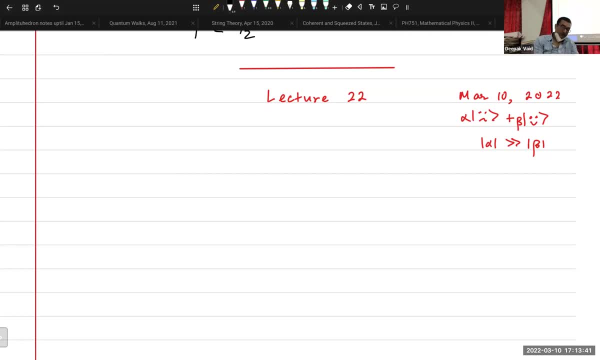 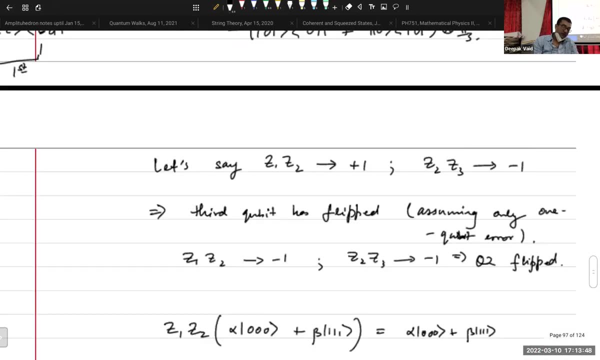 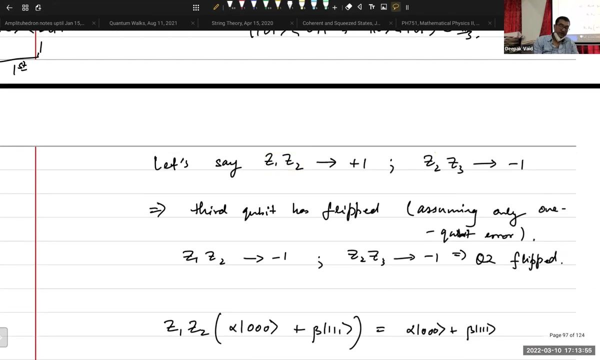 So let's start, So let me so right. And so what we also found was that these syndrome measurements can be also alternatively be expressed in terms of the action of these operators, Z1, Z2,, Z2, Z3, which allow us to compare individual qubits. right And so what? this is this. 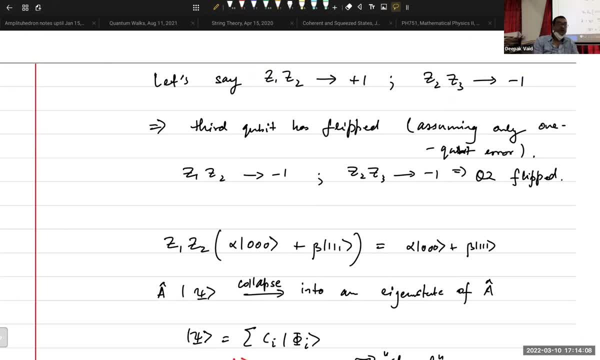 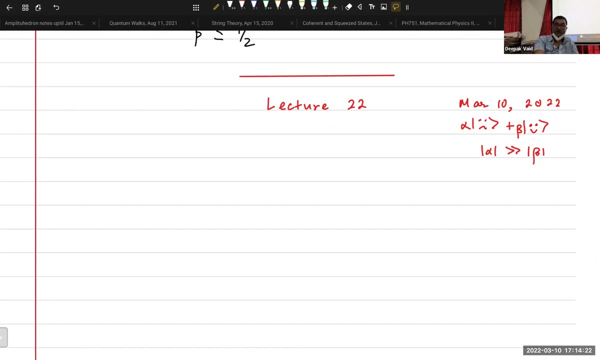 is a parity check. This is a parity check, right? Parity means if a bit, one bit, is the same as the other bit, you get plus one, otherwise you get minus one. So the question is: how do you perform a parity check on two qubits? 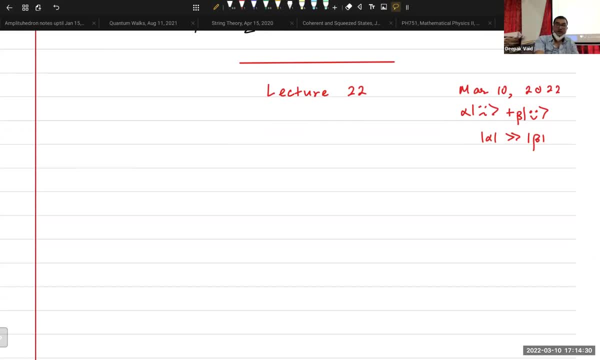 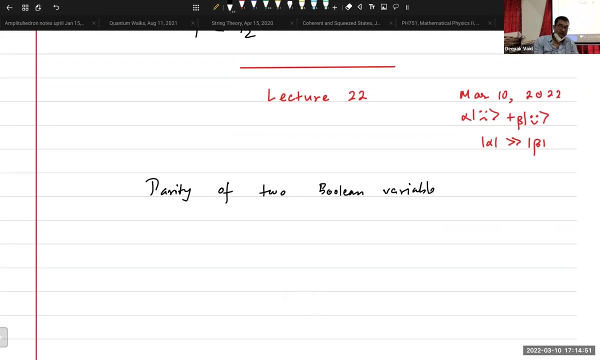 okay, Now, for this purpose, one can use a CNOT gate. So what is a parity? first of all, What is the definition of parity? Parity of two Boolean variables? I don't know if that's is that. is that visible? 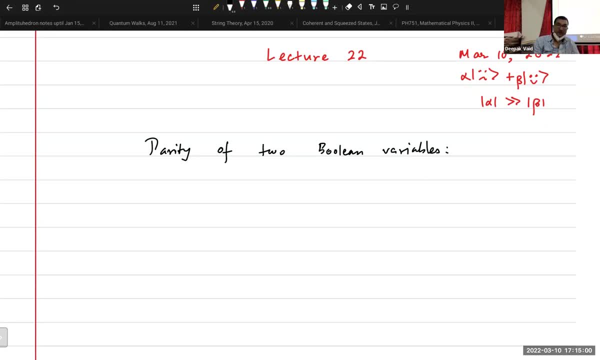 What I'm writing. Parity of two Boolean variables can be. is the XOR logical XOR. Okay. So, for example, if they're both A- B, right, both of them are zero. parity of A- B is zero. And if both of them are one parity of A- B- XOR B is zero, right For? 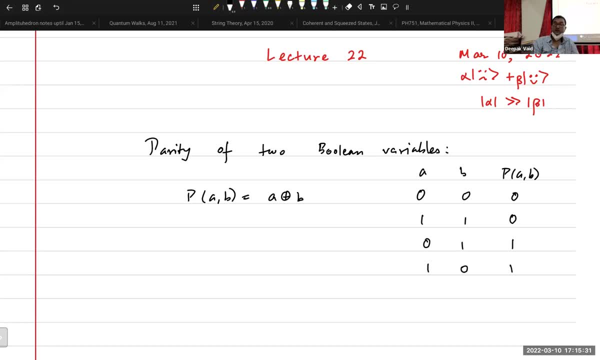 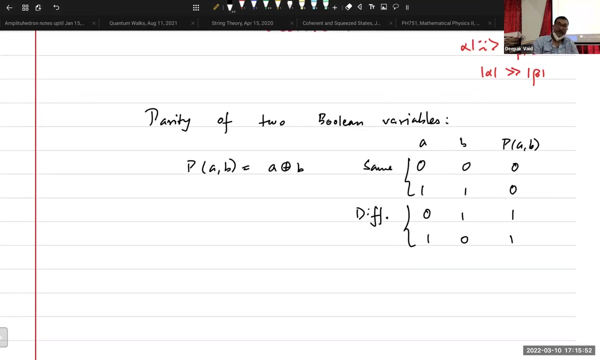 zero one, you get one. one zero, you get one right. So if both of them are the same, then the parity, this XOR, gives you zero. Otherwise it gives you one right. And we can implement this in a circuit using a CNOT gate right. Because what is the operation? 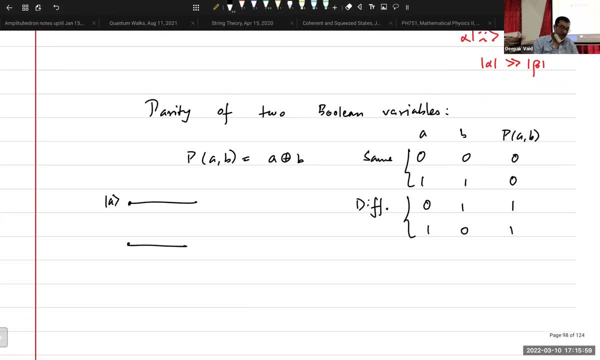 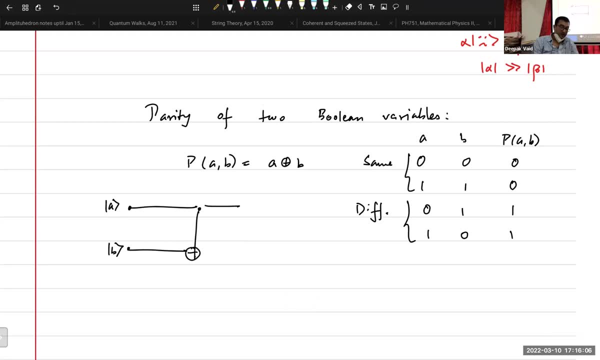 of a CNOT. If you have a state A and a state B, then what does this, what does this mean CNOT do? here? it gives you the output is the state A XOR B, right? So this is what. 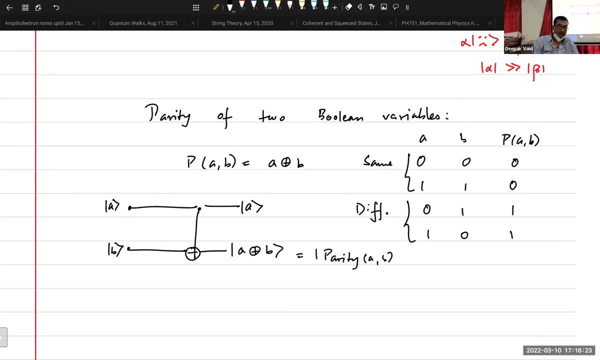 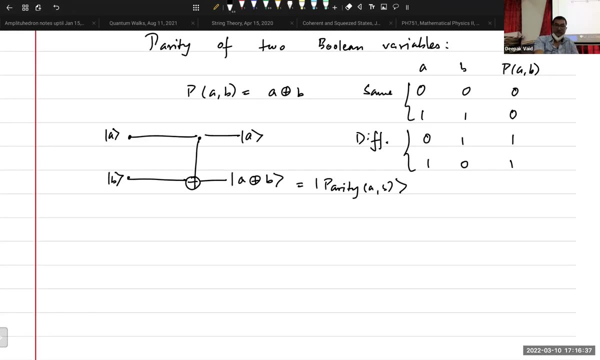 is this doing? This is giving you the parity of A- B, And you can measure this parity right, Or you can use it in the circuit to determine whether A and B are the same or they're different- right And depending on the, whatever the. 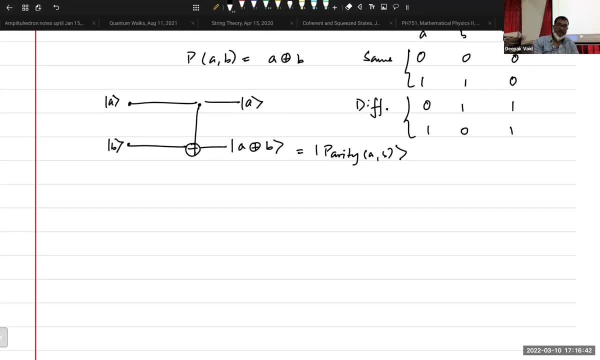 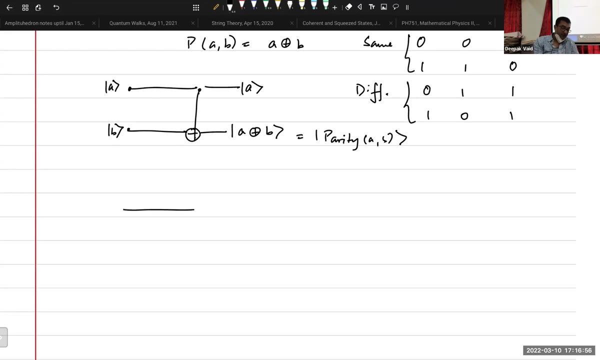 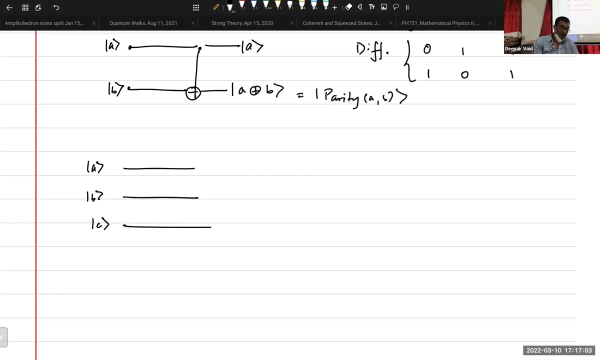 outcome is: you can perform your recovery. Now what we want to do is we want to do this for three qubits. So how do we? what is the circuit for doing that? So we need these are the three qubits. let's say ABC, And we want to do this parity check between qubits. 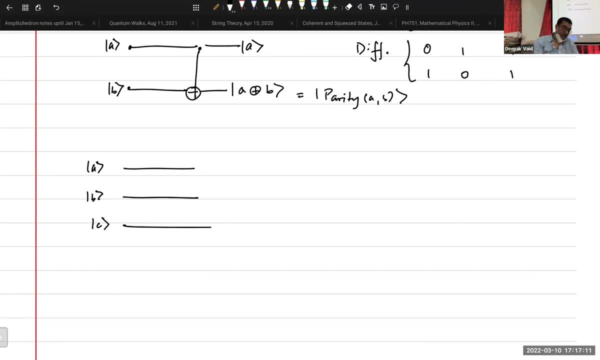 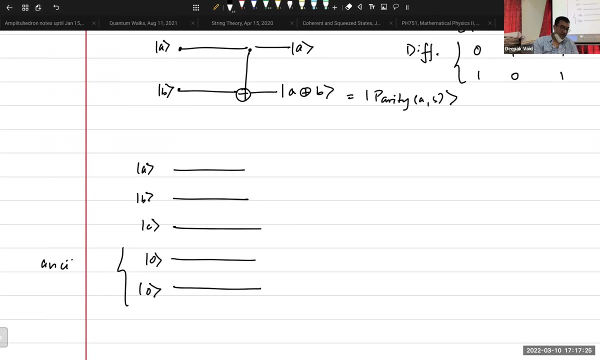 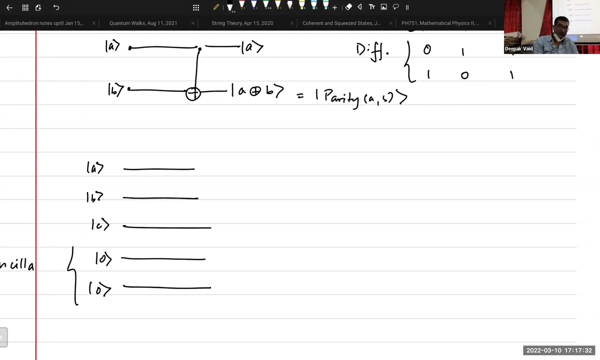 1 and 2 and between qubits 2 and 3.. So what we need first of all is we need ancilla qubits for this purpose. So these are ancilla qubits. So the first step is to perform a CNOT between: 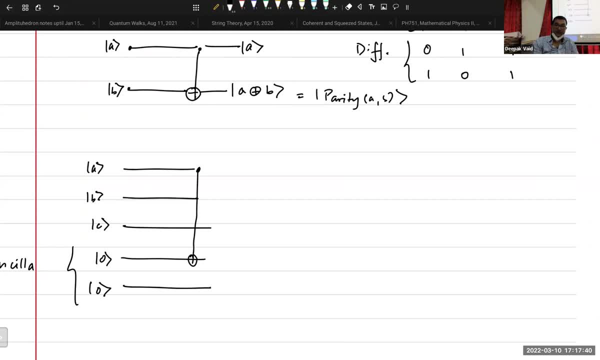 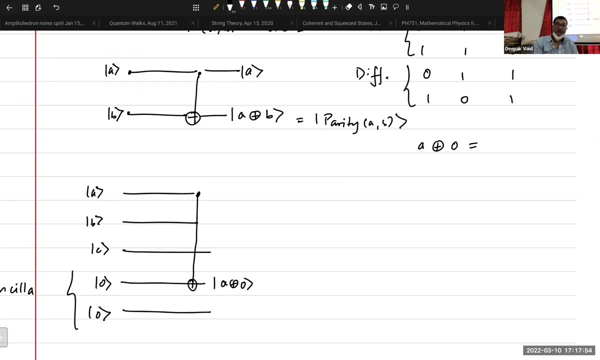 qubit A and QA And qubit this, qubit 0.. So here what you will get is A XOR 0.. Now for any Boolean variable, what is A XOR 0?? If A is equal to 0, you get 0.. If A is equal to 1,, you get 1.. So A XOR. 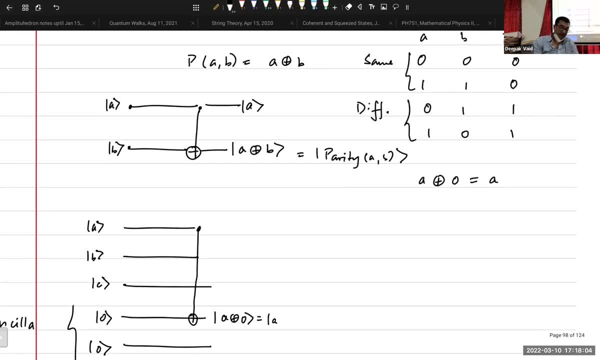 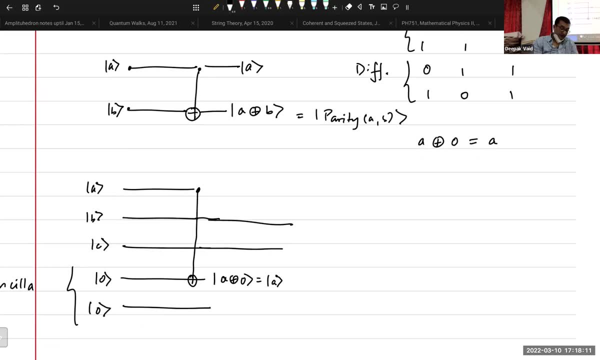 0 is A, So this just gives you the state A over here. Okay, Then you do an XOR between B and the this ANSYLAR qubit right. So after this first XOR operation, the first ANSYLAR qubit contains A right. So if you perform the second XOR, operation. now, between the second qubit and the ANSYLAR qubit, you get two XORs. Now these, any one of the two XORs will compare with another. per this answer as to what you're getting a little Right, Okay. So this is the root feature we are showing. 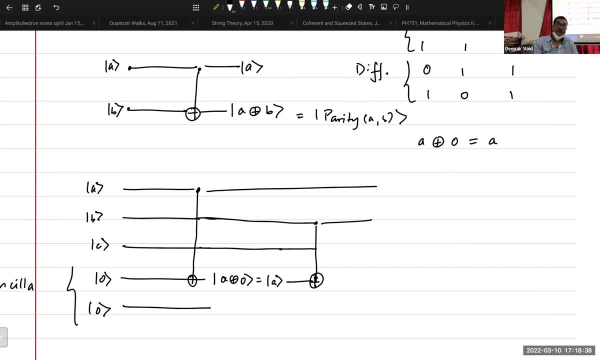 going inside. And now we need another answer as to what is actually going to be taking place. Am I properly going into this story? Am I frankly asking for help? in this 베igge rhyme and the first ancilla qubit, right, what will you get over here? you will get a xor b. 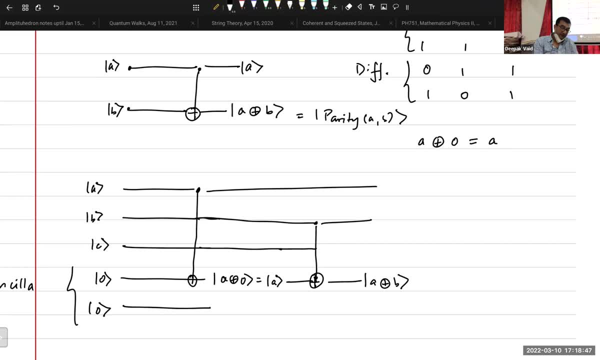 right, because that's what the c naught does. right c naught is taking this a and b and giving you a xor b. so this c naught is acting on this qubit and this qubit, these two qubits- right. so it will give you a xor b over here, zoom people. is this fine? are you able to follow? yes, sir. 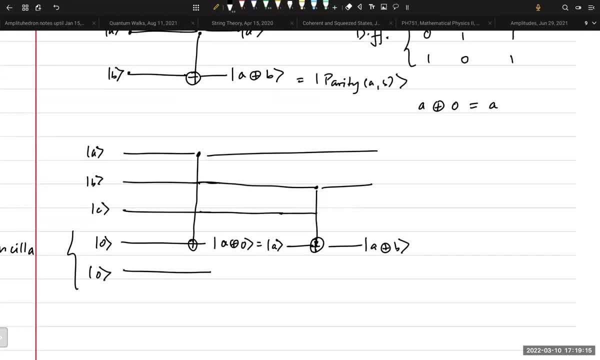 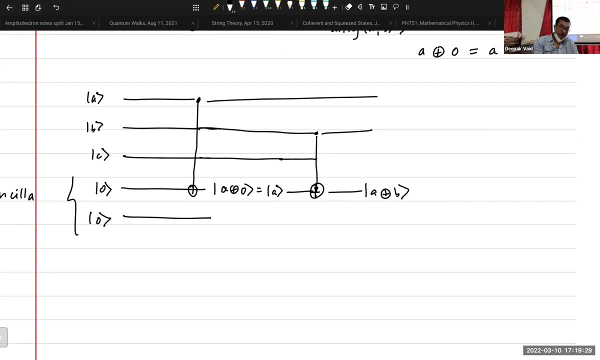 so now we can do exactly the same thing with the second and third qubit, right, and we will store that parity in the second ancilla, right? so what do we do now? we take the second qubit and we perform a c naught between the second qubit and the second ancilla. 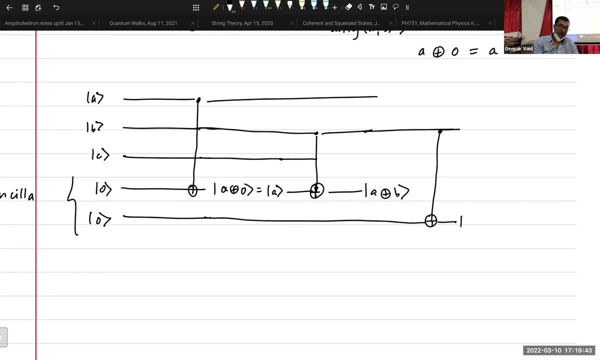 what do you end up with here? you end up with b xor 0, which is b right. then you take the third qubit right and you perform an xor with the third qubit and the second ancilla right. what do you get? you get b xor c. 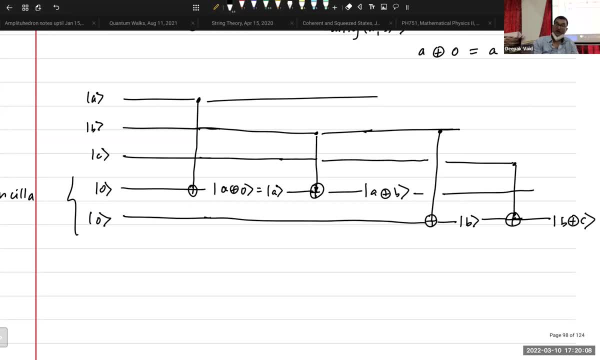 right. so the first ancilla: now it contains the state a- xor b. and what can you say about, about these qubits? well, the original data registers are unchanged, right? so you have stored the state a- xor b and you have stored the state a- xor b, right? so what do you do then? now, if we do not important data state a, really important. 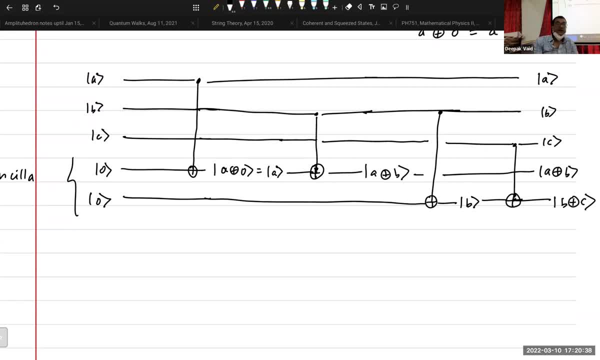 vais just that. so what'sconstortunately very women want to do is: is not the panda? we can get rid of the parody in these ancillary qubits. thank now, if the parity, so depending on the value of these two variables, that we can find the appropriate recovery. 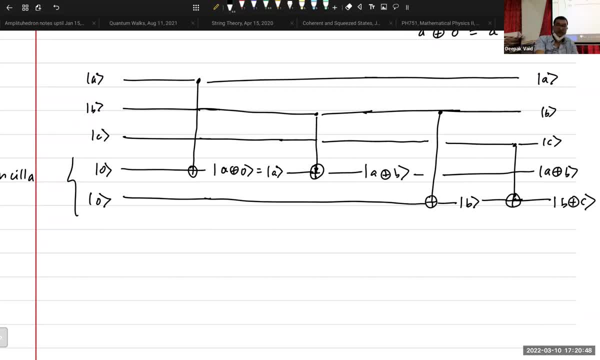 right. so, for instance, if a, if a xor b is Ben B from BC plated currency. now it was 1.3, yep sorry l that each of which plays to equal to 0, right? so if we get it again, this original data register remains the same. 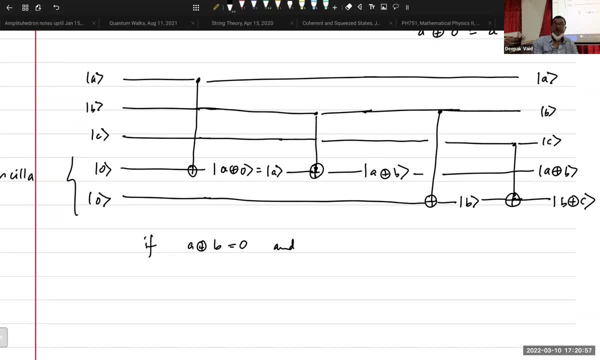 but now on every basic thing, in these ancillary q bits there is a, literally to create a product inside z飛s, compared to calling it alpha touse e, we can apply the appropriate recovery right. so if a gets or B is equal to 0, then 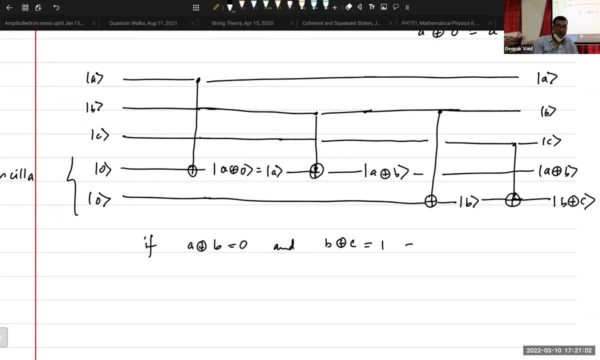 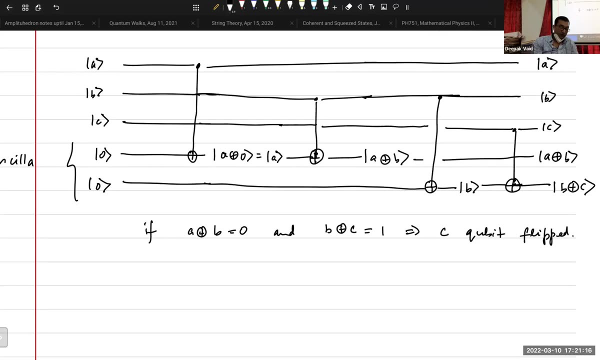 retracted. so if X xor c equals to the other N xphlish號, you can. and B XOR C is equal to one, which means that B and C are different. So this means the C qubit has flipped right. And so then, what would we do? We would apply what would be. 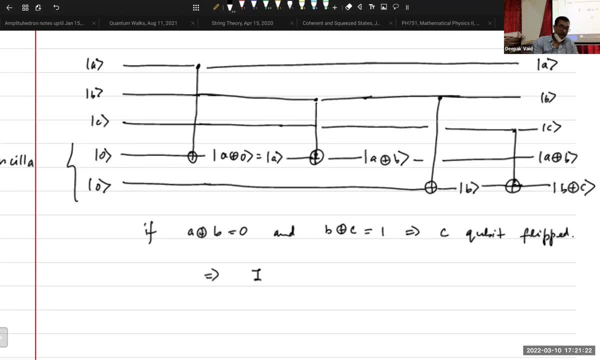 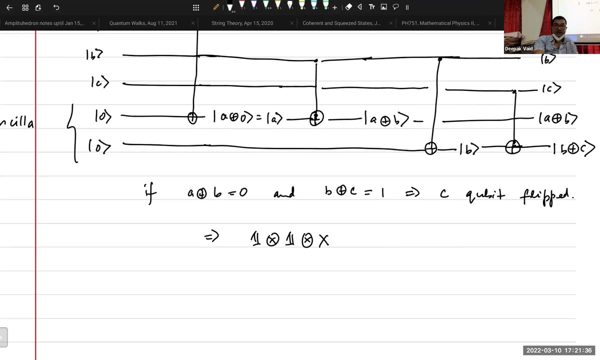 the correction, How we correct it. We would apply this gate identity identity X right, Because X gate would flip the third qubit back to its original state right. So you would need to get the complete information. you would need one more set of parity checks. 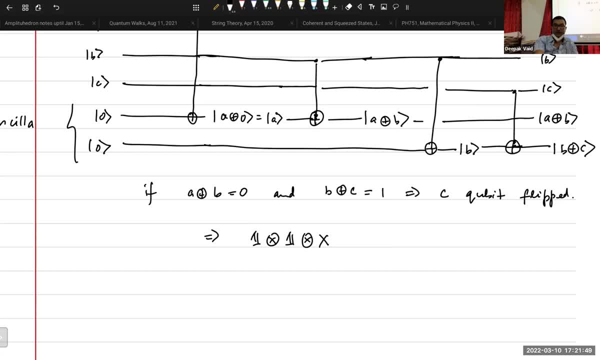 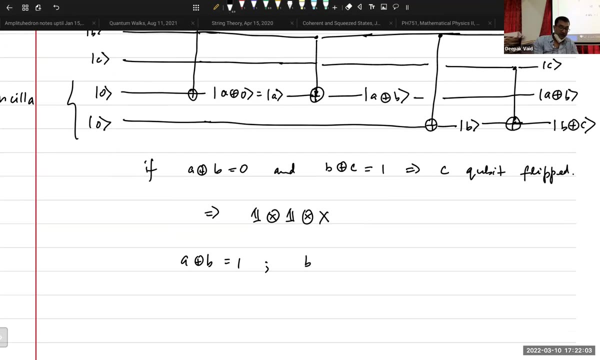 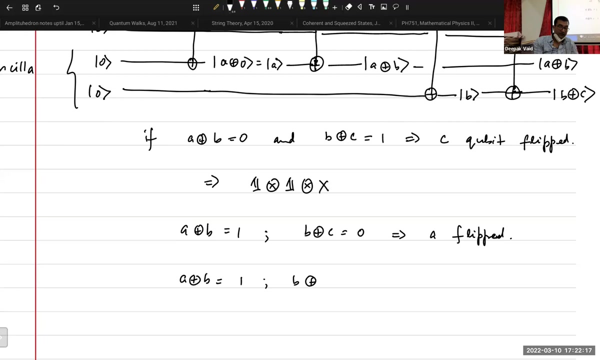 Well, no, I think this is enough, because right. So these are the three possibilities. If A XOR B is one and B XOR C is zero, this means that A has flipped Okay Again, assuming that you only have one single qubit errors. and if both A and B, A XOR B and B XOR C are. 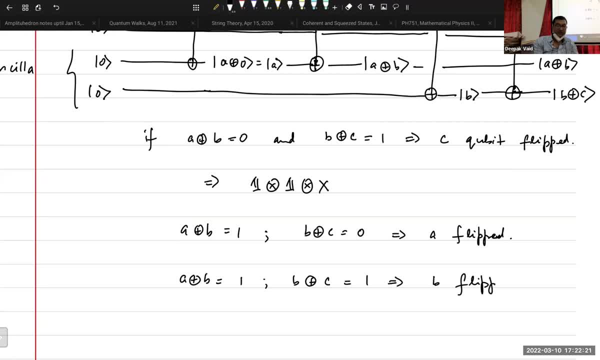 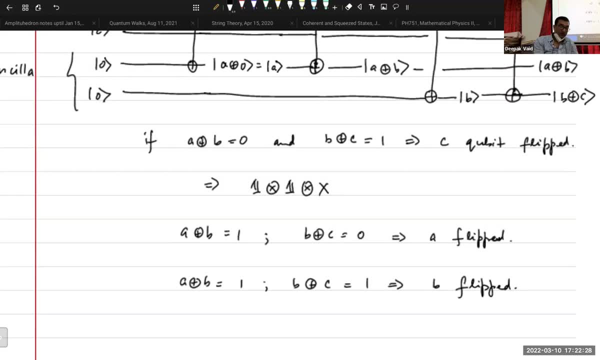 one. this means that B has flipped. So these two parities checks are sufficient to give you information about all three qubits. I hope that that was helpful, Thank you. I hope that you can convince yourself that this is indeed the case, right? So this would. 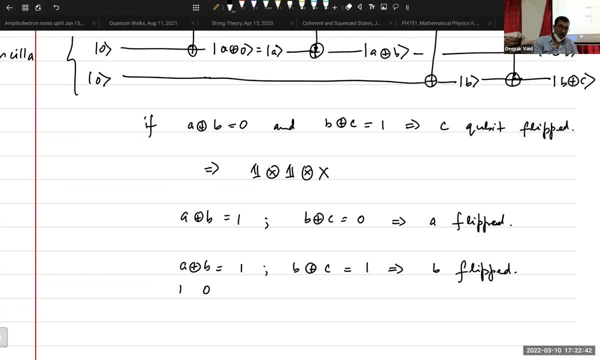 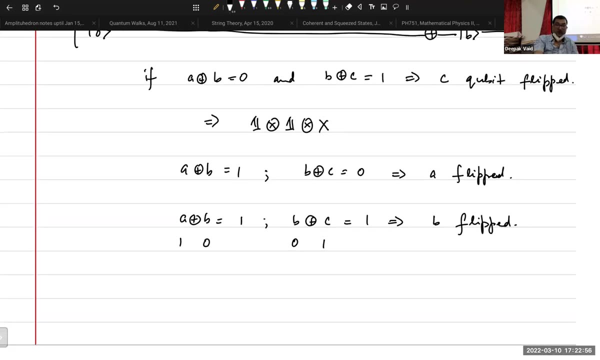 mean that let's say A is one and B is zero, but then B is one and C is zero, right? So now, assuming again, single qubit errors, this means that it is B which was flipped, Okay, Right. So what we want to do is, depending on the value of the parities, we want to apply the 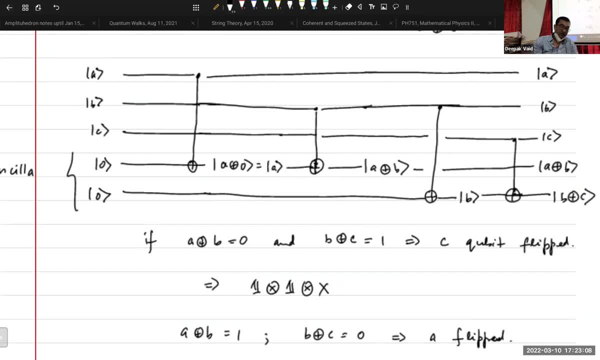 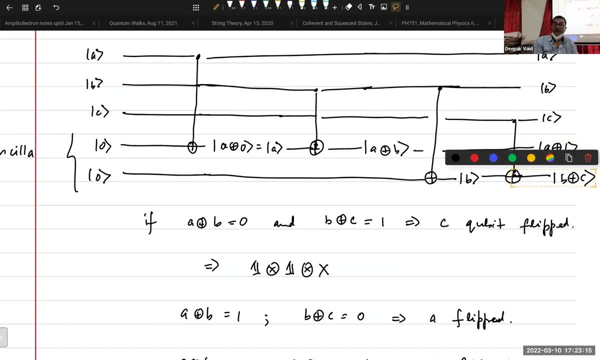 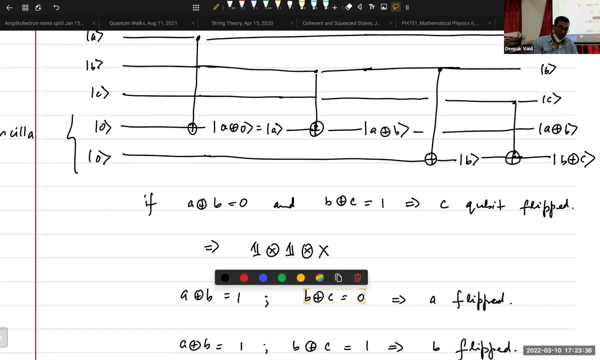 recovery procedure: right. So the recovery procedure is conditioned on the values of these parity, on these parity qubits, right? So now, if A, let's say B XOR C is zero, right Okay, And A XOR B is one, Then so B XOR C is zero and A XOR B is one, That means A has flipped. 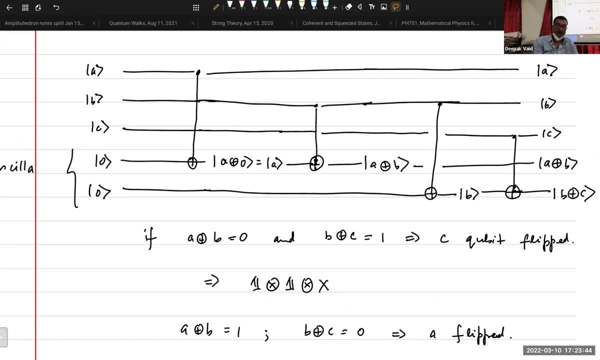 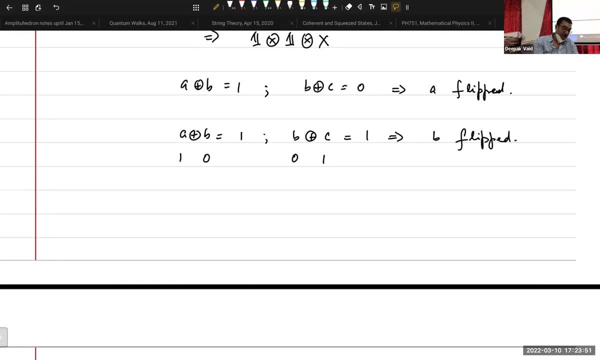 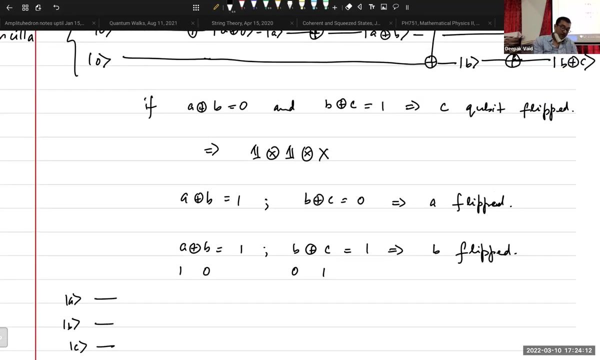 So we want to apply the X operation on A right. So now I'll begin the circuit. I'll continue this circuit. I'll begin the circuit from this point onwards that I have these, where I have stored the… the parity information in the ancilla qubits. So if A XOR B is 0 and B XOR C is 1, then 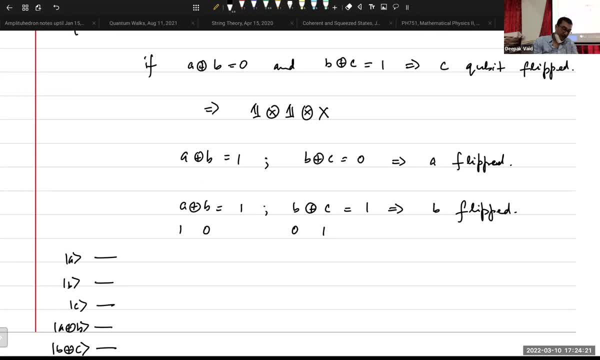 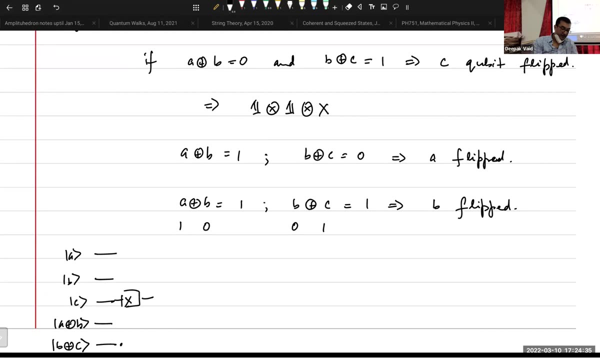 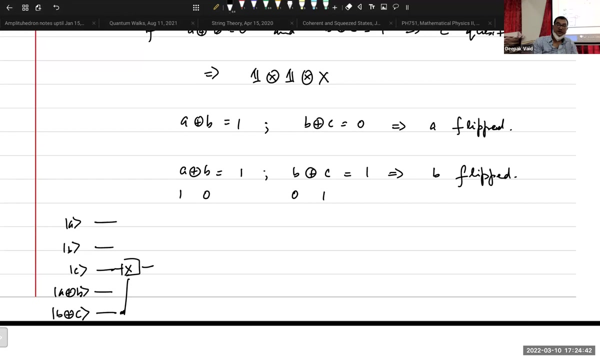 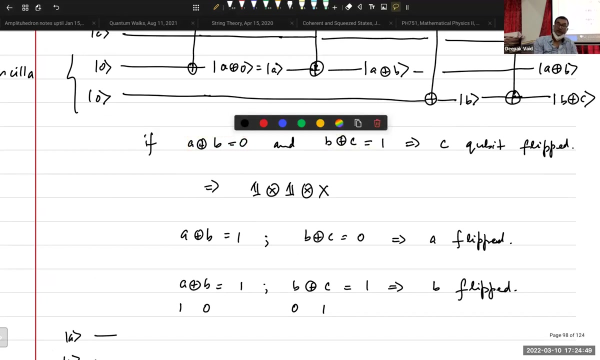 I want to apply this X operation on the third qubit. How can I do this? This is a controlled operation, So I use B XOR C as a control and I put an X over here like this: Well, I am talking about the first case: A XOR B is 0,. B XOR C is 1.. The second case: 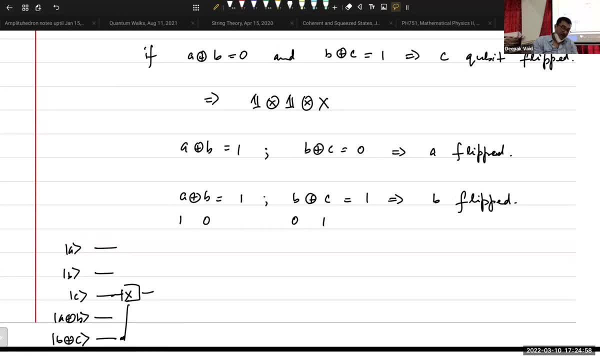 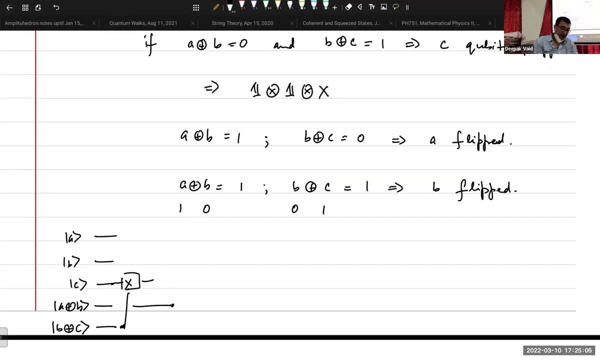 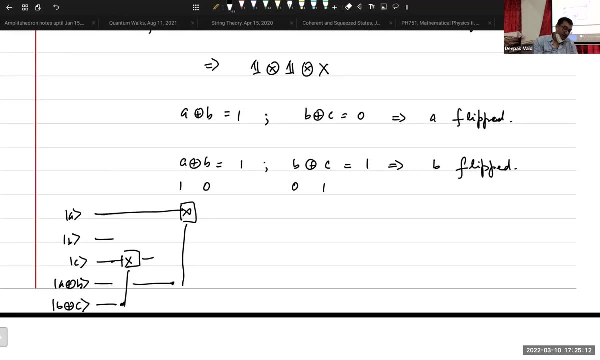 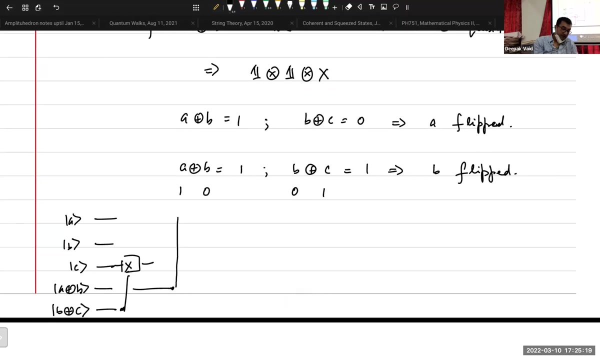 is that A XOR B is 1, B XOR C is 0. So A is flipped. So how do you implement that? You put a control X operation on the A qubit. Let me try to make that a little bit neater. 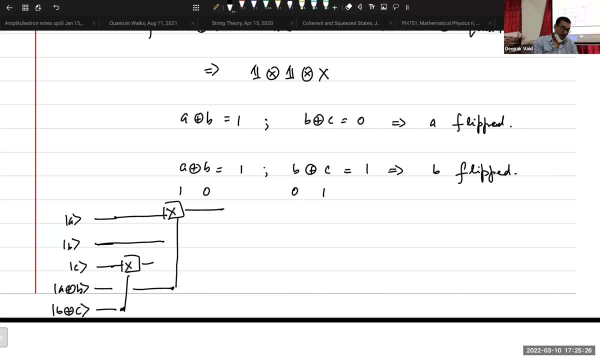 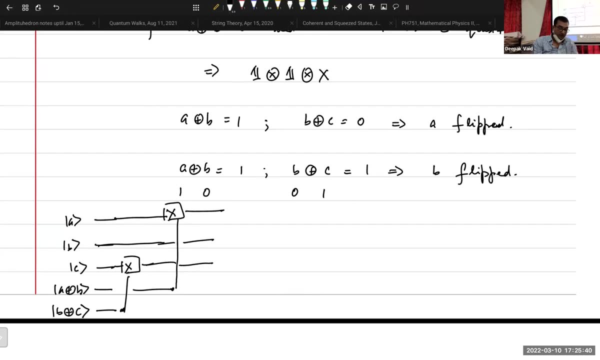 Okay, And what about the B one? The B one is dependent on both the parities. So both the parities parity qubits will control this X operation on the B. So you remember there was a CC, not gate. It is the same thing. You have two controls now and you have an X operation. 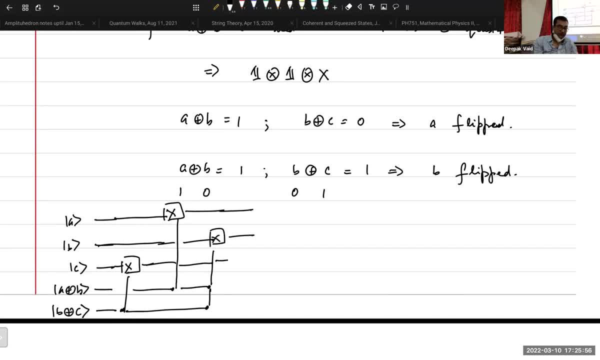 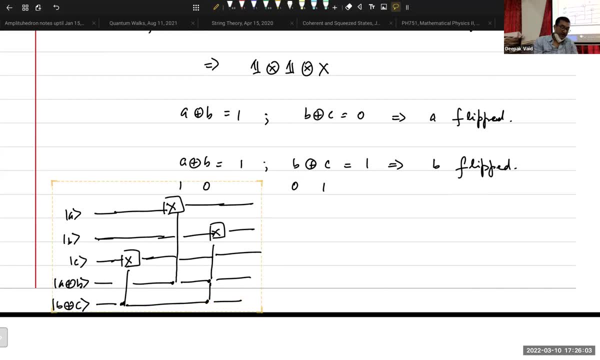 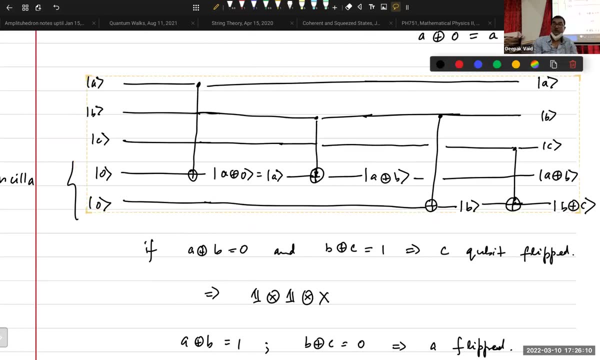 Okay, an X operation here. So this is this circuit, this is your recovery procedure, this is your syndrome, your syndrome measurement or syndrome detection. sorry, No, no, no, no, no, no. Just look at these conditions again. 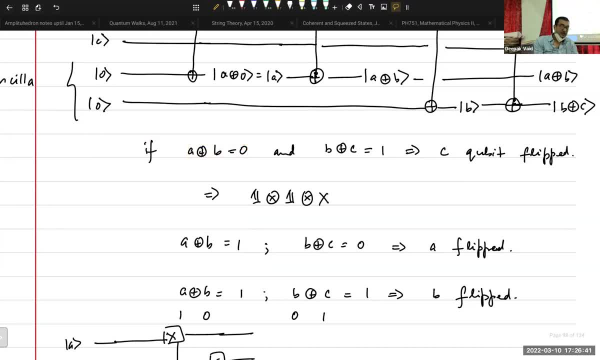 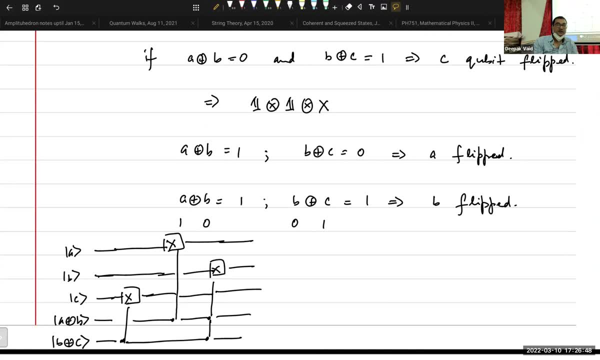 Right, This is the first condition. C, C qubit is flipped. So I don't understand. So this covers all three cases. which one? No, no, no, no, no, We are assuming single qubit errors, So only one qubit at. No, no, no, no. We are assuming single qubit errors. So only one qubit at No, no, no, no, We are assuming single qubit errors. So only one qubit at most can be flipped. Yeah, somebody else can explain what these kinds of things are. 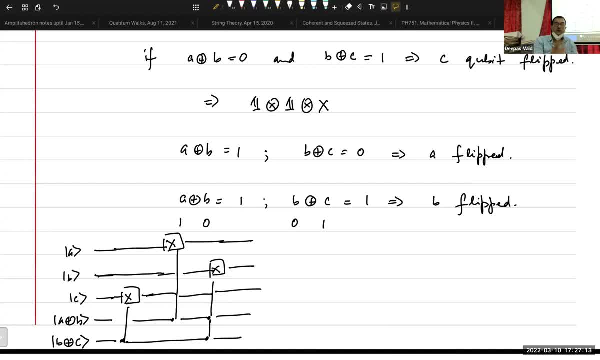 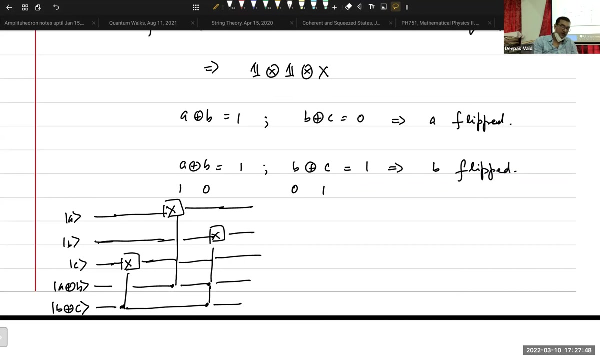 Yeah, somebody else can explain what these kinds of things are. 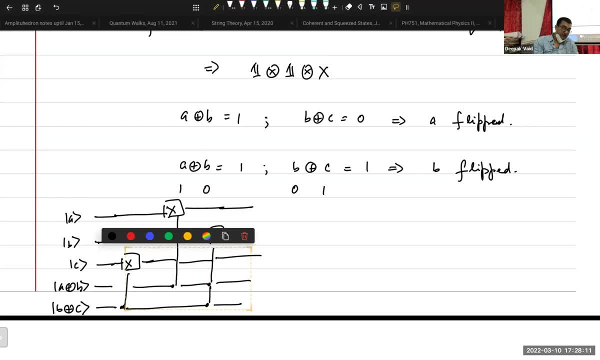 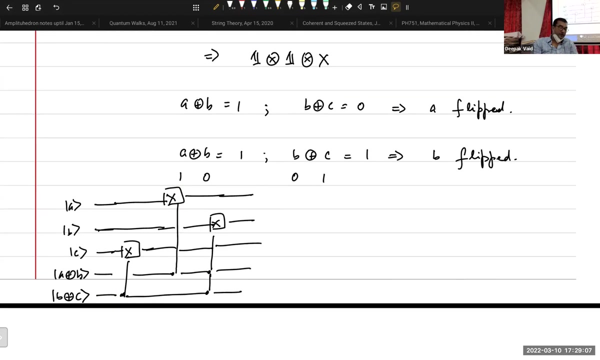 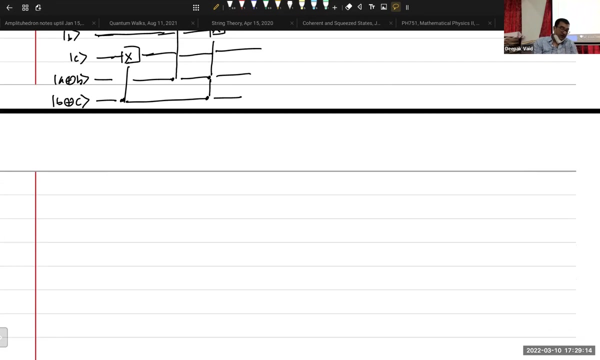 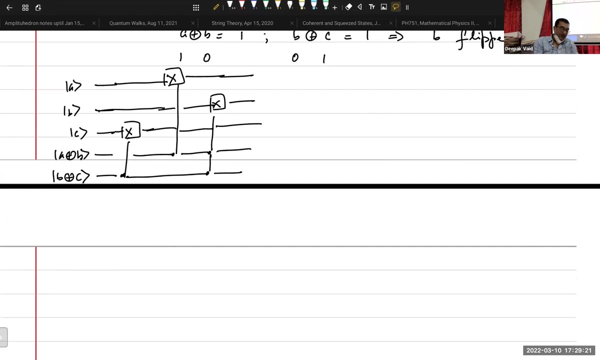 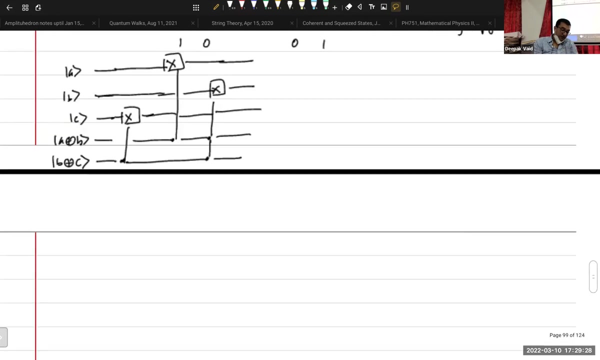 the resolution is as follows. So there's a good point. The resolution is that here I just said that you apply the control x, But in fact what you're supposed to do is you're supposed to put a measurement. 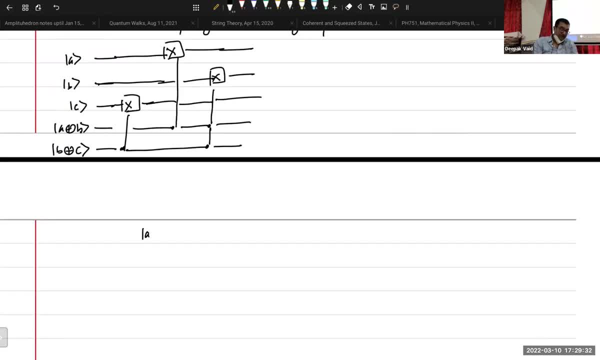 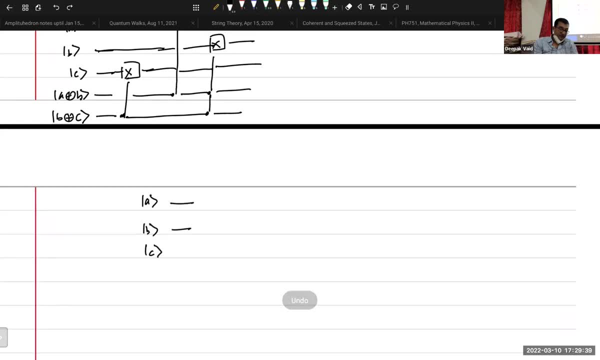 You're supposed to measure these, these, Okay, so let me write down the circuit with measurement: measurement- okay. so at this point what happens is that one performs a measurement on both of these parents, okay, and then you perform a controlled. so once you measure, it becomes: 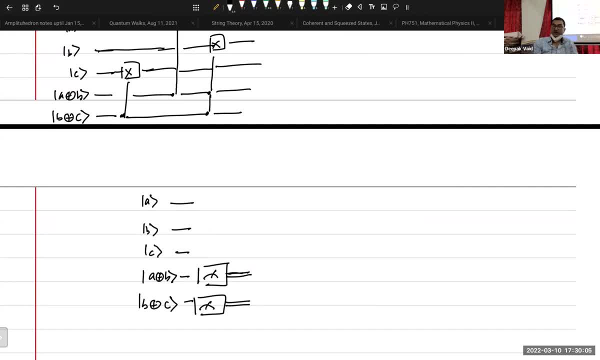 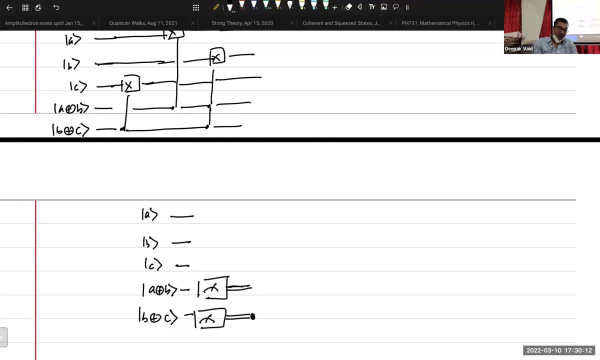 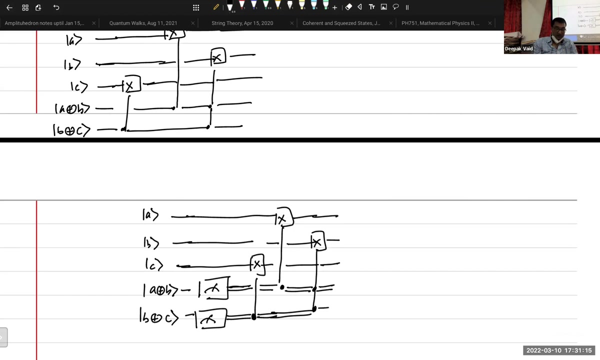 a classical bit. and when it's a classical bit, you would have draw it with two lines. and now, if we, now we put the control, this thing, x operation, right, okay, this is x, and then uh, x, which one second. yeah, you're right. okay, this is so that. 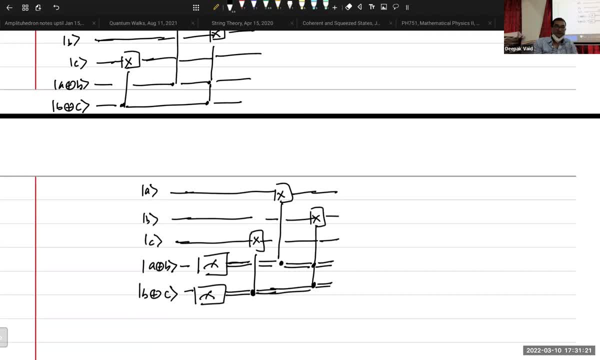 even if it takes a little time, you need to. you need to for the development of the you know uh, of this. um, no, it turns out that you don't need that. this is sufficient and i we can, so i'll do something. I will show the circuit in Quark. Fine, We will look at the circuit in Quark and then. 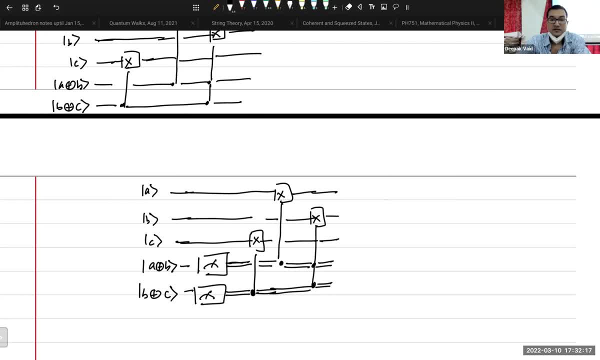 you will see One second. Let me do one thing at a time, But this is not a circuit. Guys, can you please hold off on that debate One second. Okay, I need to stop this sharing Right? Okay, Got it. 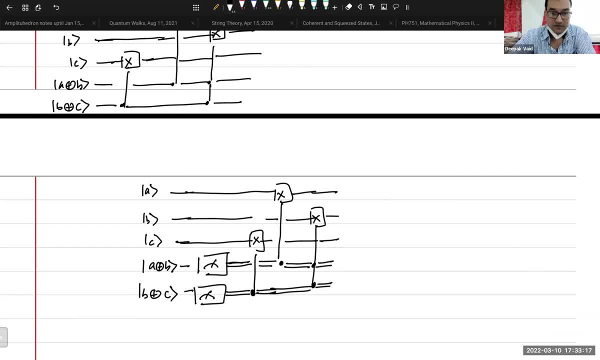 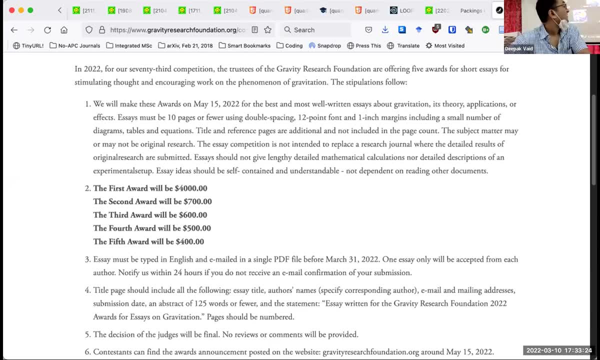 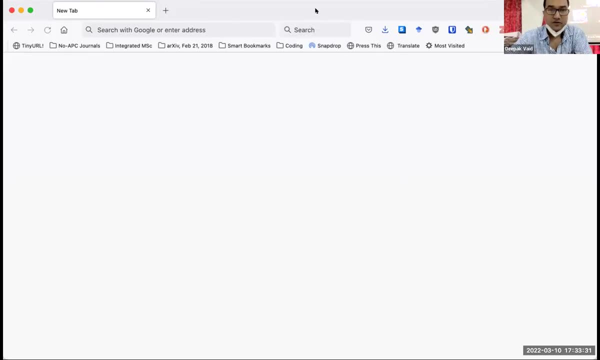 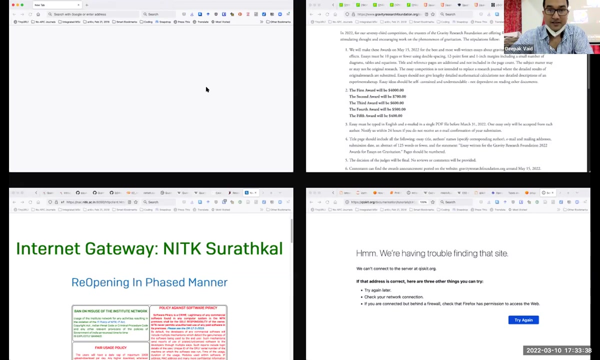 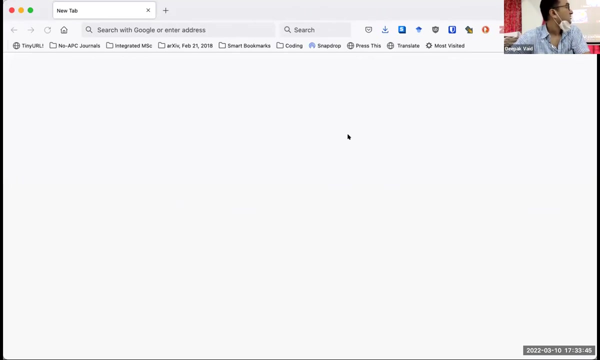 Share screen. Is it not showing One second? Yeah, yeah, yeah, I know this. I changed it, but it's not. Oh, in this desktop thing, I'm still trying to figure out One second, Stop share. 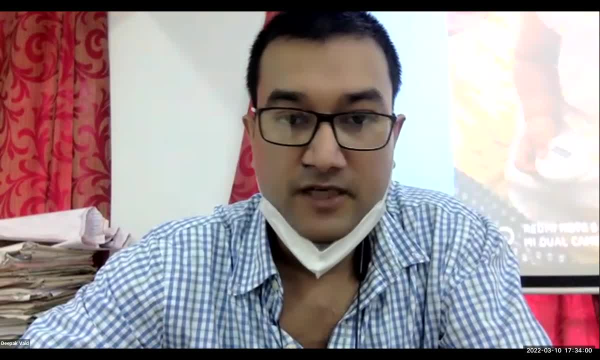 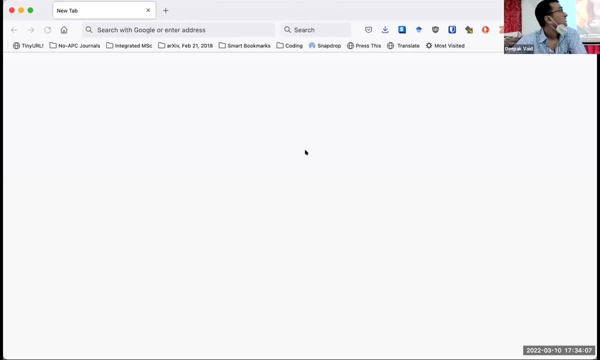 Yeah, this Zoom is One has to. Okay, no, Why is it not showing now? Can you guys see it on Zoom? Okay, Okay, Then just look at it on Zoom. Fine, So let's go to notquickercom Quark. 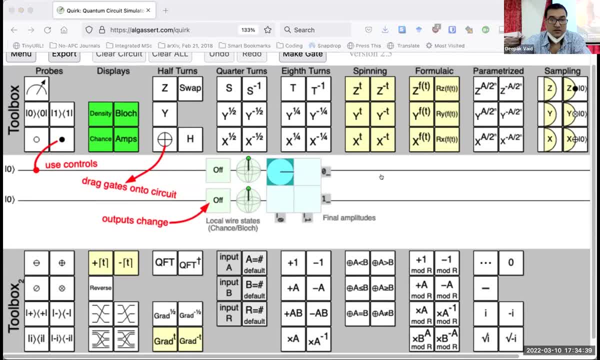 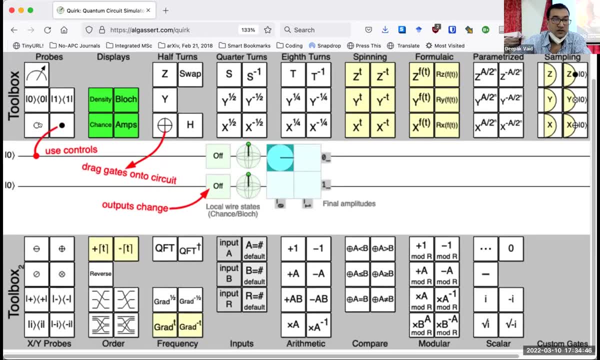 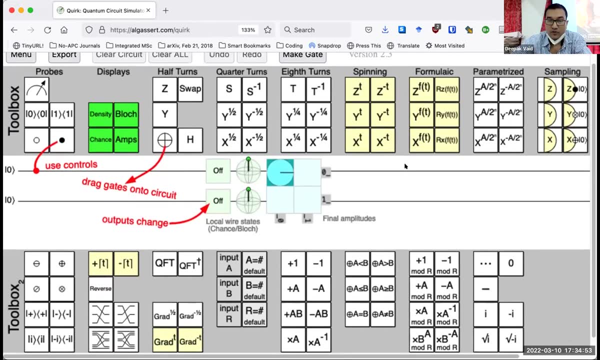 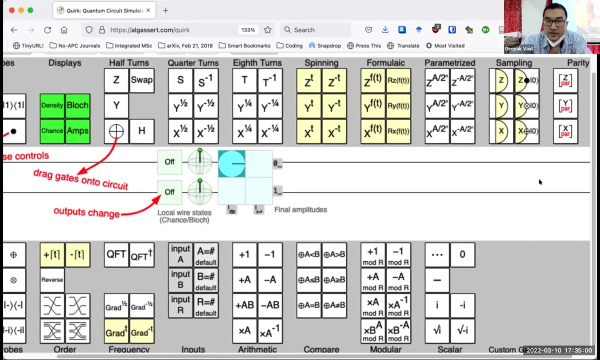 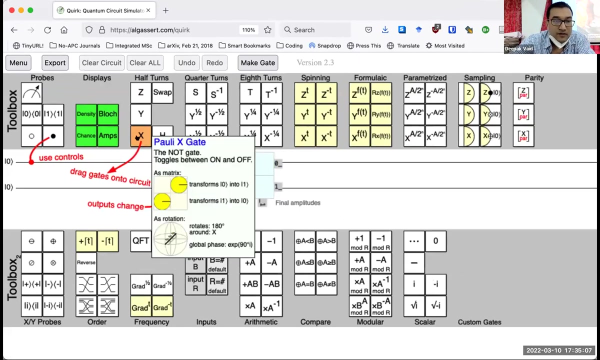 Okay, Okay. So what we want is the following: You can see the Quark one, I hope, Okay. So first of all, let me put these block spheres. Where is the block sphere? Okay, Block sphere, Block sphere. 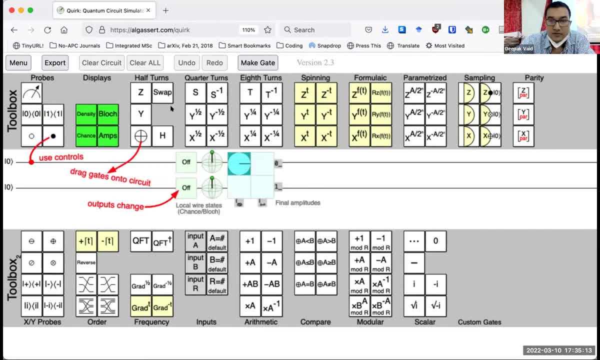 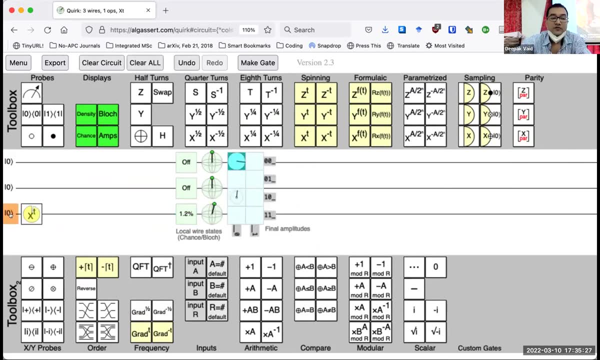 Tool: measurement block sphere. i'll come to in one second. okay, first let me take, uh, this: this is my error. okay, so i start off in 0, 1, 1, and now i put a time dependent error. this will allow you to see that the error is actually being corrected in real time, okay. 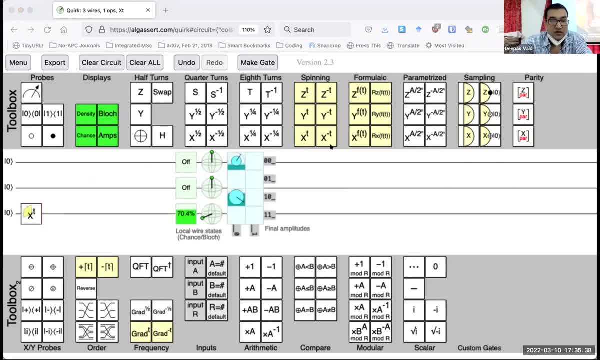 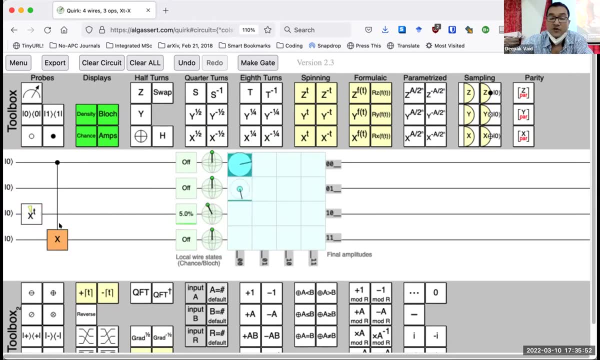 and now, uh, we have two more, uh, two ancilla qubits, right? so we take, uh, this and we have a c naught between the first qubit and our ancilla qubit, which is the fourth line here, right? so then we have a c naught over here, and 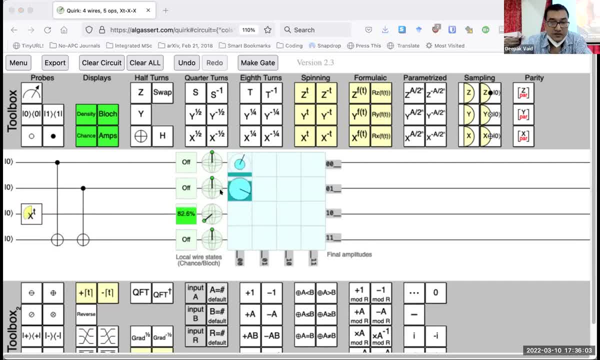 uh, so c naught, right. so we have a c naught over here and we have a c naught over here, and we have a c naught between a and b and the. uh, first ancilla. qubit ancilla is on bottom. okay, then we want to do the same thing with b and c. 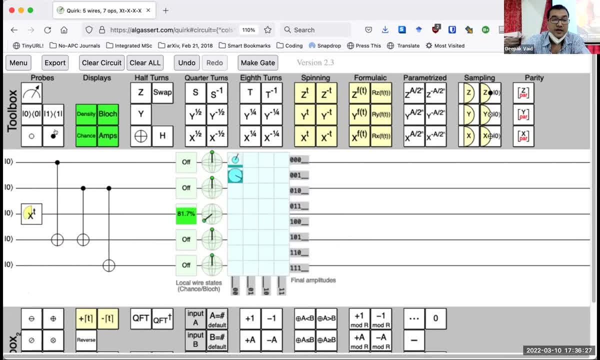 right, and we want to put that information in the second ancilla bit, which is the the last line right. this is the fifth qubit right. this is the fifth qubit right. this is the fifth qubit right. so now, so now, so now, uh uh uh. the ancilla contains the parity. 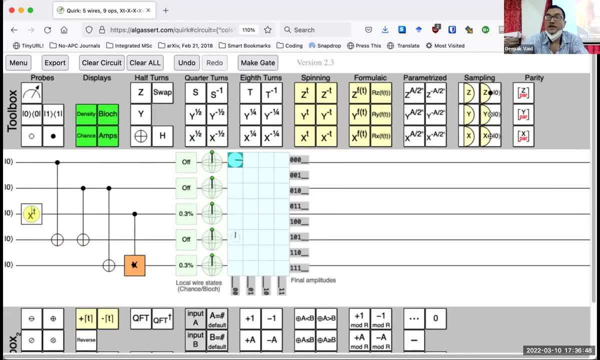 the ancilla contains the parity. the ancilla contains the parity of a and b, of a and b, of a and b. ancilla one and still two. contains the ancilla one and still two. contains the ancilla one and still two. contains the parity of parity of. 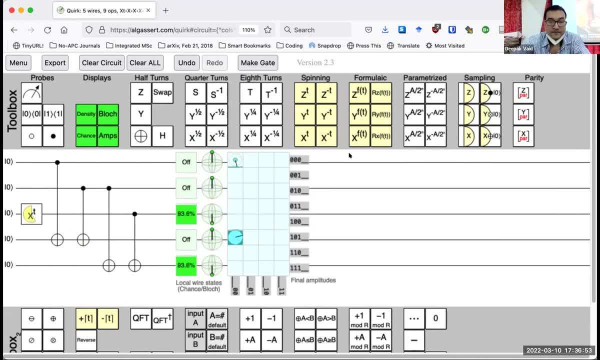 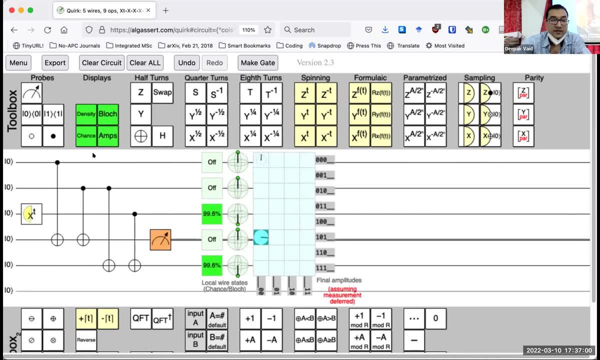 parity of uh uh, uh, b and c, b and c, b and c. okay, and now, and now, and now, we, we put a measurement, we, we put a measurement, we, we put a measurement on the ancilla bits, on the ancilla bits, on the ancilla bits. okay, 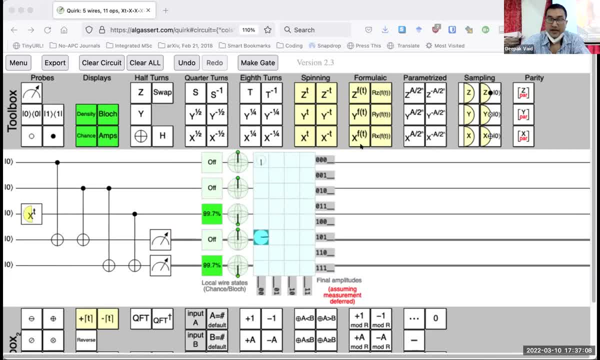 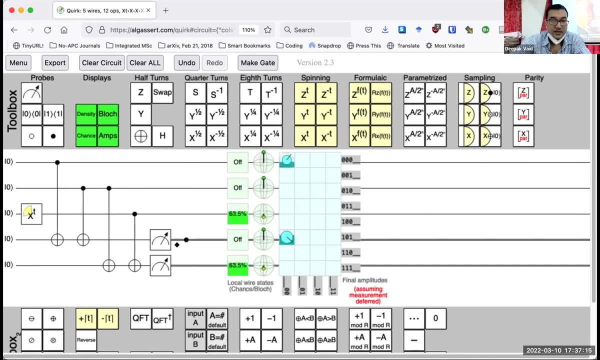 okay, okay, and now we perform the and now we perform the and now we perform the error correction, the conditional error error correction, the conditional error error correction, the conditional error correction, correction correction. so the conditional error correction, so the conditional error correction, so the conditional error correction is. 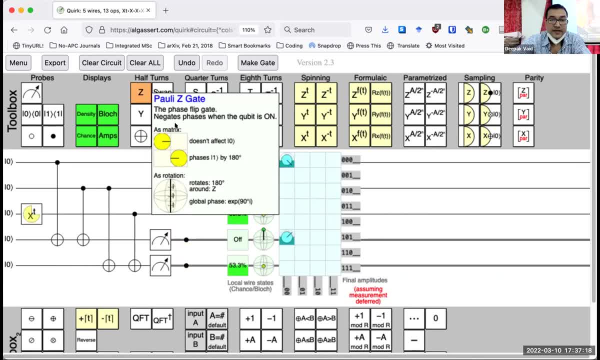 is is as follows. as follows, as follows: uh, where is x? x? is just this right? this is the one when both the parities, this is the one when both the parities, this is the one when both the parities are one right, are one right, are one right, uh then. 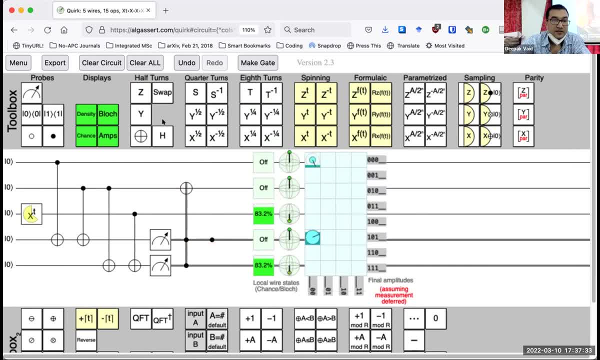 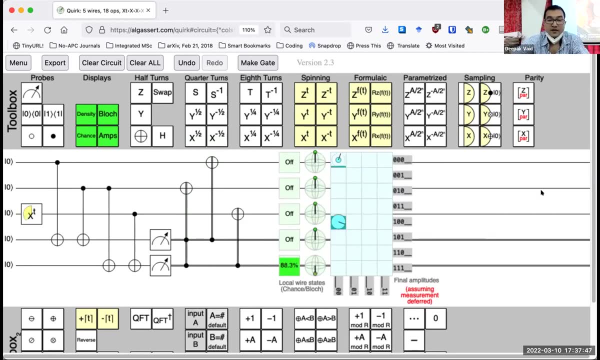 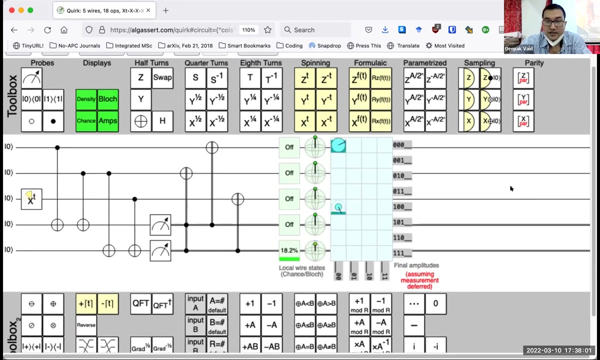 uh, then, uh, then, when, when, when the second parity is the second parity is the second parity is uh, uh, one, we flip a. and when the third parity is second parity is one, we flip c. okay, now, this should give you the same state. uh, after doing this, you should get a, b, c right now. you see one thing: this is zero, zero, zero. 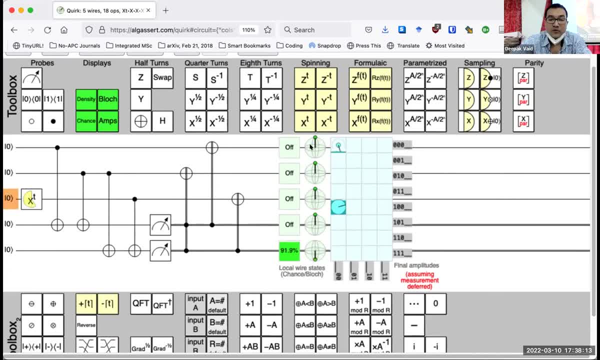 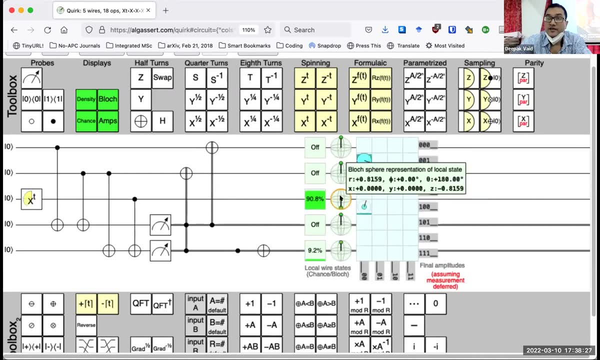 right, the input state is zero, zero, zero. what is the output state we are getting here? zero, zero, zero. right, let me remove one of these. let's say: right now, the output state is not the same, right? okay, let me remove this guy. let's say: this doesn't affect anything, uh, 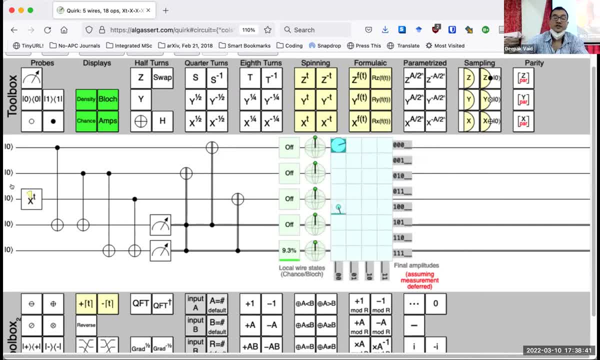 well, these two, removing these two will not affect anything, because so let me put another error on the y right, so that way it will become one. let me put y of t over here, and this will not do anything. z of t will not be an error. remember that z of t will just. 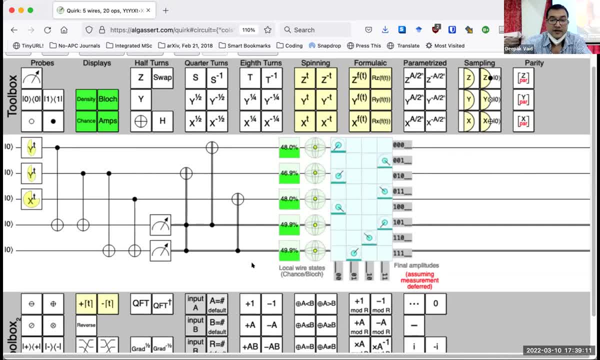 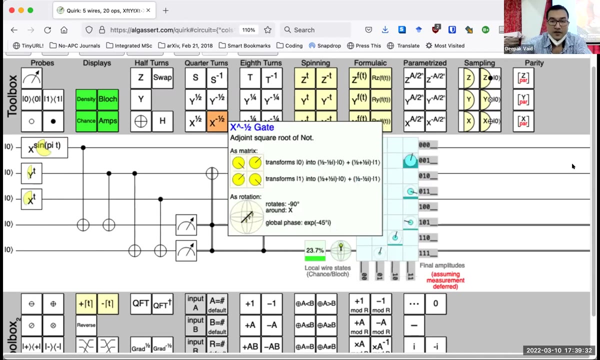 give me a phase. right now, you see, i have, and in fact you know i can change it to something else so that it doesn't. no, not okay. yeah, this is fine. so one, two, three, okay, is it? it doesn't work, thanks, thanks, thanks, thanks for pointing that. so, yeah, let's do it one at a time. 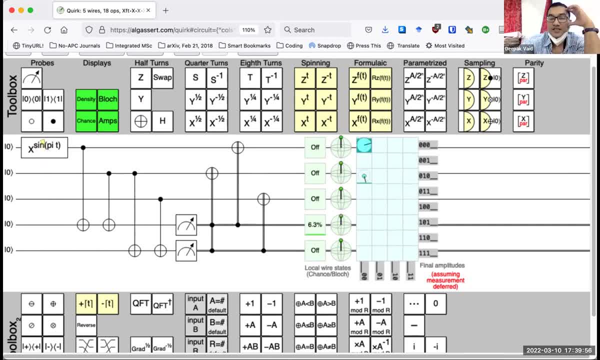 right, it's working for us, okay. So, working on this error, it works here, It works with this guy, But now it doesn't work. I think that, yeah, So let me just put another. yeah, okay, So I think you have a point there. Utsav, thank you for pointing this out. working on 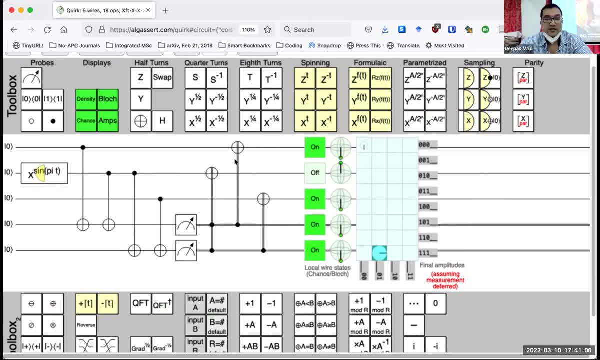 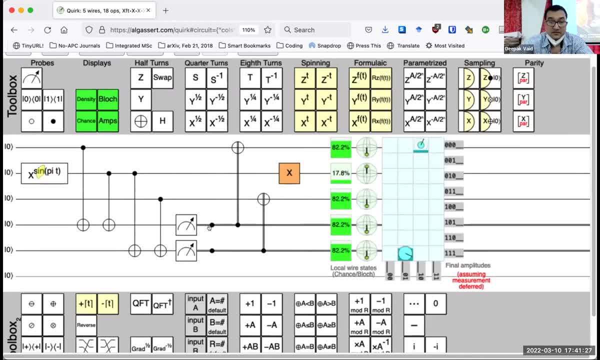 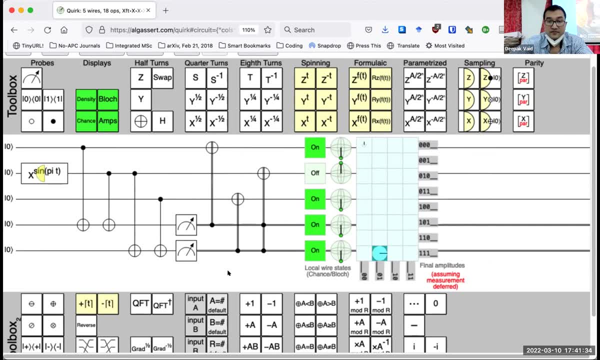 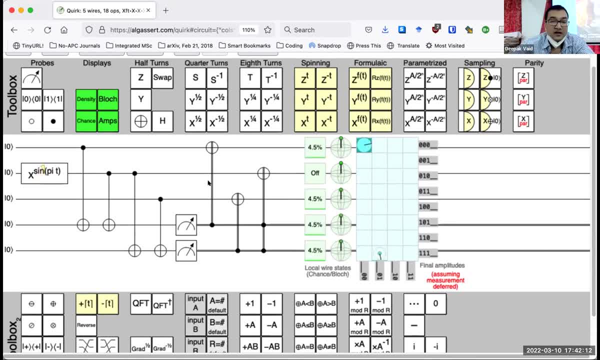 So you are saying you put an A here, X here and an X here. right, This is what you are saying. right, That's right, Brilliant, That's actually quite brilliant. I didn't think of it. I don't know if anybody 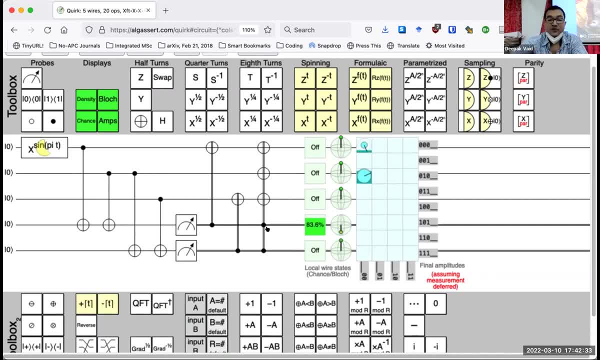 else thought of it. But he's right. If you put a double controlled xxx gate here, then all three of the qubits are correct. As you can see, all three of the qubits are correct And you have found an error in a textbook also in this process. So I will email the. 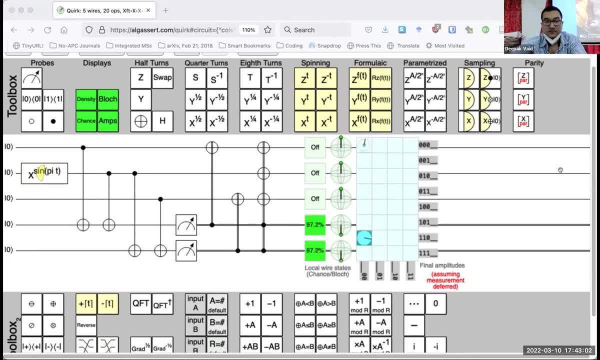 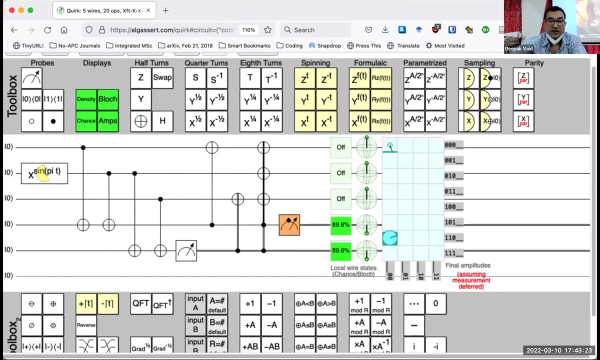 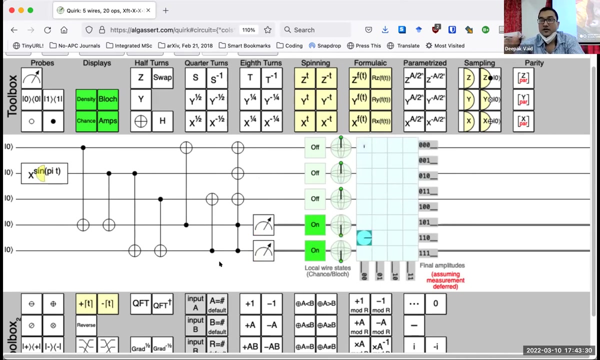 author and cc that to him. So anyways, this is an example of correcting a single bit-flip error. Now here's something very interesting. I have placed these measurement operators here. Now I'm going to do something funny. I am going to put my recovery sub circuit before the measurement. Is it still working? 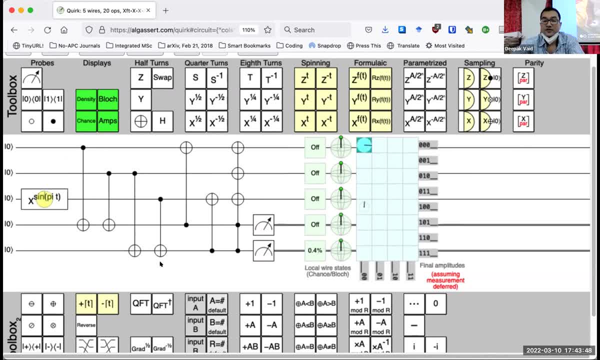 It is still doing exactly what I expected to do. This is a very important principle. This is called the principle of deferred measurement, So one way of stating it is that measurements can always be moved from an intermediate stage of a quantum system to the end of a circuit. So in this example, we had an intermediate stage where we put 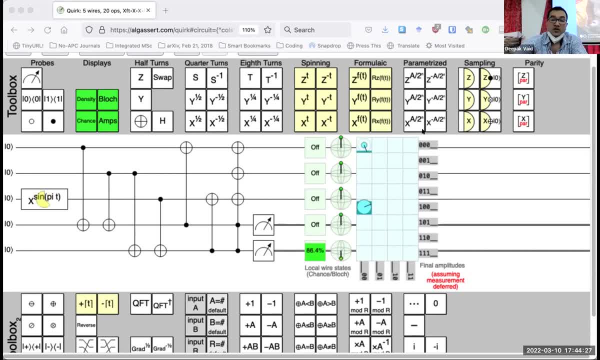 a measurement and then we put some control bits, I can always take that measurement and move it to the end, past the rest of the circuit. So in other words, I can take my classically controlled operations and replace them with the quantum version. So now you see this. 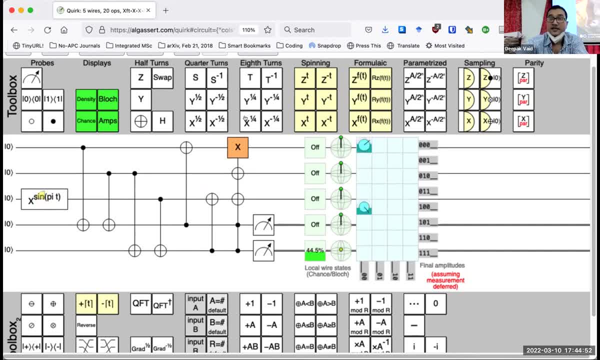 is a CNOT gate. this is a CNOT gate. this is a CCXXX gate, not a classically controlled gate. These are quantum gates, So this idea might take a little bit getting used to, but this is a very powerful idea, as you can imagine, Because in all sorts of algorithms this is 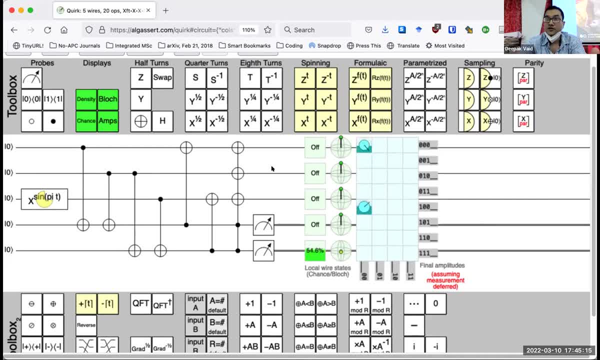 just an example. This is a building block for measuring parity, But you can imagine that if you have a bigger circuit, like a 9-qubit circuit or something like that, you will have lots of measurements because you have 9 qubits if you want to construct. 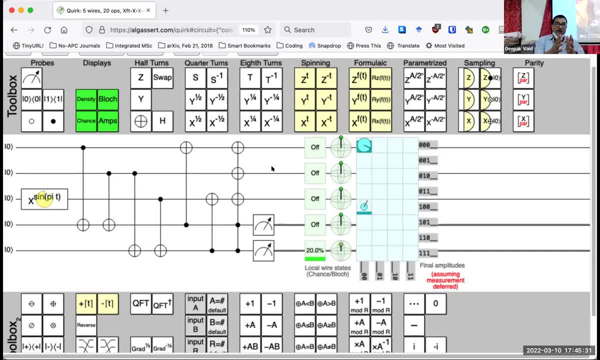 a circuit like this, So one can take all of those measurements and put them at the end. So first you construct your circuit with the measurement and then the classically controlled gates. Once you are happy that it works, you just take the measurement and 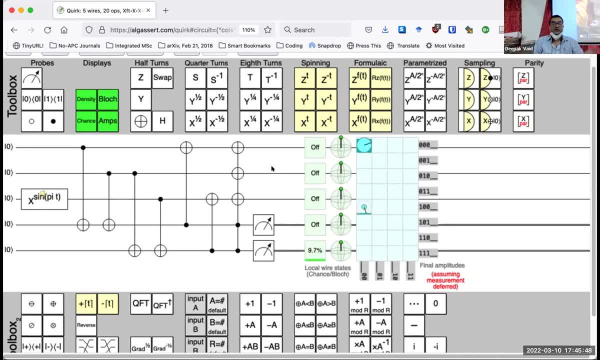 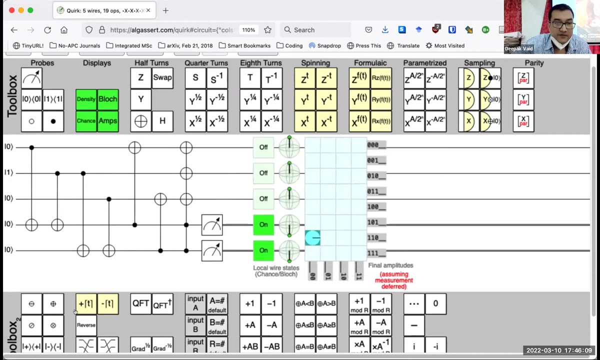 put them at the end. It's weird, I know it's weird, but it works, as you can see. But now is it working for arbitrary this thing? One second, Let's see if it works for arbitrary values of these bits. So it will only work if your input state is 0, 0, 0, or. 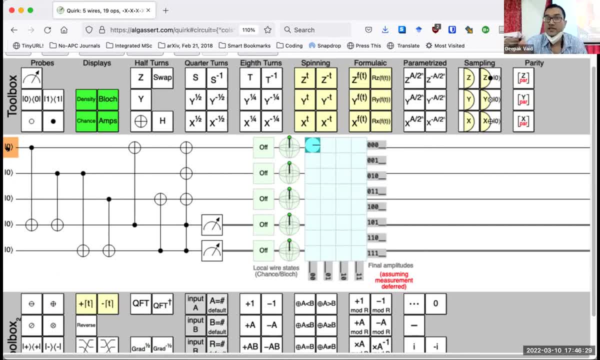 1, 1, 1.. Because if you put in a state that is 0, 1, 0,, which I had just now, that state already has an error. So if I put 1, 1,, 1, 1,, then it will only work if your input state. 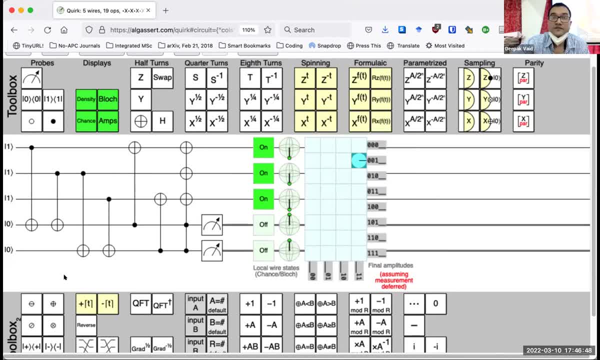 is 1, 1, 1, 1, right, Then I see I get 1, 1, 1.. Oh, no, no, no, the error correction part. right, right, right. So sorry To see the error correction part you have to change. 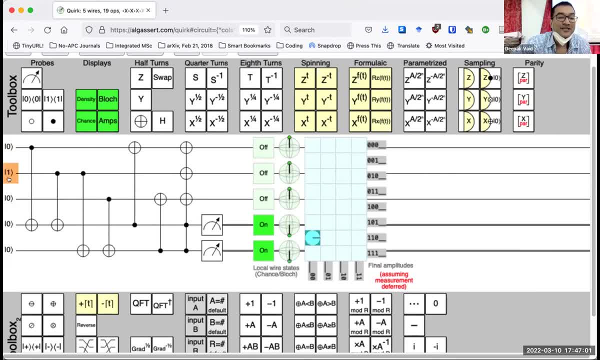 one of these bits, my mistake, So let me put in 0, 1, 0.. 0, 1, 0 should be corrected to what 0, 0, 0.. 1, 1, 0 should be corrected to what 1, 1, 1.. 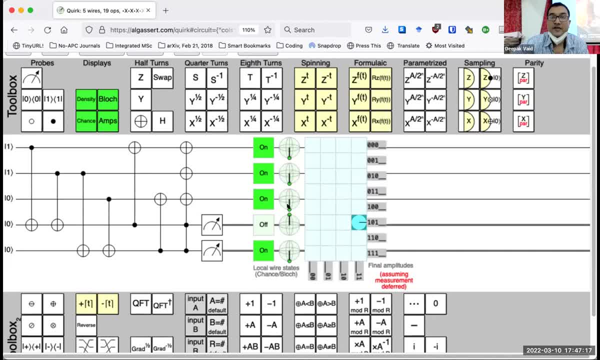 Right, Right, Right Right. We are getting 1, 1, 1 here, right? Yes or no? Yes? And then, of course, if this is 1, 1, 1, there is no error. Then we can try making this: 0, 1, 1, 0,. it is being corrected. 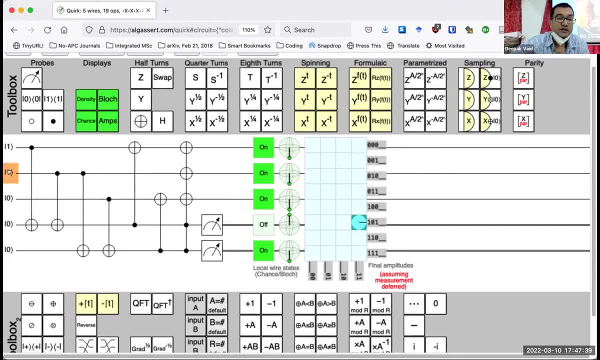 to 1, 1, 1.. What if we make this 1, 0, 0,? it is being corrected to 0, 0, 0. Right, So this is our state, which has a single bit flip right The first four gates. 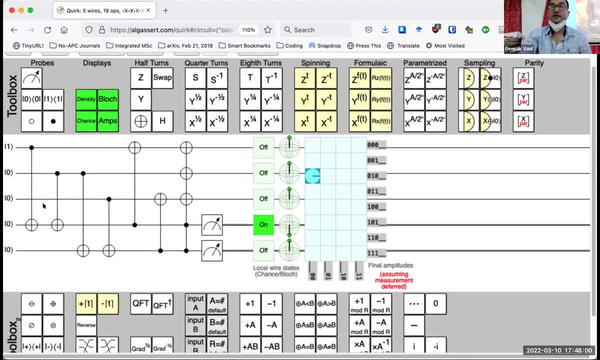 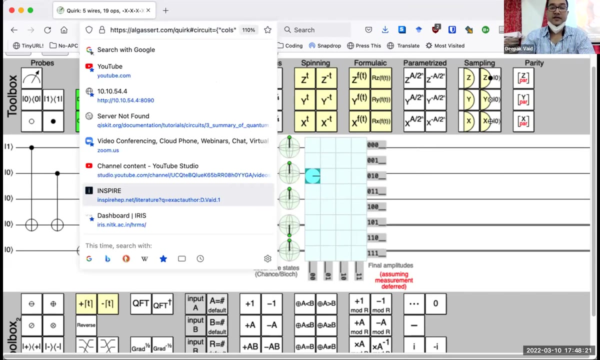 are doing the parity check. This is our syndrome measurement. And then the last set of three components is performing our recovery. Right, And once you have this in Quark- by the way, Quark has a very nice, nice aspect- that the URL itself right, if you look at this URL, it contains all the information. 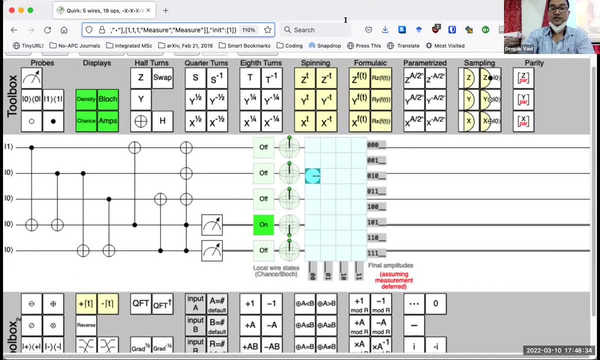 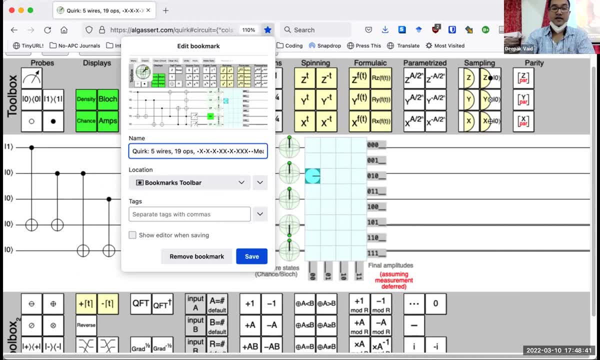 about the circuit. It contains the full circuit. So if I just bookmark this URL, okay, if I just bookmark this URL and then I can give it a name Right: Quark C qubit single bit flip error correction code: Right, And I just save it. 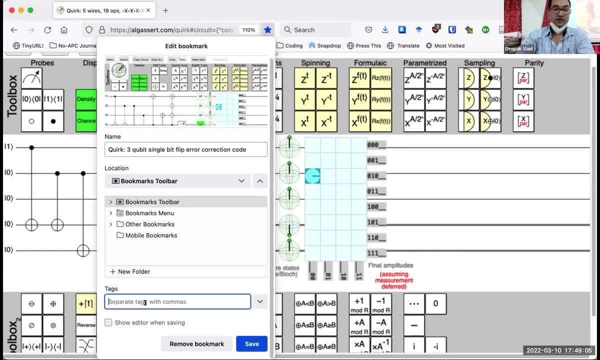 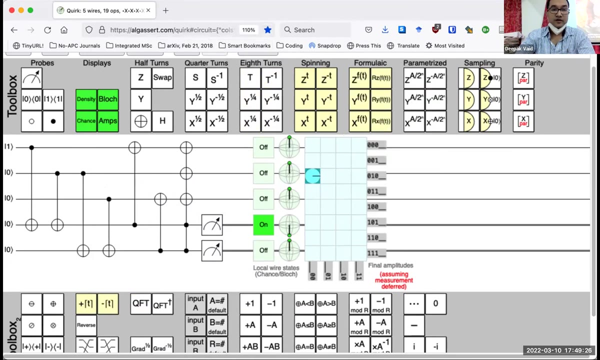 in my whatever I can call it- Quantum circuits, let us say Quark quantum circuits, Okay, Sorry, new folder: Quark quantum circuits. Then it is saved. And whenever I want to look at this thing again, what do I do? I go to my, my bookmarks, And, well, I look at. 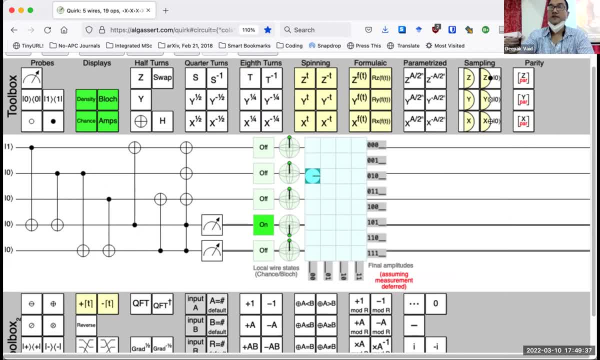 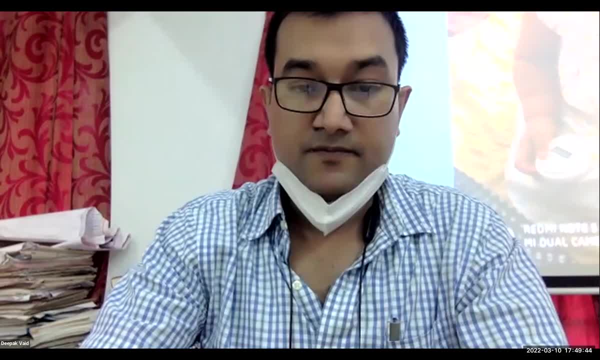 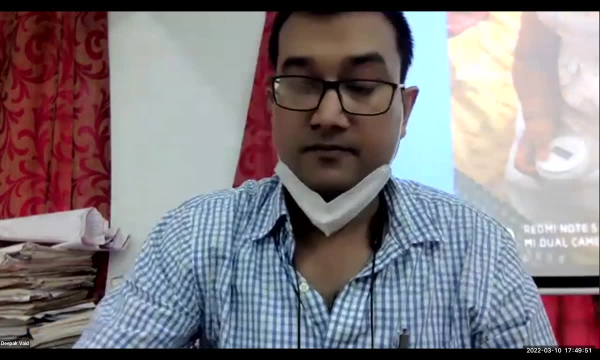 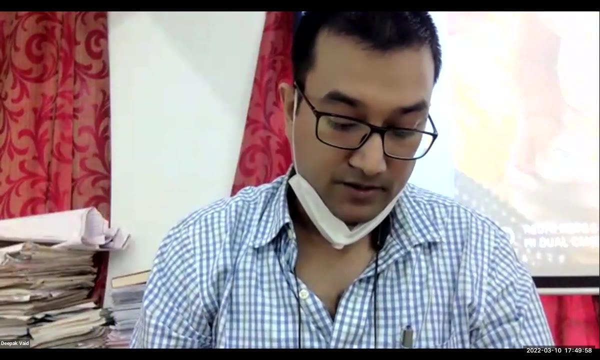 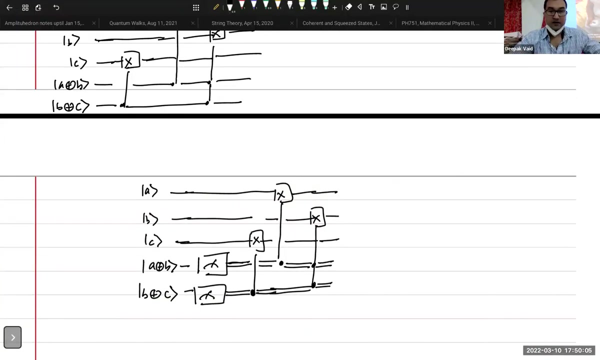 my Quark quantum circuits and I will get this Right. Okay, any question from the Zoom people? Zoom people, any question? No, Okay, then I will continue. I will move on to the, to the next part, And okay, great, Excellent. 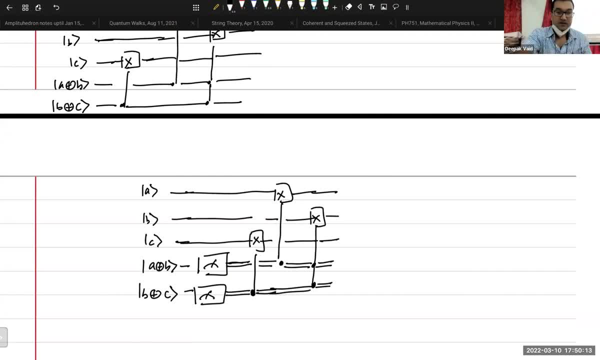 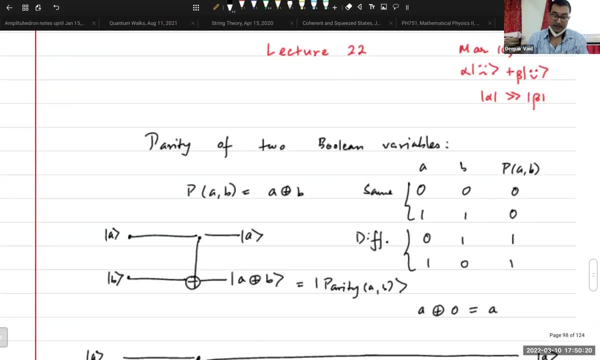 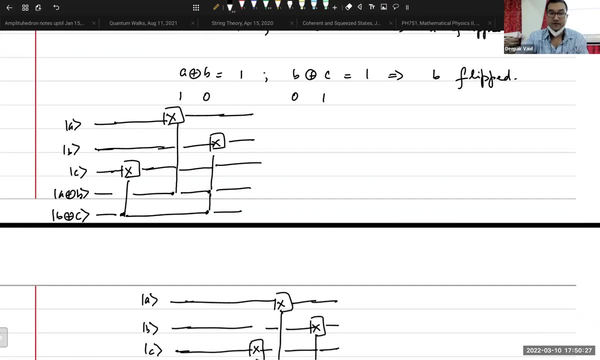 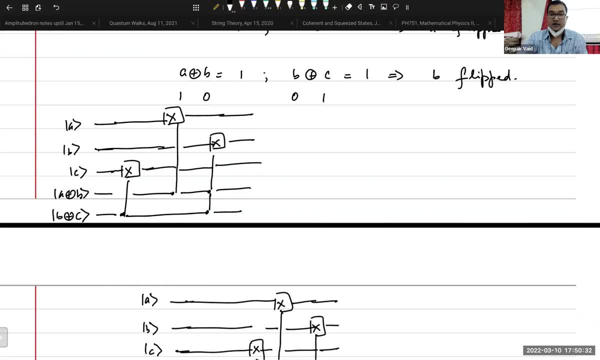 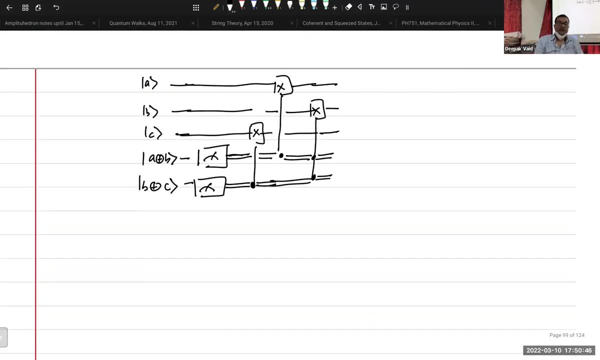 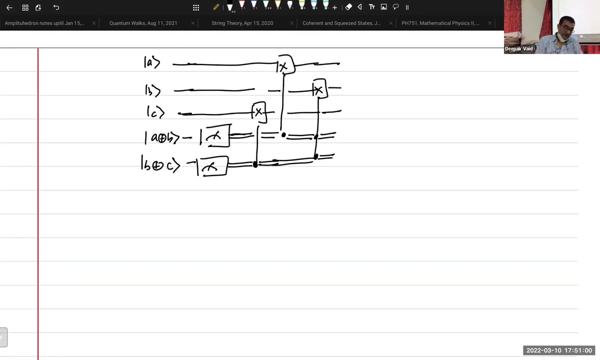 Now there are there are some more very useful circuit identities which are important to know. The first is that how can one perform a measurement of an operator without destroying the state, So as an example. so what we want to do is we want to measure operators which act the 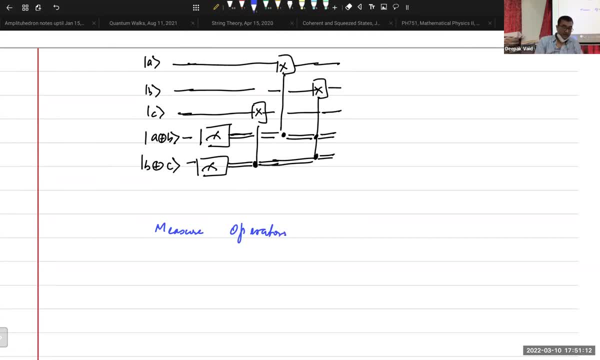 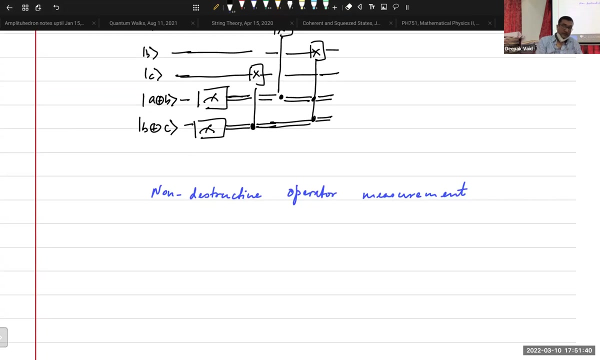 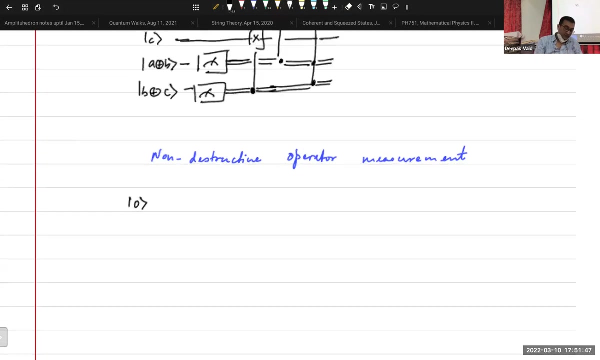 action of some operator on a state Without destroying the state. So maybe I'll call it non-destructive operator measurement, right? So now here's a circuit for that. as an example, I have some ancilla qubit. actually I'll put my ancilla. 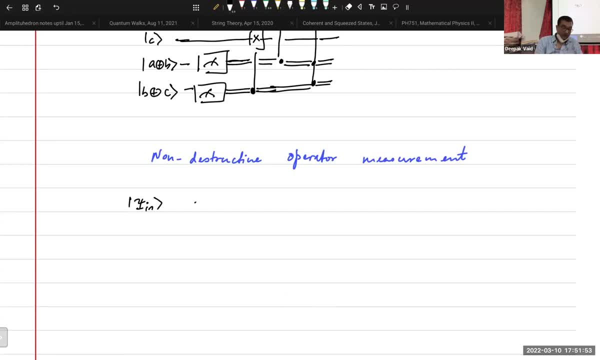 So this is my state, psi in I have some unitary operator, u. I want to ask what is the result of u acting on psi? I want to measure, I want to measure this, this state, Okay, Okay. Is it possible to do it in a way that does not cause this original state to collapse? 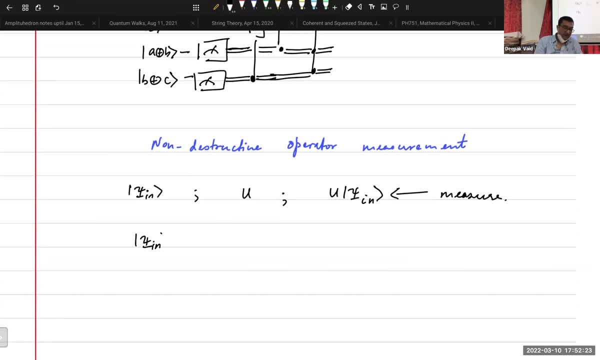 Right, And the answer is that it is possible. Again, we use an ancilla. This ancilla is what will? it will store our result okay, And here it's important to keep in mind that you cannot do this for an arbitrary operator. 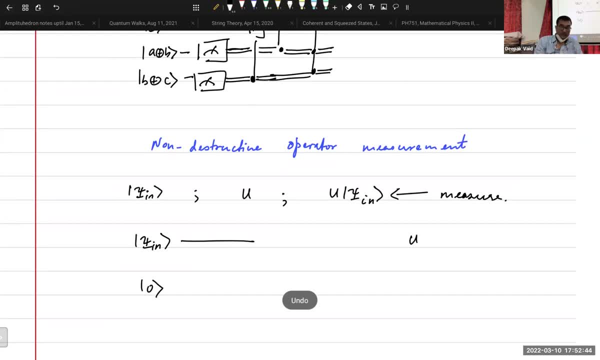 okay, You must be commision and unitary and it must have eigenvalues plus or minus, 1 only okay. Now, I am not saying that this cannot be done for arbitrary operators. maybe it can be done, but this method works only for this set of operators. 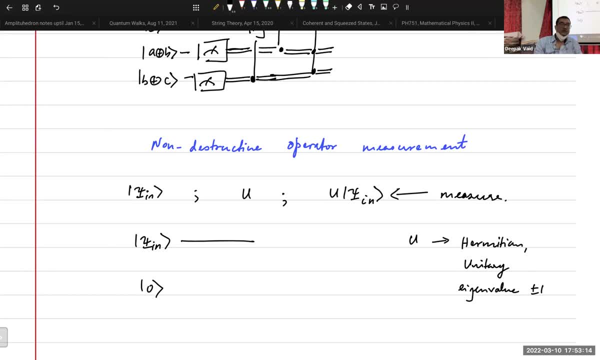 Okay, This is enough for most many purposes because, remember, when you want to act with this z operator right On some state, z is one of those operators. x is one of the operators if it's acting on the in the in the Bell basis or the Hadamard basis, right. 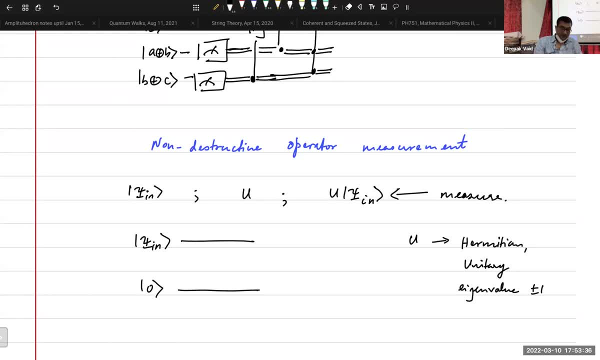 So you have. so the first thing we do is we put the ancilla into the, into the, into the Bell basis, and then we perform a controlled unitary right. So this is a controlled unitary. The control qubit is the ancilla right. 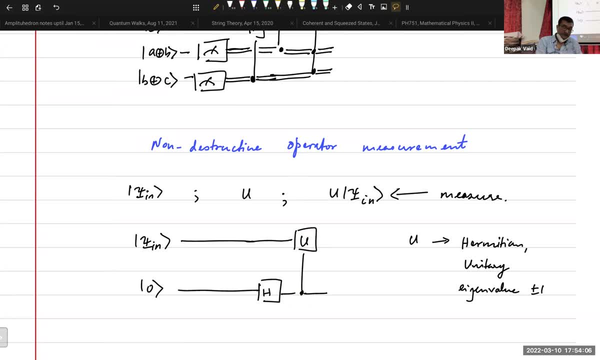 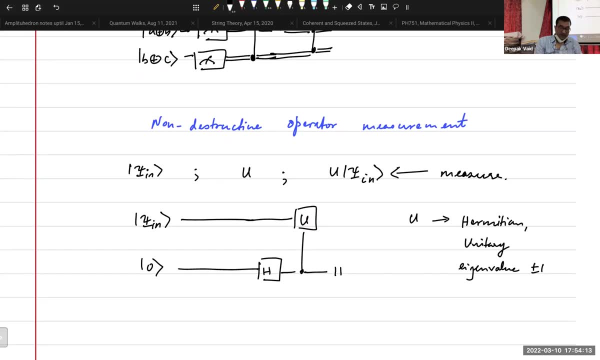 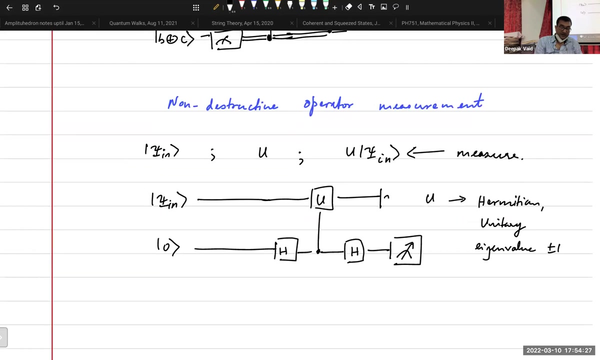 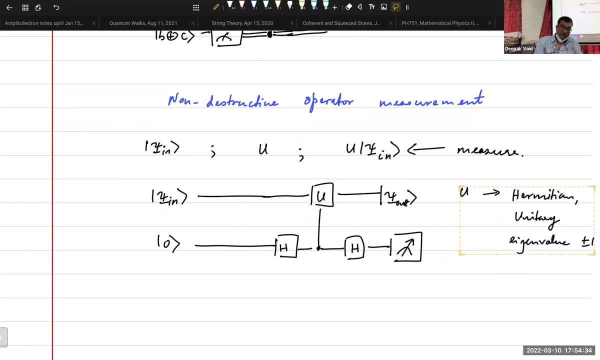 And the unitary is acts on the state psi, Okay, And then we again put a Hadamard here, and then we we measure this, okay, And then here I will get psi out right Where psi out is going to be 1.5.. 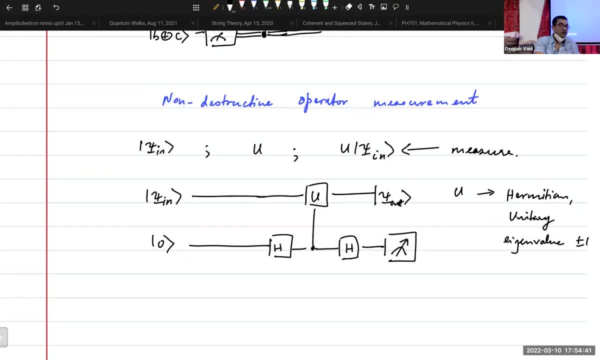 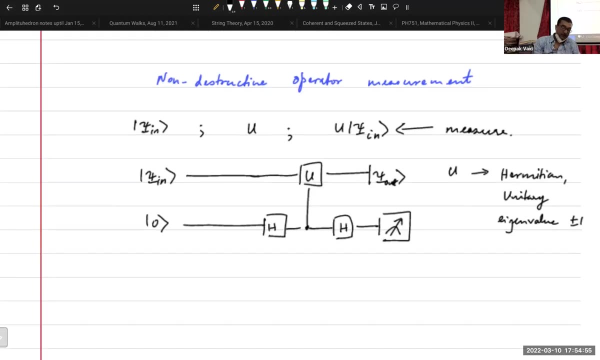 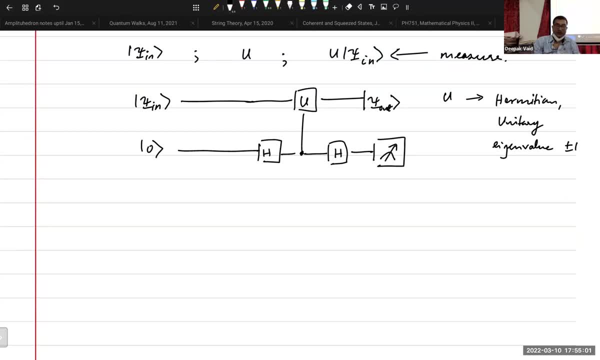 So, in particular, if you are talking about something like z acting on on on some state right Zero or z acting on 1. These are eigenstates of Z, So in this case psi out will be equal to psi in Our original. 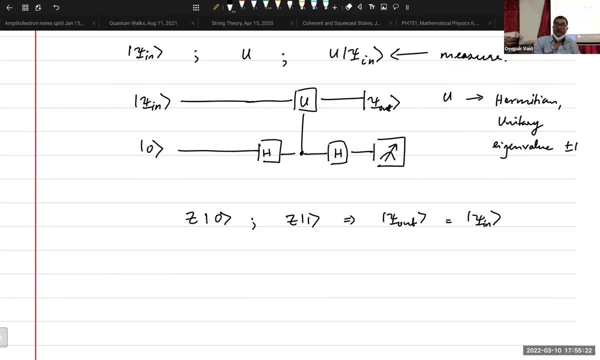 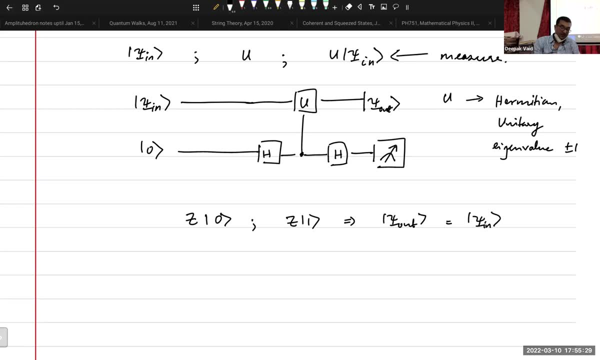 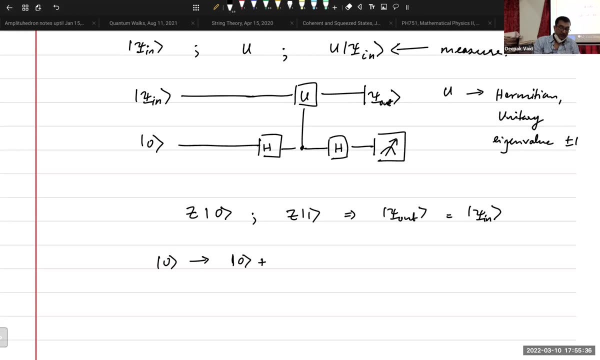 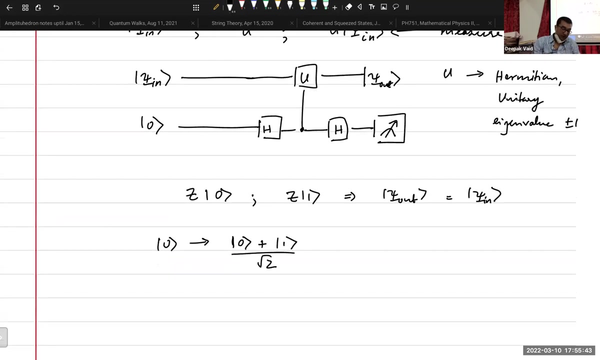 state will not be changed And at the same time, the measurement output here will give me the relevant eigenvalue. So let us see how this works. So the Hadamard takes the zero and converts it into zero plus one. So what is your original state? Original state. 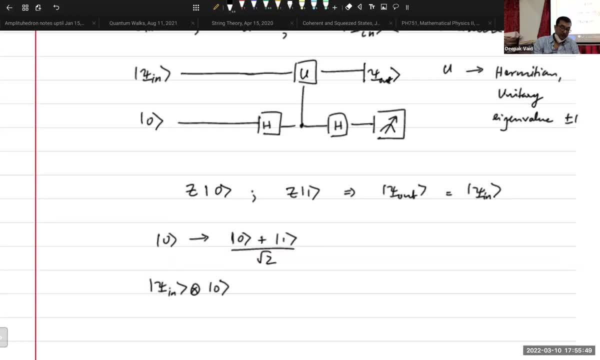 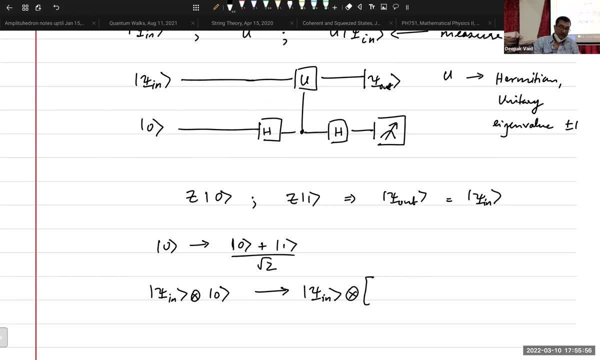 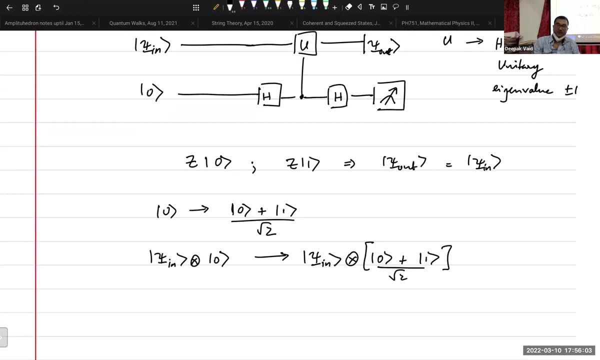 is psi in zero. After the first Hadamard your state becomes right, Psi in tensor, the zero plus one superposition right. And now the unitary operator acts on psi at this point. but it is controlled. So let me write this, Let me expand this out: This is psi. 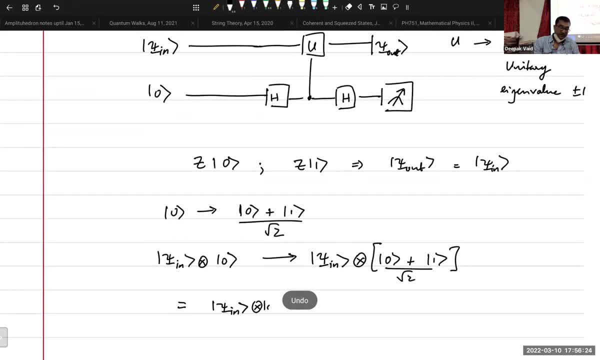 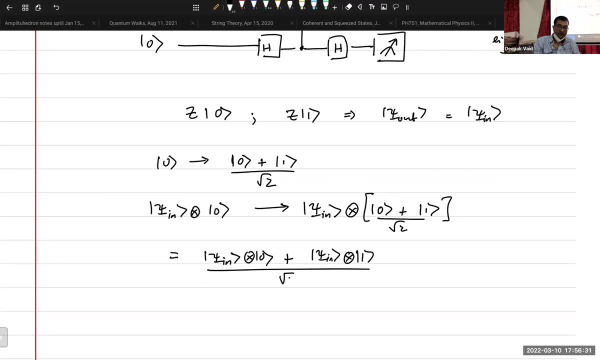 in tensor zero plus psi in tensor one by root, two right, And now there is a control unitary. So the control unitary does what Control unitary means nothing happens to this component. right, Because the control is zero. And this component 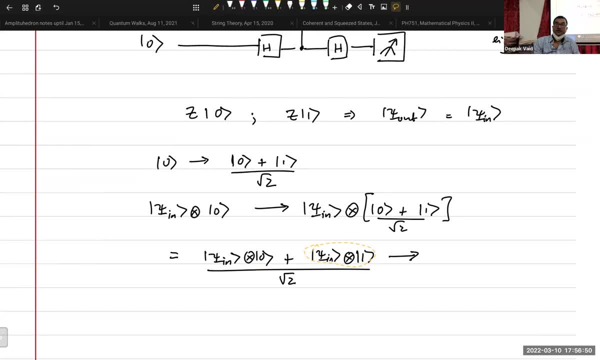 gets acted upon by the given operator. So after this- this is the control unitary operation- You end up with the state psi in zero plus one superposition. So this is the control unitary where you acting on psi in tensor- And I hope you all can see why doing all this- 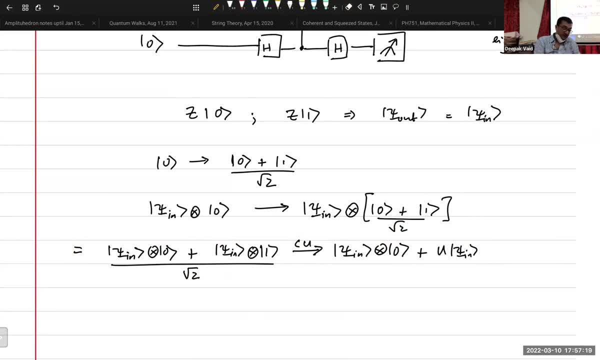 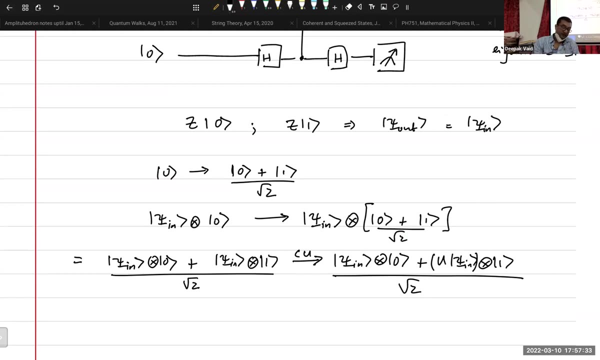 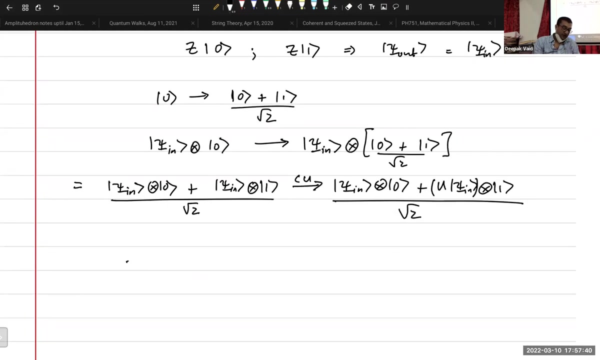 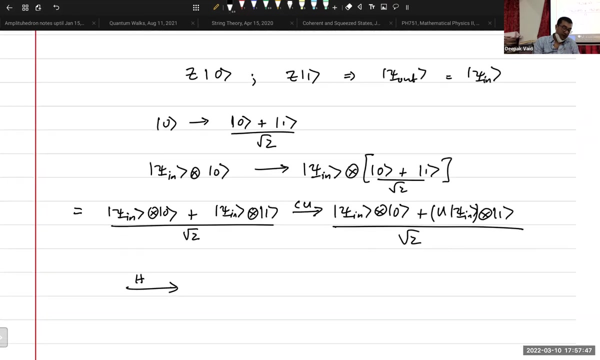 on a blackboard would be not very elegant. You end up with this state where you acts only on psi in, And then we perform another Hadamard, right? So then we perform another Hadamard on our ancilla qubit. What will that do? That will take our zero to zero plus one and the one. 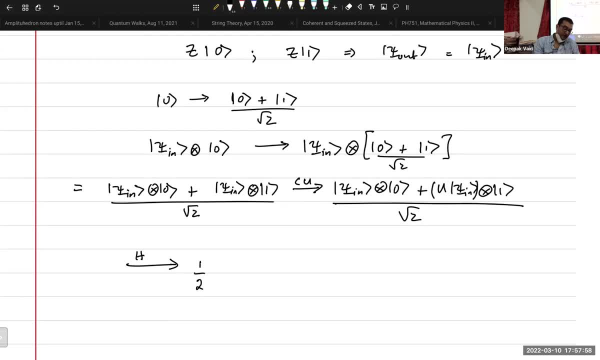 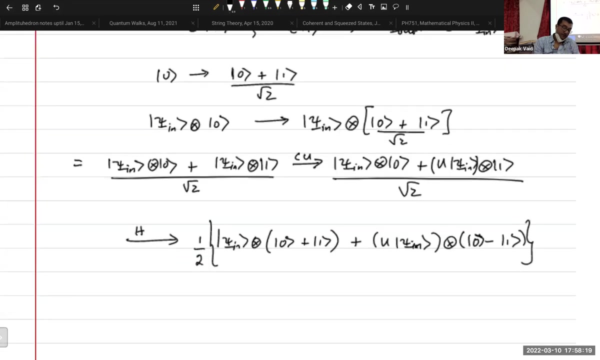 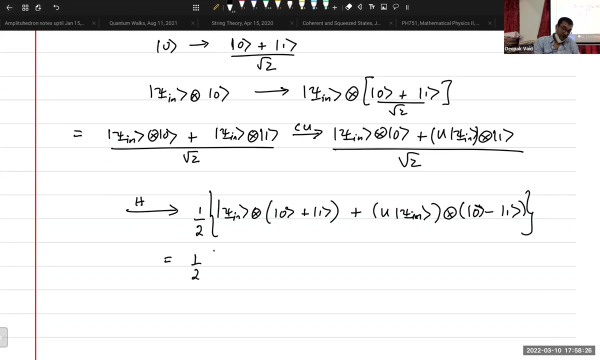 to zero minus one, right. So we get one by two psi in tensor, right. Zero plus one plus u times psi in zero minus one. okay, And let us see what this is. This is one half. Now, if I factor out the terms- and I collect the terms- I get one by two psi. 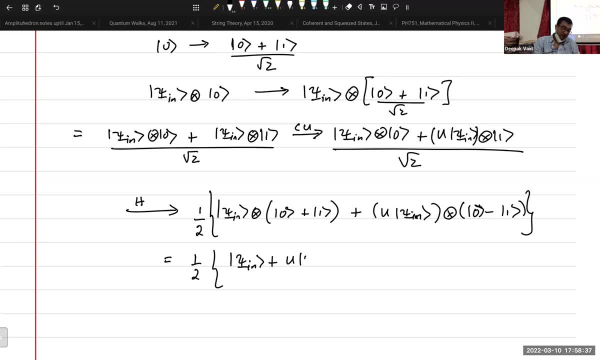 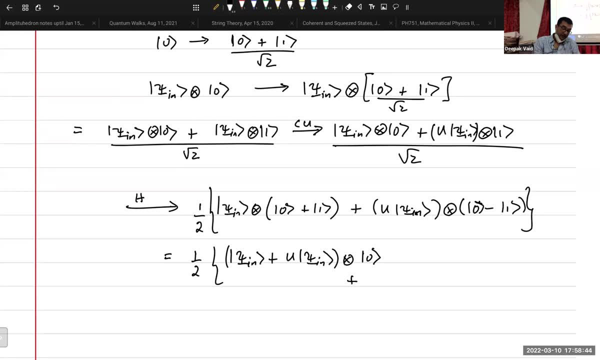 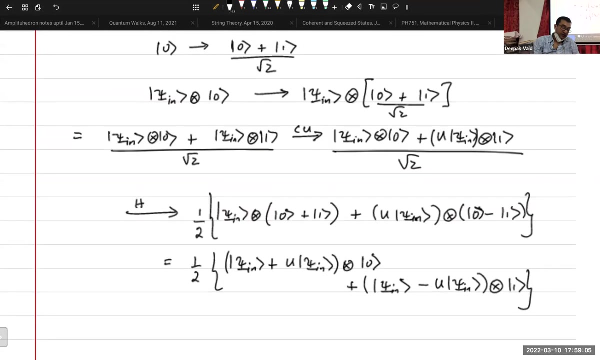 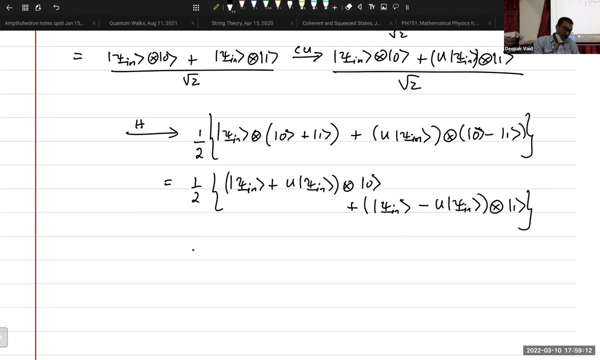 in plus u psi in tensor zero and psi in minus u psi in tensor one. okay, And now what have we said here? We have said that This state, psi in is an eigenvector of u right, So that means u psi in is equal to. 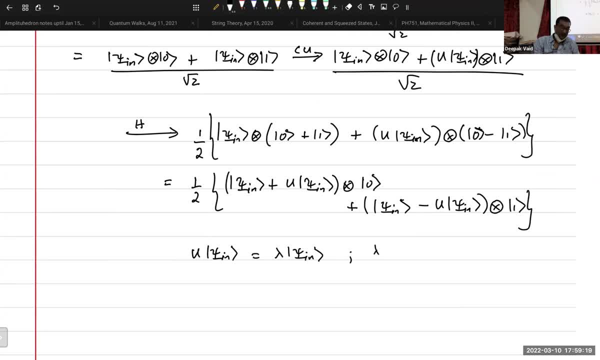 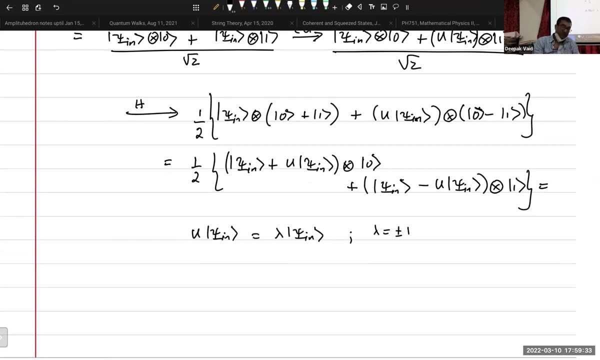 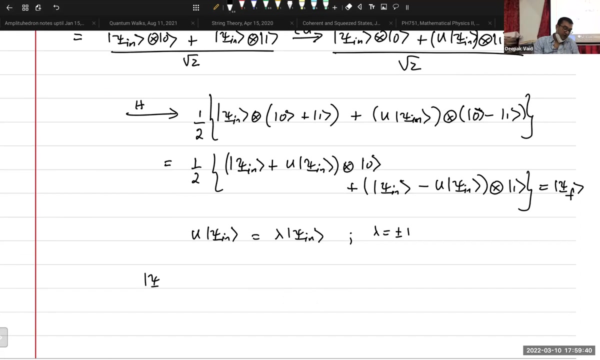 lambda psi in right, Where lambda is equal to plus or minus one right. This is the restriction we have put on this operator u. So then, what happens to this? This is our, this is our final state. Let me just call it psi f. So what is the final state If lambda is equal? 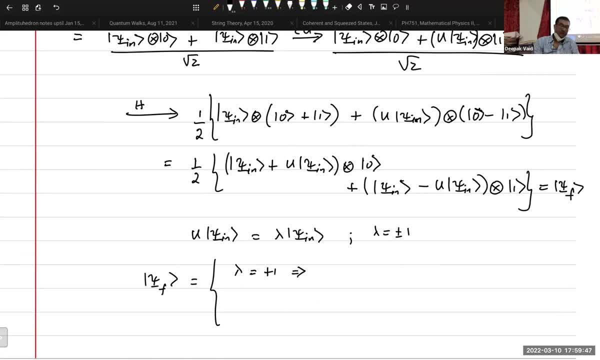 to plus one right. What will happen? This term will vanish. The second term in this expression is psi in minus u. psi in This term will vanish because it will just be psi in minus sine And I will be left with this psi in sorry right, And that is very important. That is. 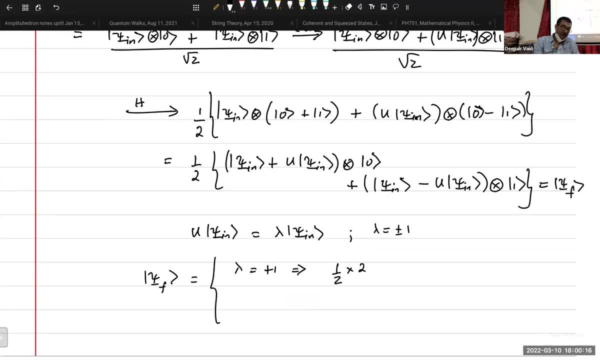 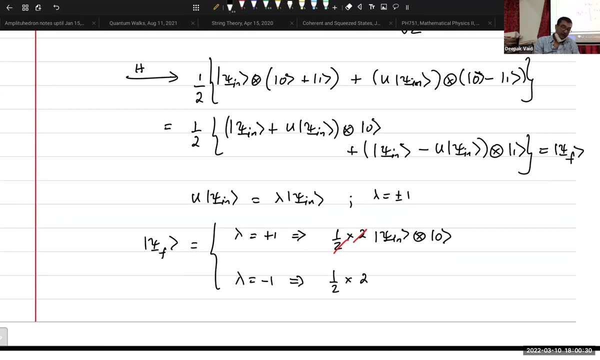 why the factor of one half has to be kept. I will be left with two times psi in tensor zero. The two cancels out. If lambda is equal to minus one, the same thing will happen. I will be left with The same state Because if lambda is equal to minus one, the first term will be zero. 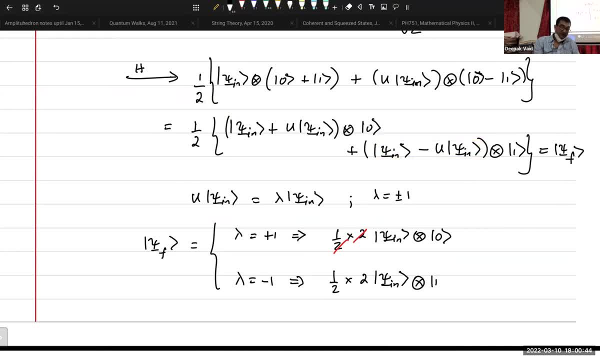 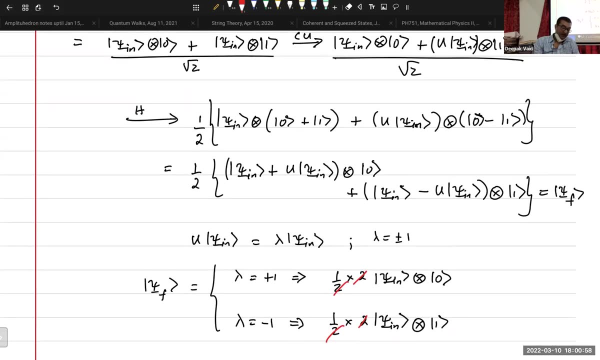 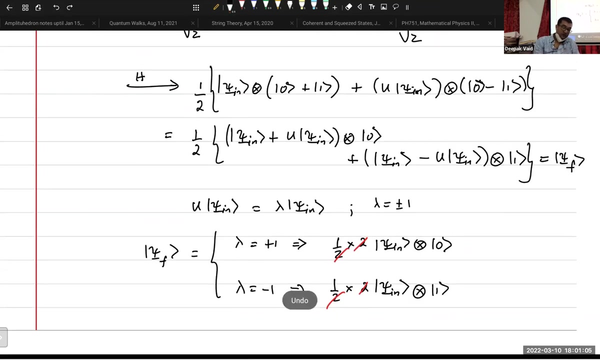 This term will be equal to two times psi in tensor one, And again the factor of two will cancel out right. And now I perform a measurement of my ancilla qubit, right? So if my measurement gives me zero right, So you measure your ancilla. So this tells me that my lambda 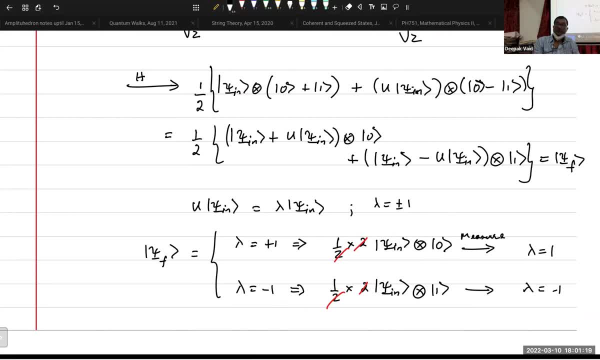 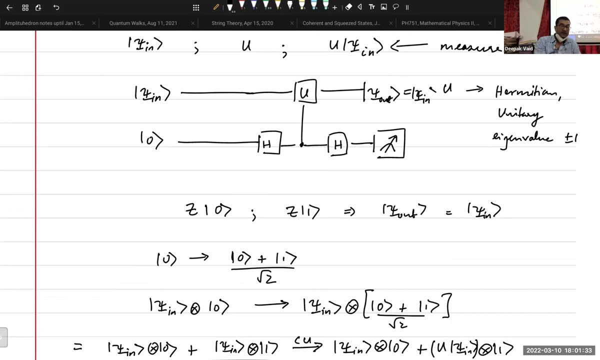 is equal to one, and this tells me my lambda is equal to minus one. So I have managed to non-destructively measure my state. So I have managed to non-destructively measure my state. So the final state that I am left with is psi n and the measurement value of the measurement. 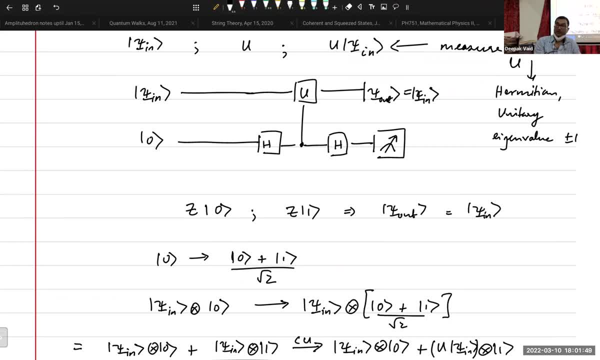 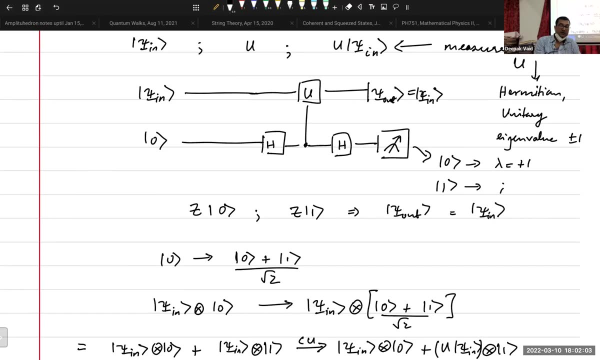 tells me whether the eigenvalue of u acting on this state was plus 1 or minus 1.. So the measurement, if it is 0, that tells me lambda- is equal to plus 1.. If it is 1, tells me lambda. 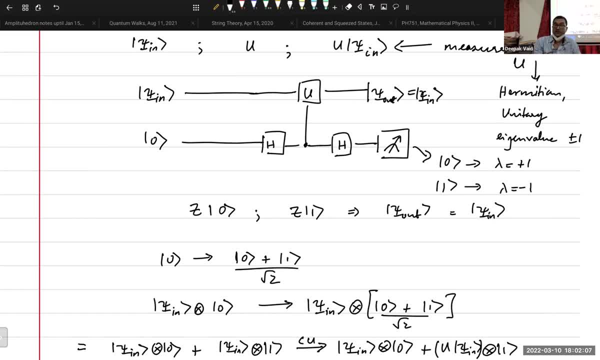 is equal to minus 1.. And my original state is unchanged: It is unaffected by this right. This is really nice, isn't it? I mean, like you just like think about it like it is completely not something that intuitive right- Intuition kind of fails you. 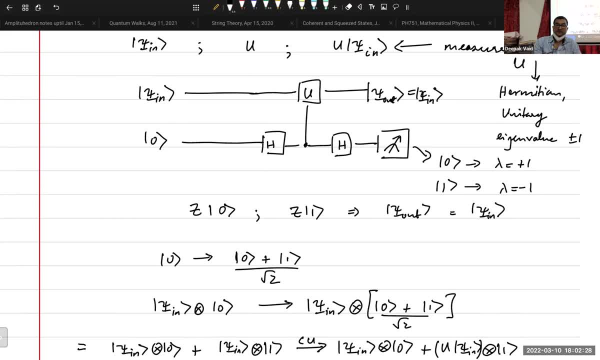 Yeah, but that is enough for many purposes Because, like I said, if you want to measure the syndrome for bit flip errors, the syndrome is what It is: multiples of the poly z, which falls in this category, right, Yeah, Then in the Hadamard basis, if you want to measure again, you want to measure the poly. 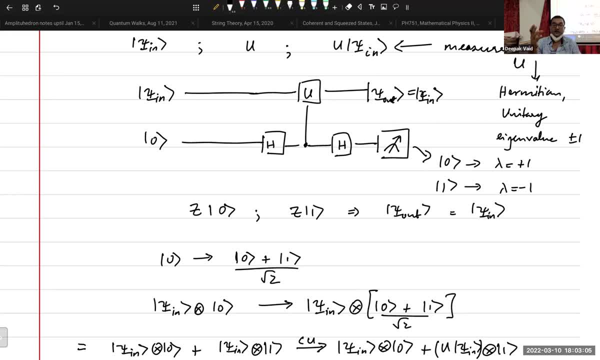 z, but in the Hadamard basis. the same thing for the phase flip. So you would put a couple of extra Hadamard operators in front of the state. to put it in the Hadamard basis like one edge over here then u, then another edge to bring you back. 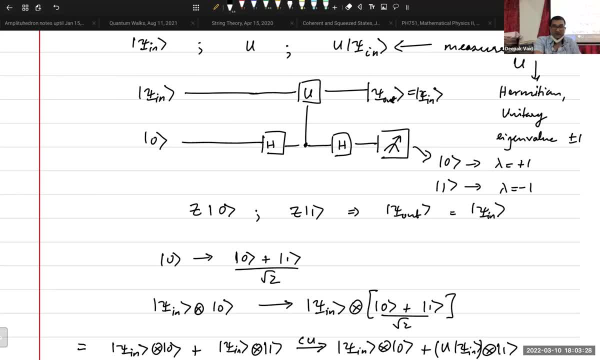 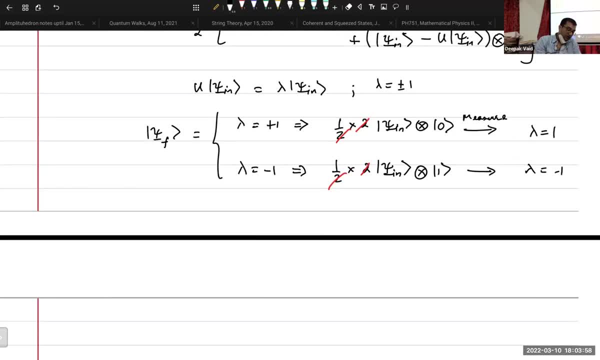 So all the possible syndromes can be expressed as linear combinations of such unitary operators. Actually, more precisely, the correct statement is that all of the errors that can act can be written as linear combinations of these polys. Okay now so let me see second, second, yeah. 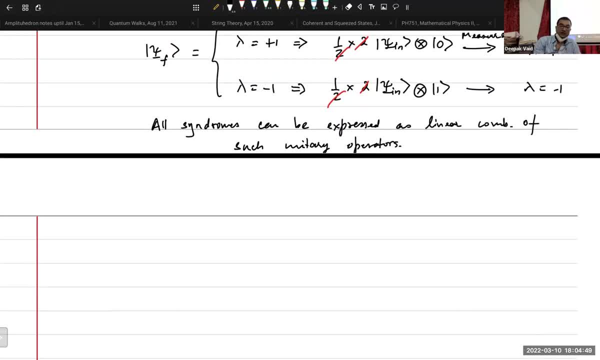 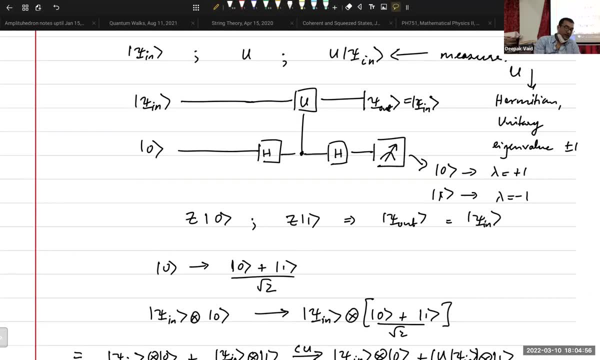 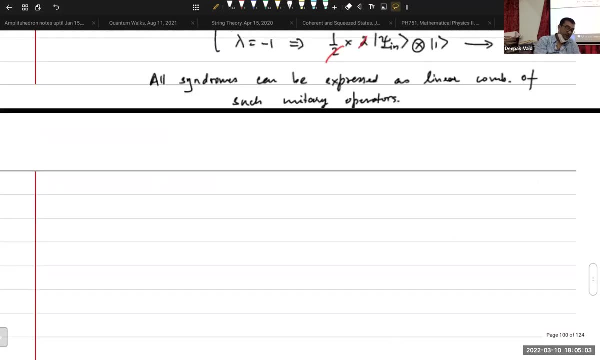 And now there is another very useful identity which comes from this only. So here in this picture, what is happening is I am applying these hard mods to my Ancilla qubit. Okay, Okay. Now this is the following identity, which is this: 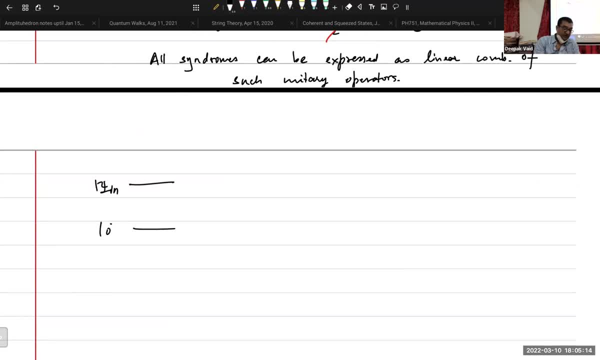 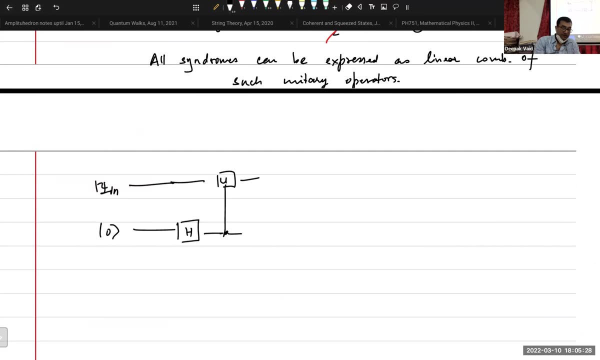 So I have psi in my Ancilla. I apply the hard mod to the Ancilla, Oops, Then I perform a control U right, Then again a hard mod on the Ancilla And I am left with psi in and lambda, which is my eigenvalue right as a measurement. 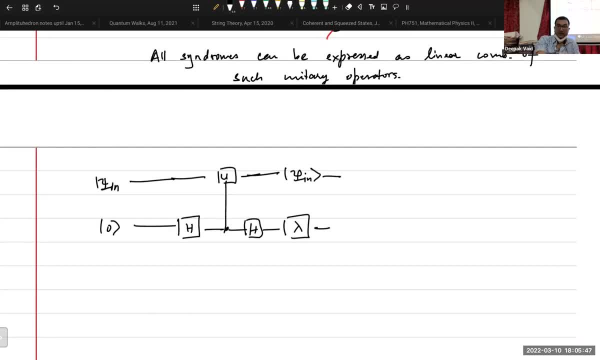 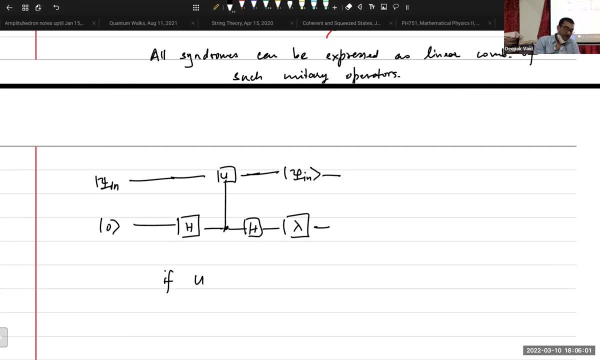 Now the identity is the following: That if U is the X gate, okay. So if U happens to be X, okay, I want to measure the, so let me put X over here, Okay. In that case, this circuit can be alternatively written in a 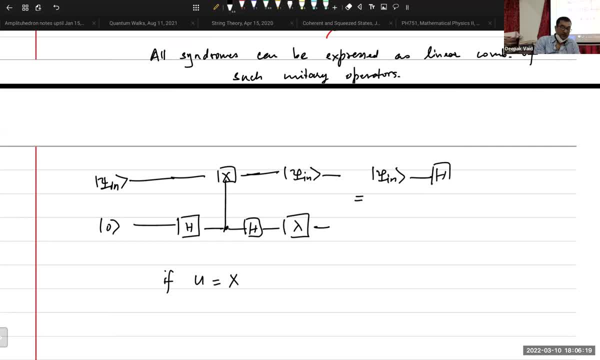 different way. I act on my input state now with the hard AMARD, And then I act on it again with the hard AMARD, And what I have here is I have a control, a CNOT acting on my ancilla, And once again I perform a measurement. 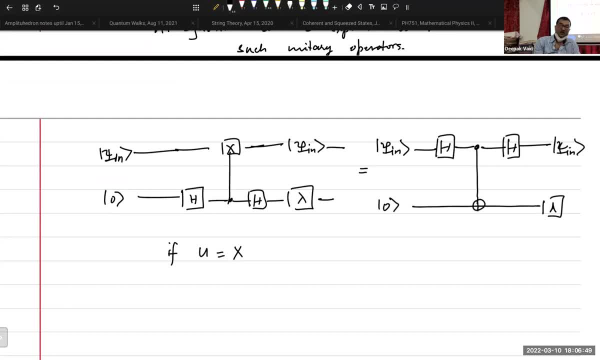 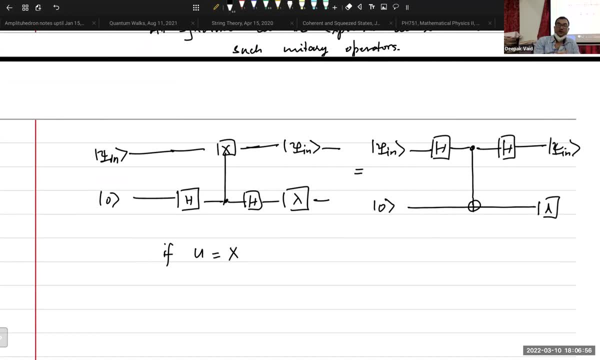 And here it's sign. So the measurement is not important because it doesn't affect whether the identity is true or not. This is an example of what Phase kickback. Phase kickback is the, The operation where you can have a control and a target. 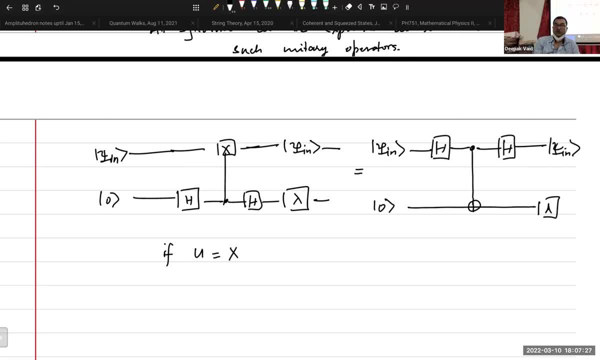 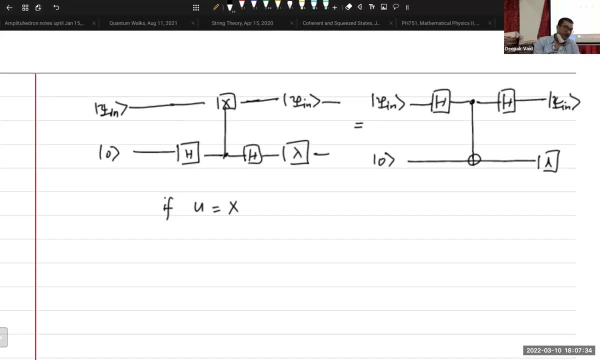 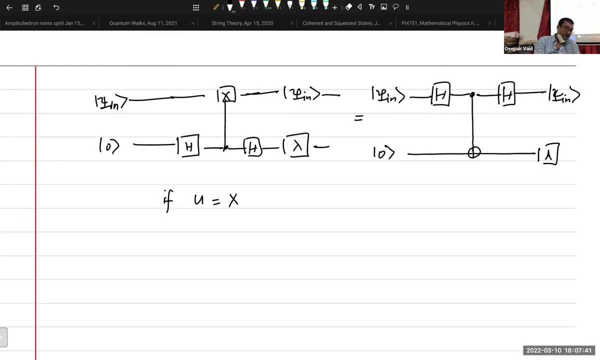 And the target can change the state of the control. Well, I'm not sure if this is. it looks similar to that, but it might not be exactly phase kickback. So this identity holds for the case when u is equal to x. 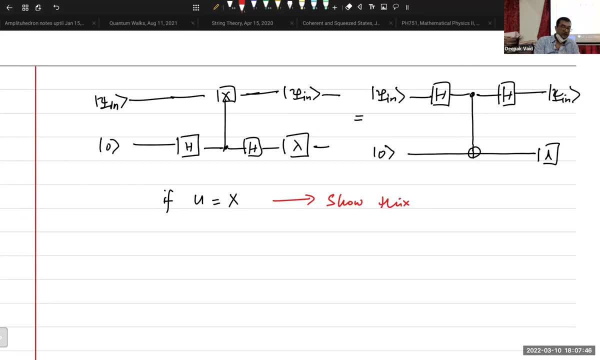 And I will leave this for you, And I will leave this for you, And I will leave this for you. So I will leave this in here as a as a homework, okay, Which will be part of your homework assignment. So this: 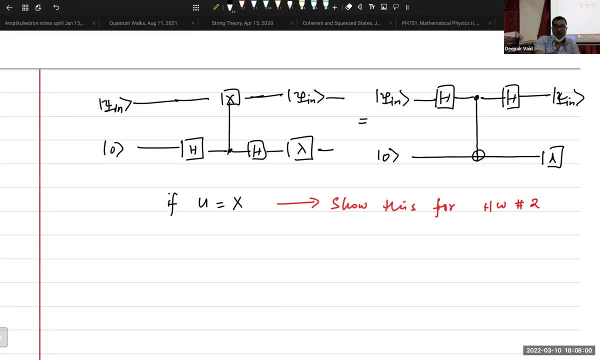 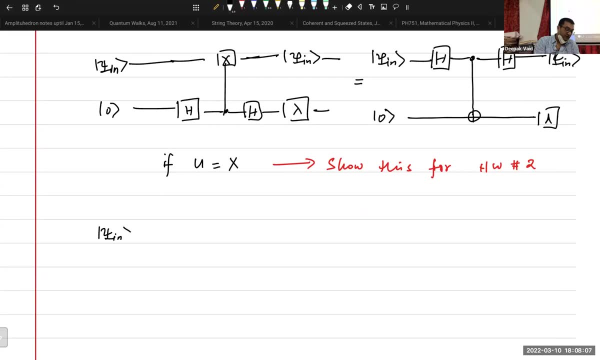 Oh, homework number two. okay, One has a similar identity for the Z operator. If you want to measure the Z operator like this, which is the following again, you know hard AMARD Control, hard mod you have over here, right, you get psi in and you measure the eigenvalue of of. 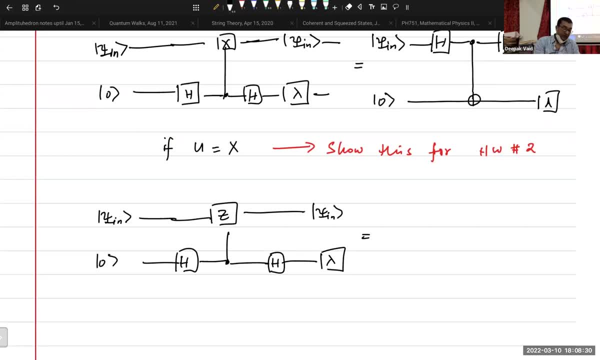 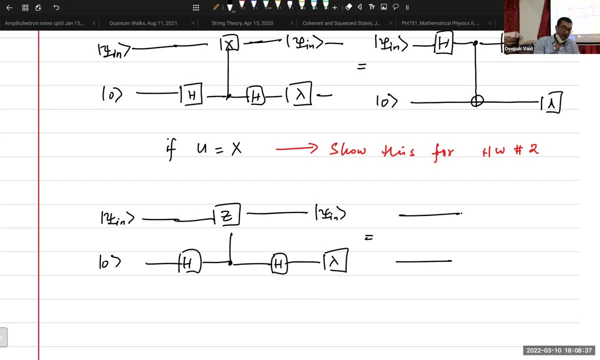 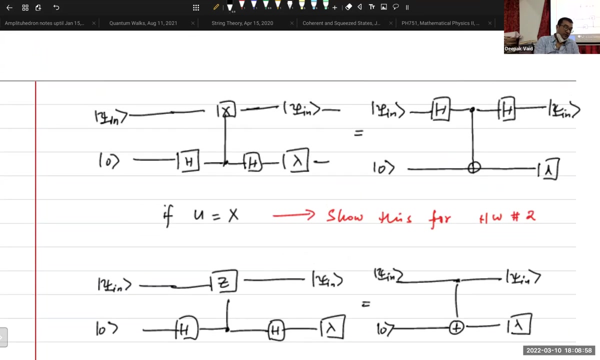 z over here. so the statement is the following: that we can replace this um with the a single c, naught psi in, zero psi in, and then this will be the eigenvalue of z. so what is the statement? the statement is that if you want to measure the eigenvalue of z, 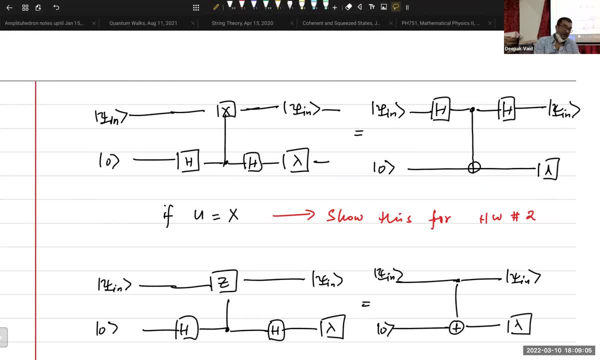 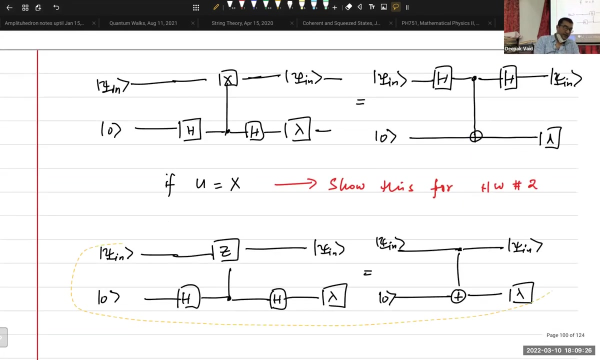 action of z on a state. you take the state, put it into the hard mod basis, right, what? what will this do? this will take all your zeros and ones and convert them into pluses and minuses, and then you measure. you perform the c? naught operation now from the second identity. what you can see is that this c? naught operation 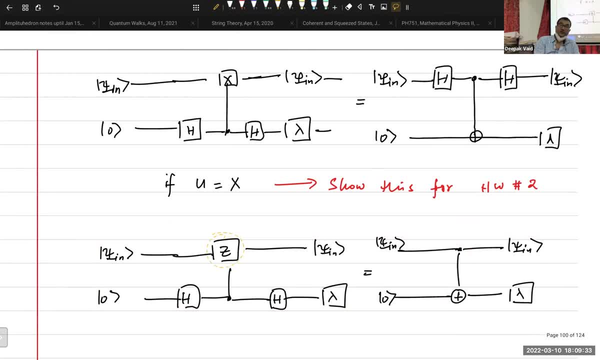 what does it do? it measures the eigenvalue of the z operator. so you are measuring the eigenvalue of the z operator in the hard mod basis, right. which is what? which is the measurement of x in the hard mod basis? what happens to the x operator? it becomes the z operator. right, it becomes diagonal. 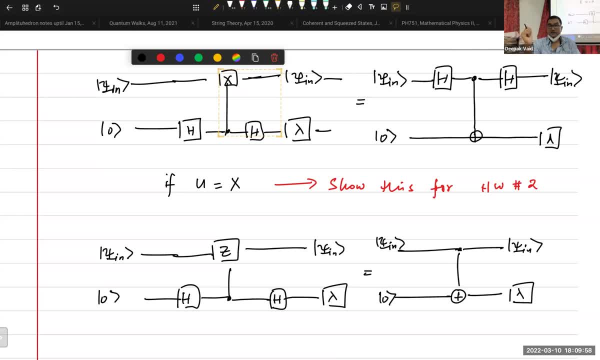 the plus and minus states are eigenvalue, eigen states of the x operator. so maybe, like you, are all reaching such a point that you are not able to measure the x operator, so you can see that there is an acceleration now. so this is, i would call this, the first identity. 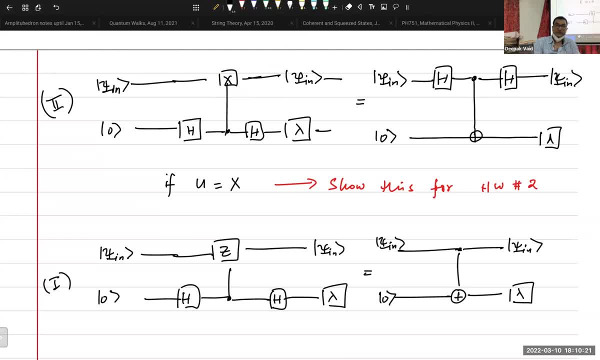 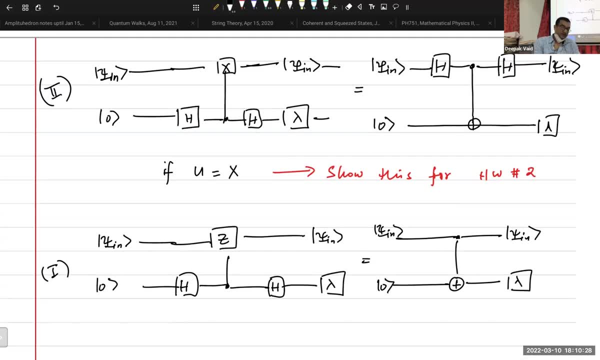 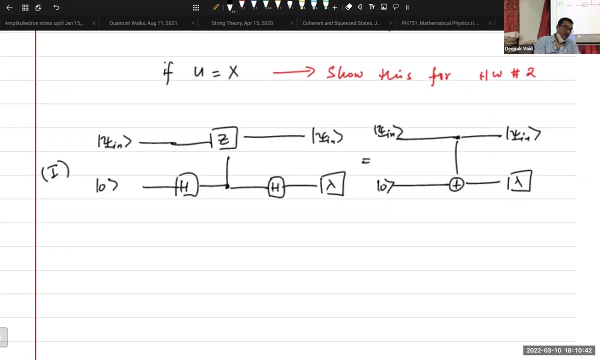 so this is- i would call this- the first identity that you should prove, and then this will follow. the second identity will follow as a consequence. let me, let me just So, let us just look at the second identity really quickly. Let us say: psi in is equal. 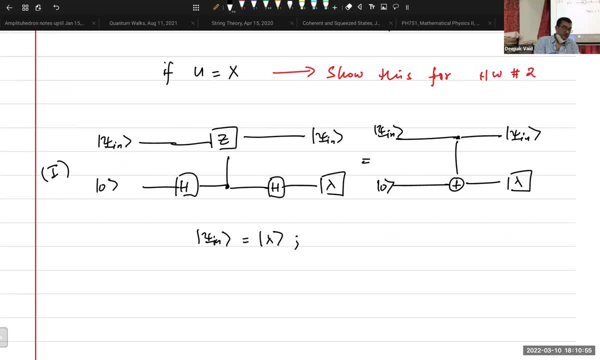 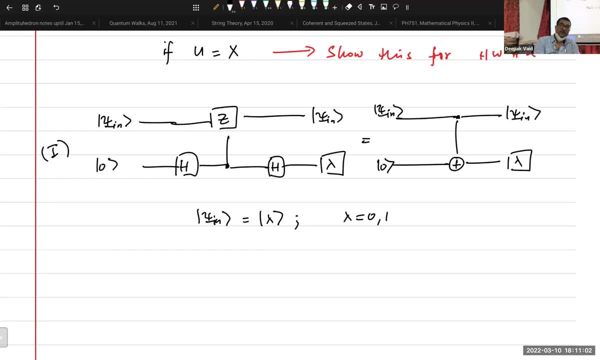 to this state lambda, where lambda is equal to 0 or 1. Then I act with the CNOT operation on the ancilla qubit. If lambda is equal to 0, what happens to the ancilla qubit? Nothing happens to the ancilla qubit And when I measure it I find lambda is equal to 0.. If lambda- 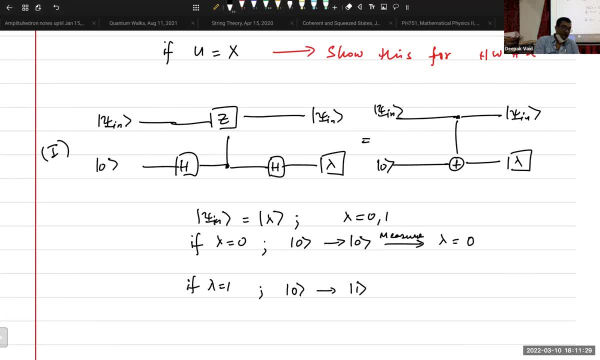 is equal to 1, then my ancilla qubit is flipped. When I perform a measurement, it tells me that lambda is equal to 0. So this circuit is doing exactly what is advertised, which is it is measuring the effect of the z operator, It is measuring the eigenvalue of the z operator on my state. And since we 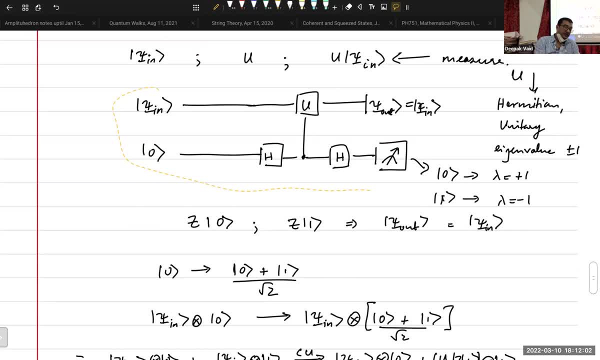 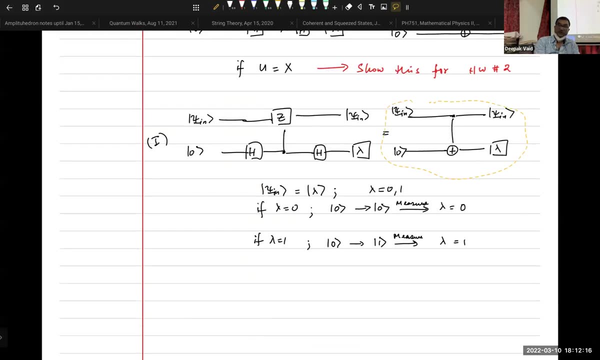 have already seen that this is the general form. So this is the general form of the circuit when you want to measure this kind of a unitary operator. And what is this circuit doing? It is measuring the z operator. So that means. 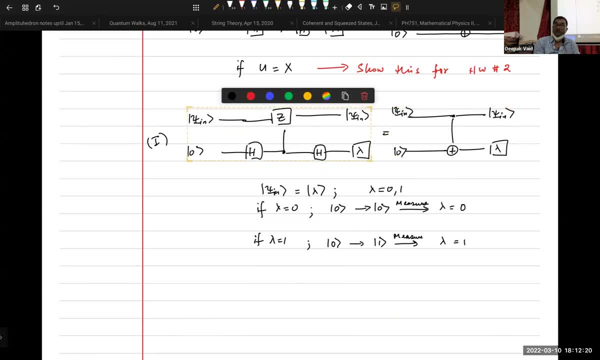 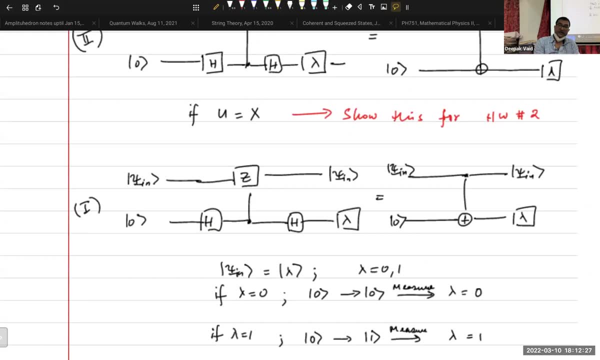 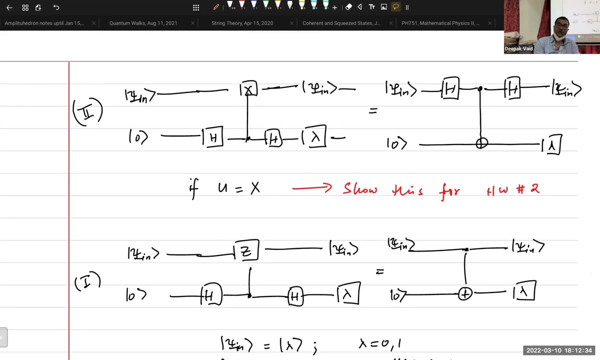 this circuit has to correspond to the circuit with u given by z. So that is proved, And now let us see what happens, Okay, Okay. So let us say: you want to measure this thing, this x operator, right, So to measure the. 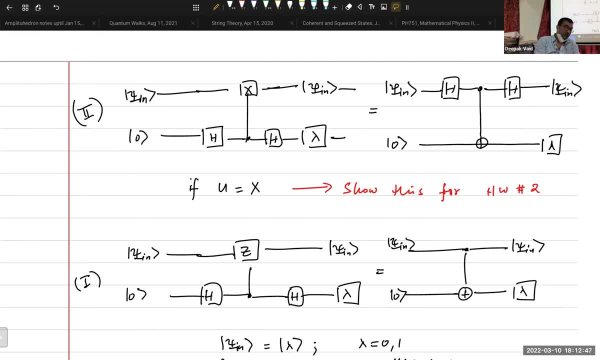 x operator. what do you do? You take your state psi, put it in the Hadamard basis. Then you measure the z operator on your state when it is in the Hadamard basis. Now how do you measure the z operator? 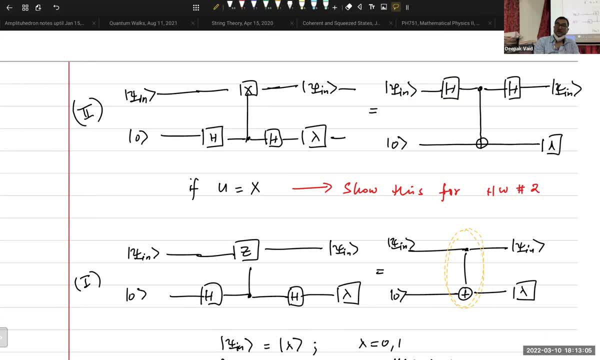 You measure it by this c naught. Okay, This c naught gate, As we have just shown, putting this c naught gate measures this input state over here, the action of the z operator on this state. And then we put another Hadamard. 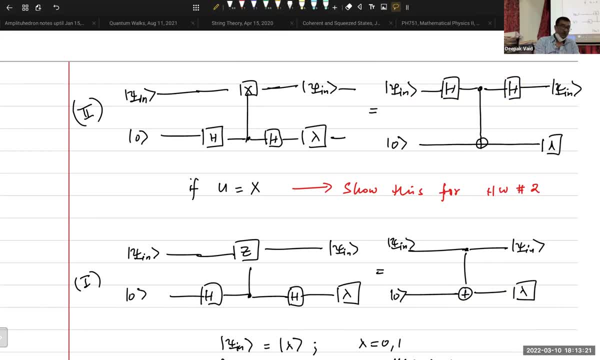 to go back to our original state. So this operation together, what will it do? It will measure the x action of x on the state. So therefore, this has to be equal to the input state. Okay, This is equal to the circuit on the left-hand side, right. So this is not a mathematical. 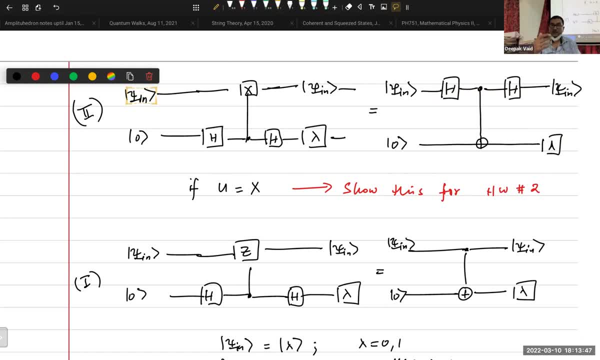 proof. I mean: well, you can, but it is not in mathematical language That I will leave for you, for the homework right, To work it out step by step that this is indeed the case. Okay, So let us see. Okay, Zoom people can I take and all of you can I take some more time? 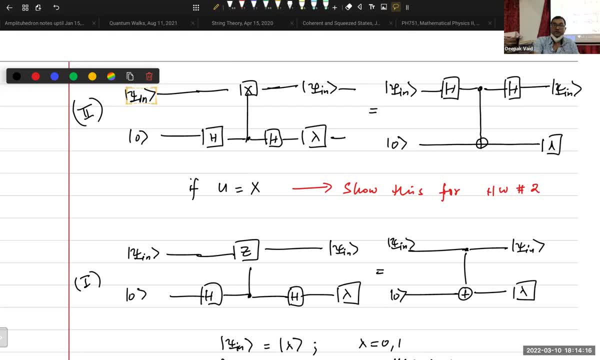 Do you guys have to go anywhere? Can I take another 15 minutes? Is that okay with all of you on Zoom? Please say something. Okay, Okay, Okay, Okay. Yes, sir, You can. I will assume that, in the absence of any statement from you that it is So what I want to do. 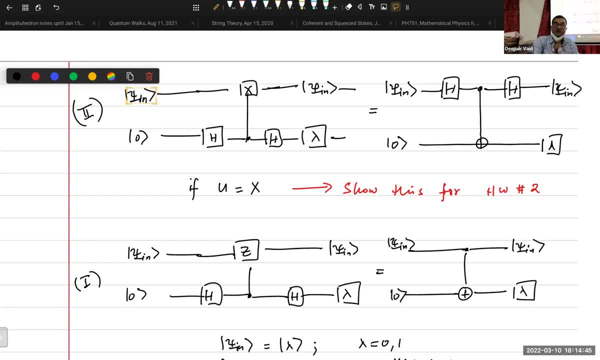 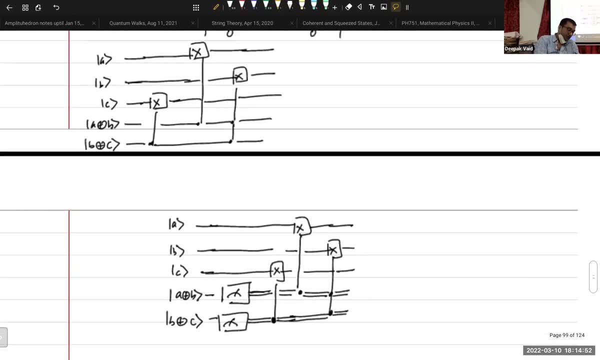 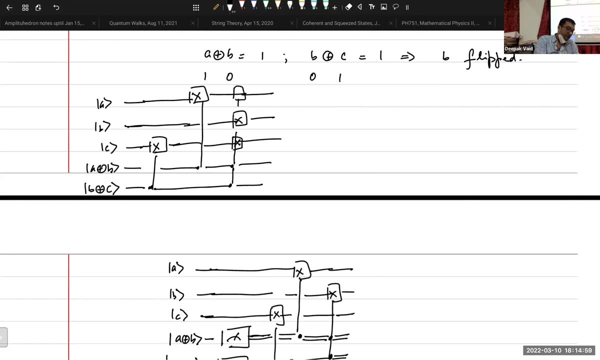 is. I want to talk about the phase flip code also. Okay, So we have already talked about the bit flip code And I hope that I have convinced you, with the correction very nicely provided by Utsav and the rest of you, that this should be a correct. 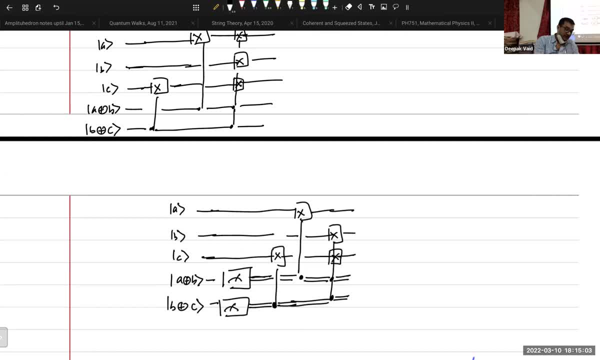 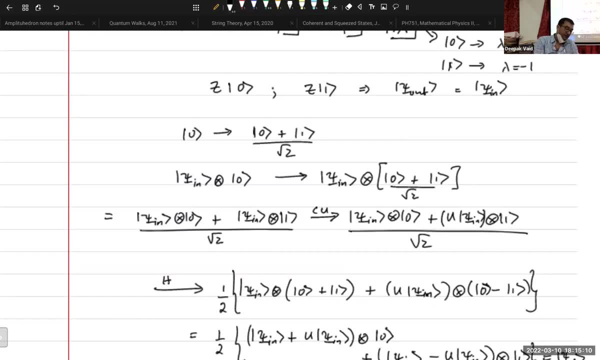 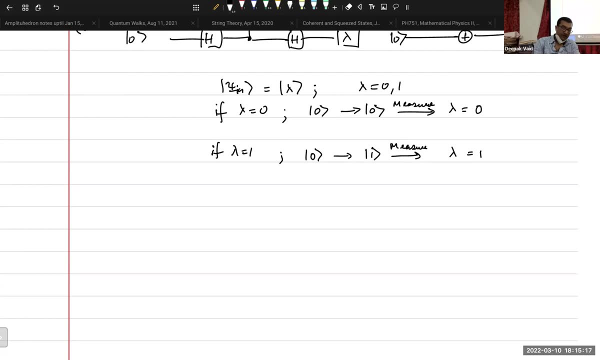 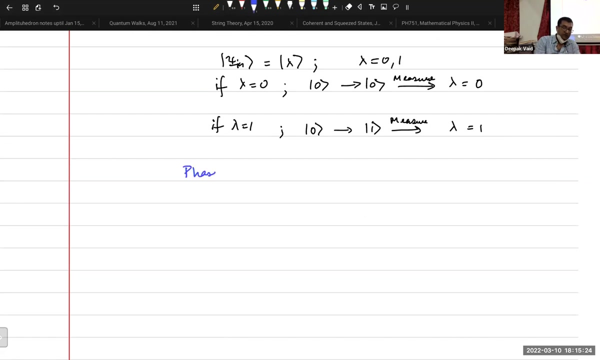 Okay, a cc xxx gate, right? this gives us our correction for the bit flip, for a single bit flip. now we want to do a correction. we want to do it for the phase flip, right? so what is phase flip? so we have done the correction for so: phase flip, recovery and diagnosis: recovery and sorry, diagnosis and recovery. 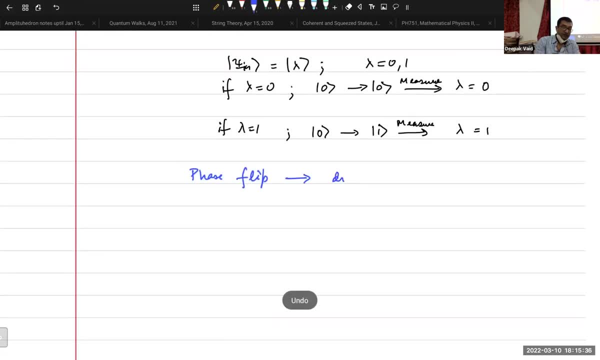 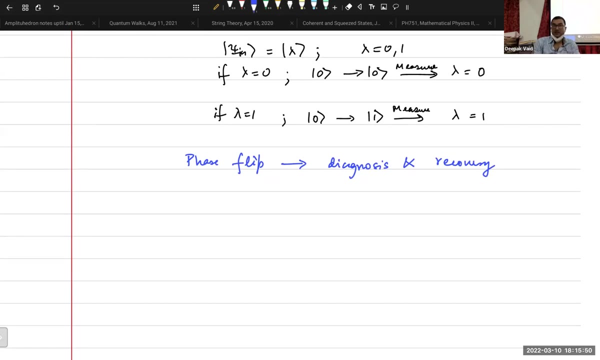 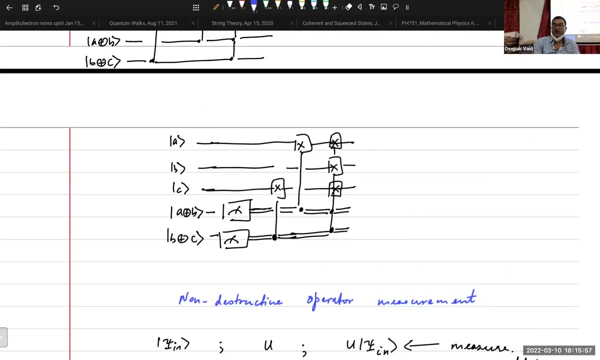 circuit: diagnosis and recovery circuit. right now, before i show you the circuit, i will ask you to make a very simple circuit simple. guess, can we modify this circuit in some way that you will? you know, in a simple way that will give us the phase flip instead of the bit flip check. 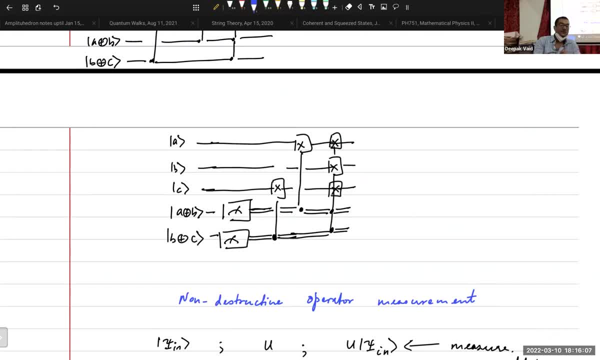 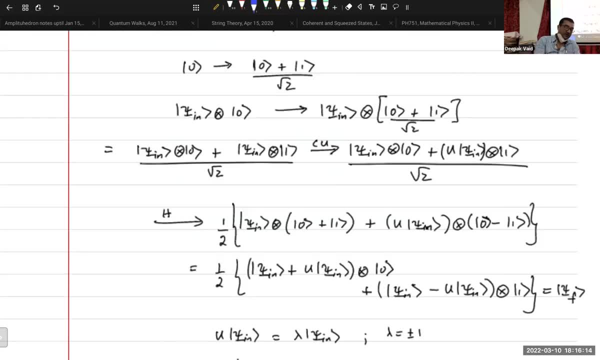 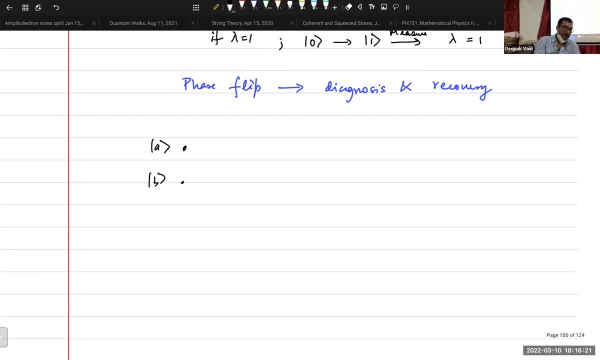 right, that's the most obvious thing one can do is just take these states right and act on them with, with hard amounts, and that's exactly, uh, what one has to do. so you have a, b and c right, and now you want to check for the phase flip. so the phase flip means 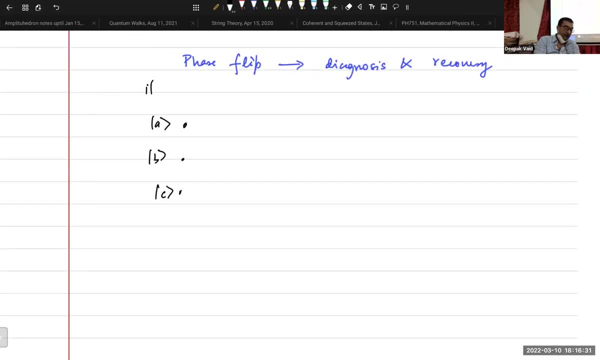 that if a, if the state a, for instance, is of the form zero plus beta one, right, a phase flip error means that you go to zero alpha, zero minus beta one. so first of all we just put all of these in the higher amount basis out and then we perform our parity check as before, with one c naught over here. 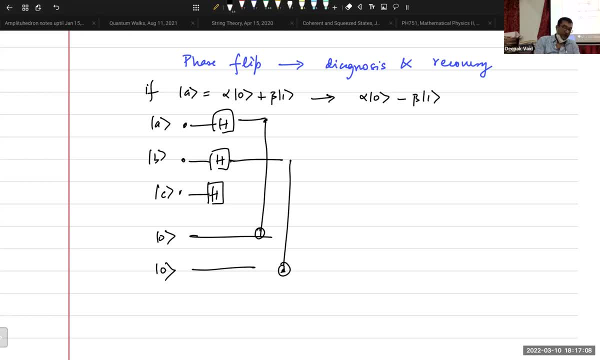 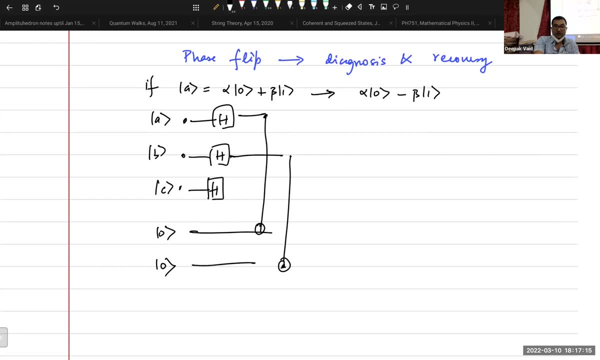 one c naught over here. and, by the way, this operation with with multiple, where you have one c naught followed by another c naught, it can be abbreviated and written as: rather than putting two CNOTs in a row, one second. no, no, no, not this. 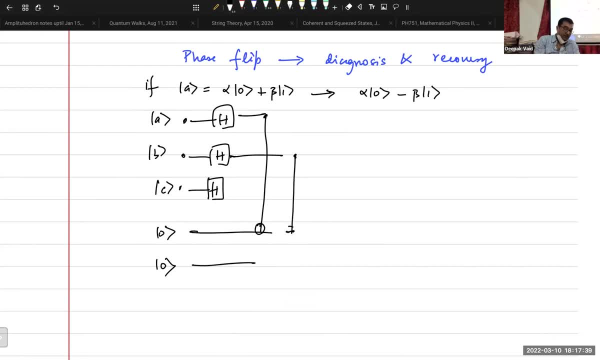 circuit. that's a different circuit, so I won't do that. yeah, yeah, this, okay. so this is the parity check for the first qubit, first two qubits, and then we perform the same operation with the second and third qubit. okay, so this is this performs our parity. 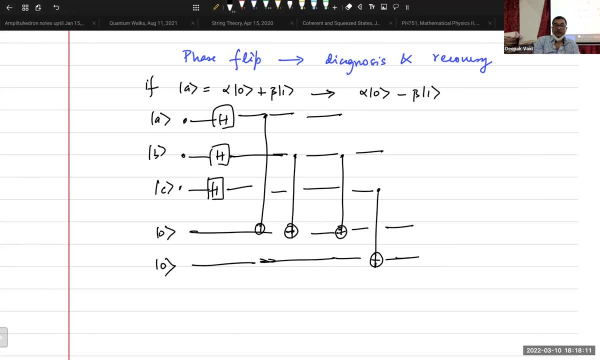 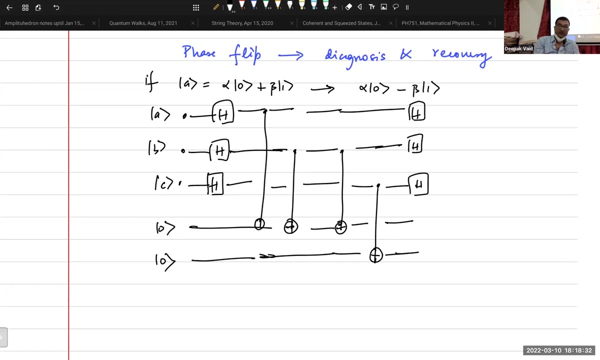 check right in the hardware basis. but now what we want to do is we want to apply again hardware after this, So that we can come back to the normal basis right, because our states have been modified. we want to convert them back right and then after this, the correction procedure proceeds. 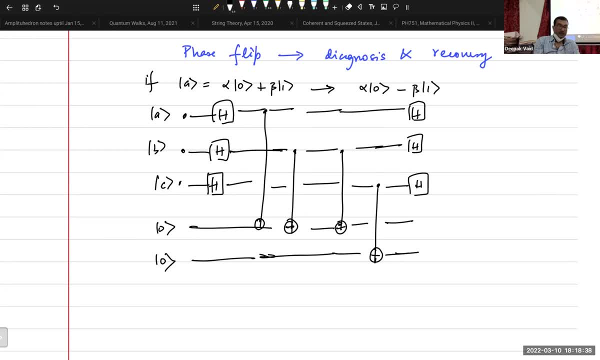 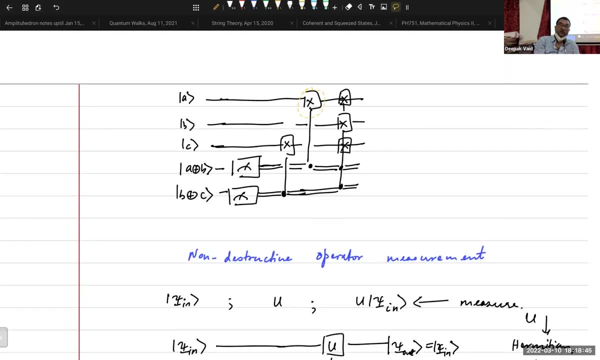 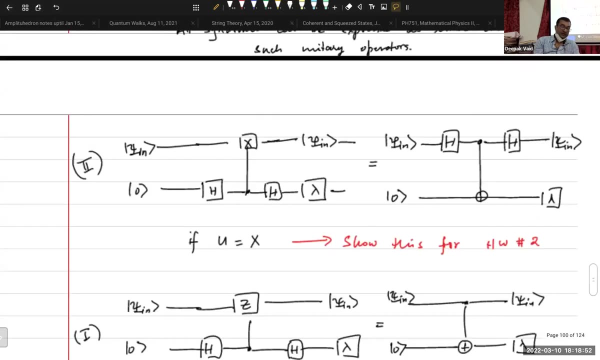 as in the same way, right. so here the correction procedure involved. what Here the correction procedure involved? the X gate. why the X gate? Because the X gate is what flips your qubit. Which gate flips your phase Z, Z. 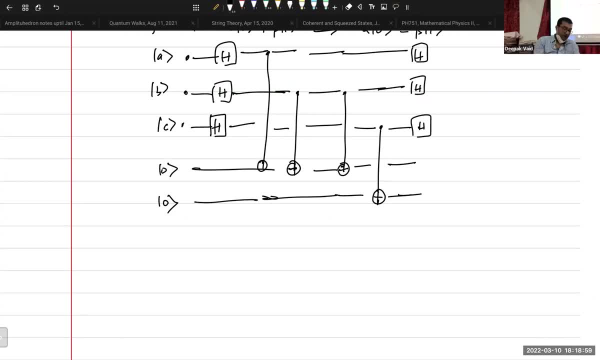 Right. So if you have the Z gate acting on a state- alpha 0 plus or minus beta 1, this will give you alpha 0 minus plus beta 1, this will give you a phase flip. so depending on the value, 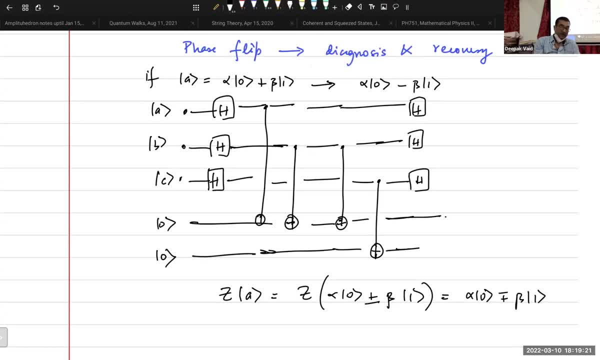 of your parities, Okay, So once again, you take your parity as your control, right? and then you go ahead and perform your phase flip on these states, okay, So in exactly the same procedure that we had earlier. okay, and then this one is the. 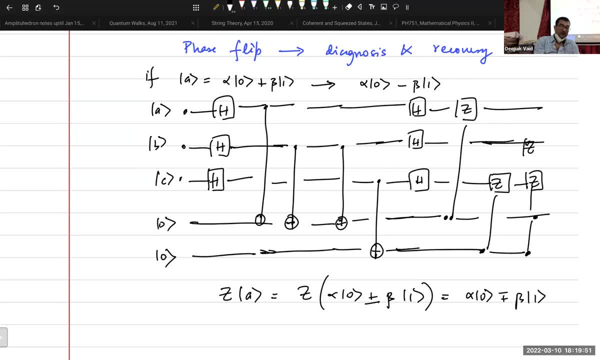 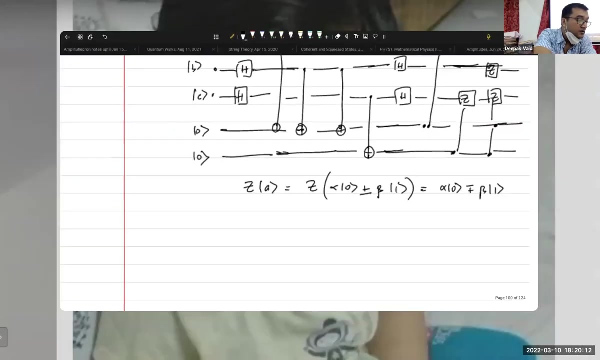 double controlled And then it will be Z Z, Z once again, to take into account the correction that we discussed. This is your phase flip recovery. okay, We can check that this works out in Quark, Let's see. 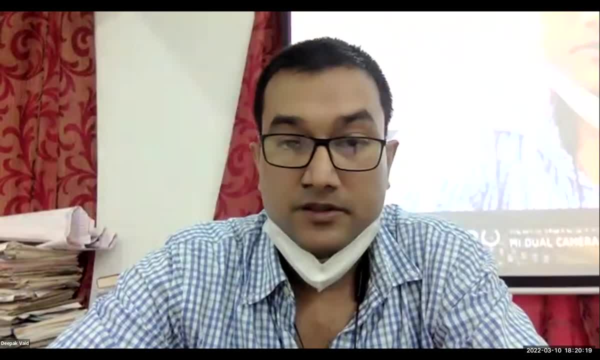 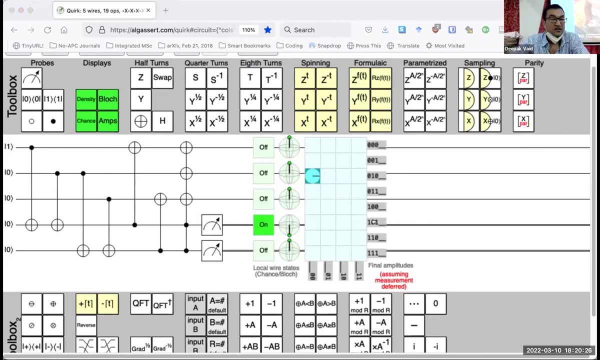 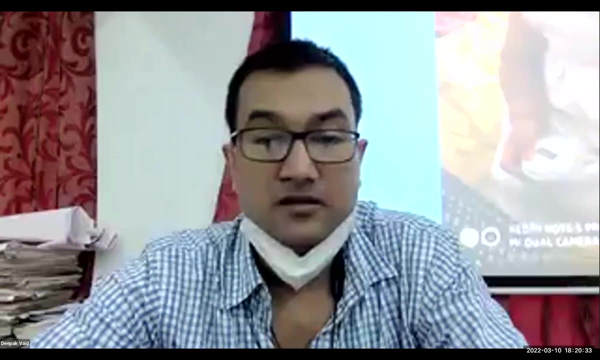 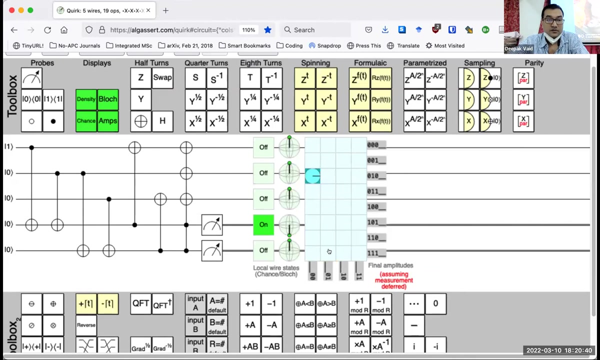 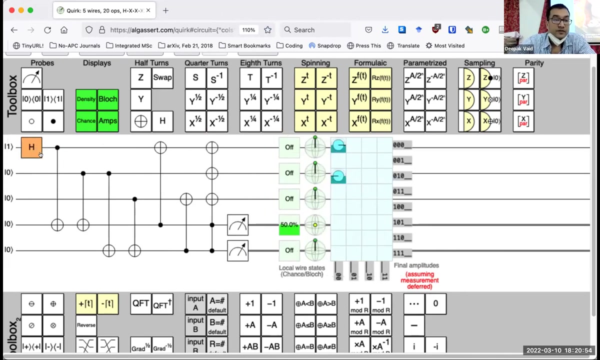 Let's see. Okay, So let's see. Is it showing? Is it not showing? Is it showing on your? okay, it's showing in Zoom, right? Okay, good, That's all I need. So I just need to modify this circuit for phase flip. 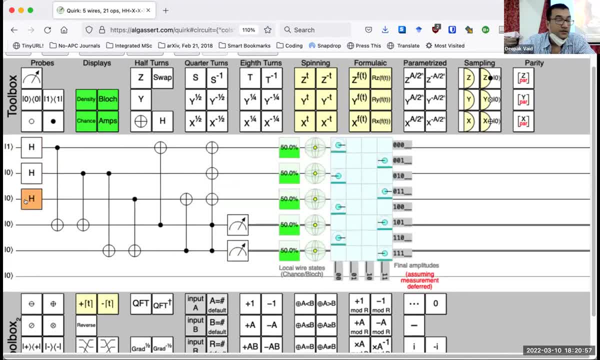 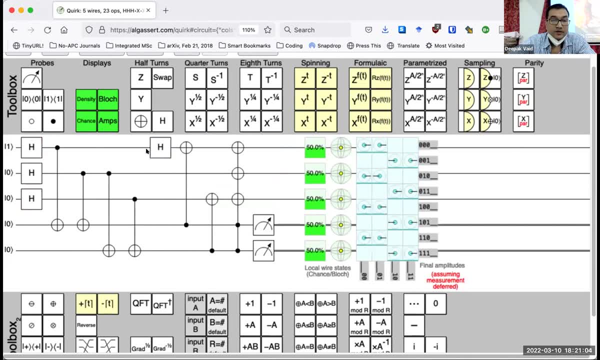 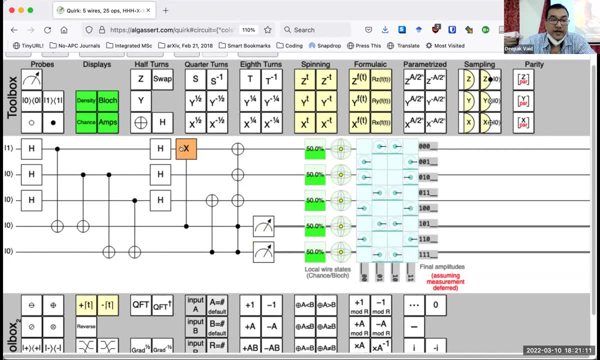 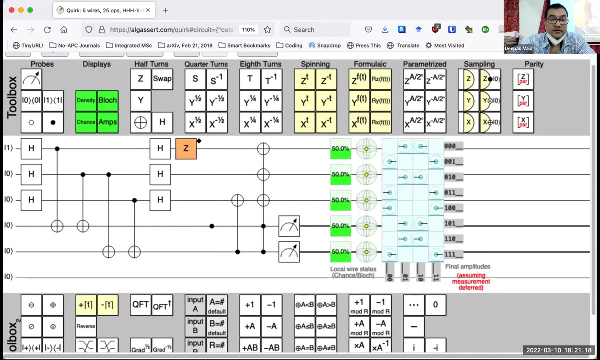 So I put three hard amards here right, And then I put three hard amards here right, And then, instead of X, what do I do? I put Z, Okay. So I put Z, Okay, Okay. 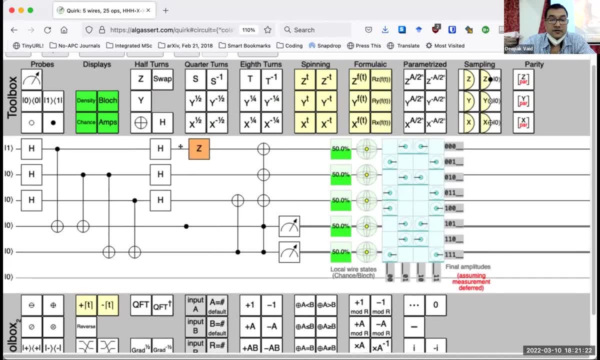 Make sure it is in. That's what the data has all been right. It's actually in there. Okay, Make sure that minus two. Make sure that minus two, Just like that. Thank you. So one is short, this is long. 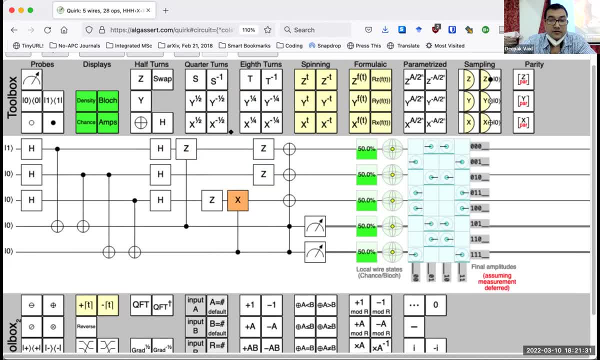 So it's one digit. This is a short, this is my long, this is something called 10.. You are going to have for 30 seconds, and you ourselves will see how long this will take. So here is the last place thing, right there. 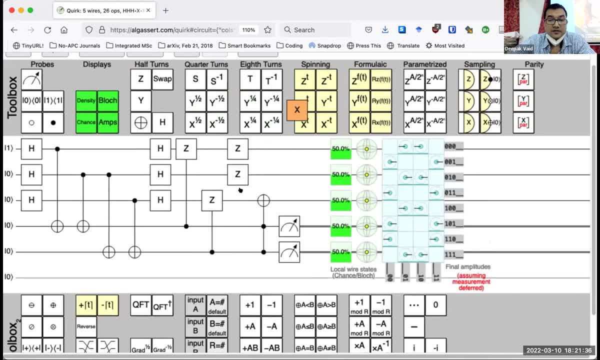 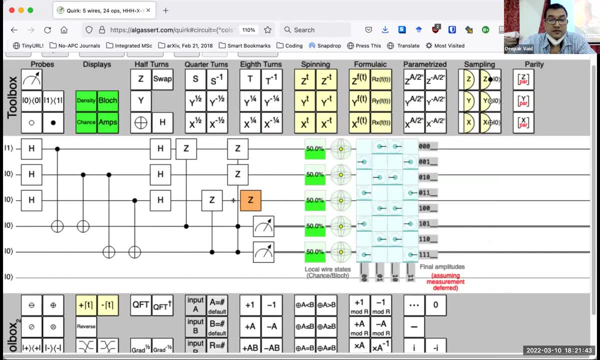 Is that what you have to do? Okay, So we are going to have this Kelvin matrix here, So I'm going to have this other one right here, This resistance going to be more than nine minutes. We could do that right now. later. 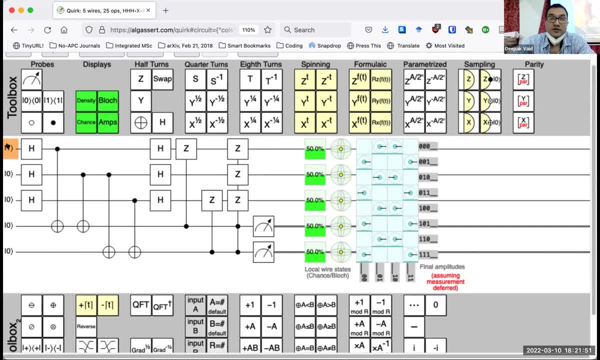 uh, let's check for a face flip error. for that, what should i do? i should take my, uh, my state right one, and uh, so i have zero, zero, zero. right now i want the phase to change. so where is the phase gate? let me put an error. 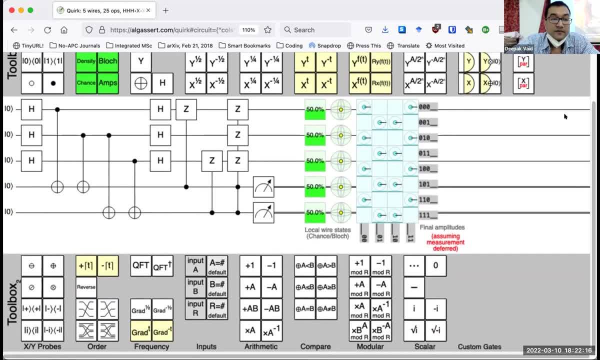 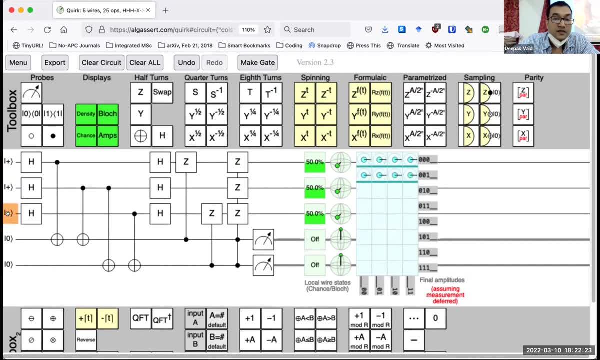 here. okay, yeah, let's say we can do that. let's take two pluses and one minus, right, and what is the output? output you can see is is three pluses, right, what if i take two minuses and three pluses? i get three minuses. 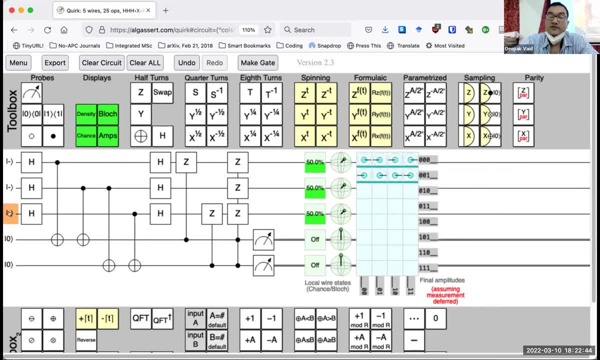 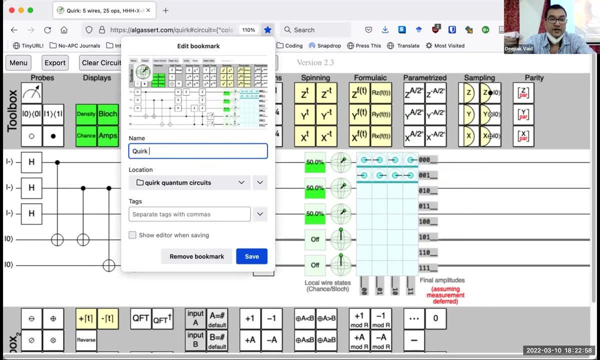 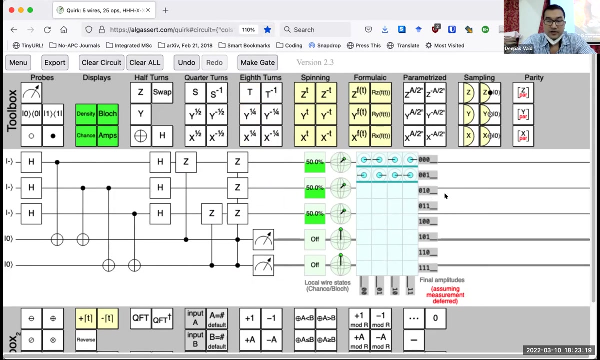 right, it's working right. once again, i save it in my bookmark folder. i call it the face clip, error correction b qubit face with error correction. right, so i think i'll stop here. i think this is enough for one day. zoom people- are you? are you? is this clear to you what's going on here? 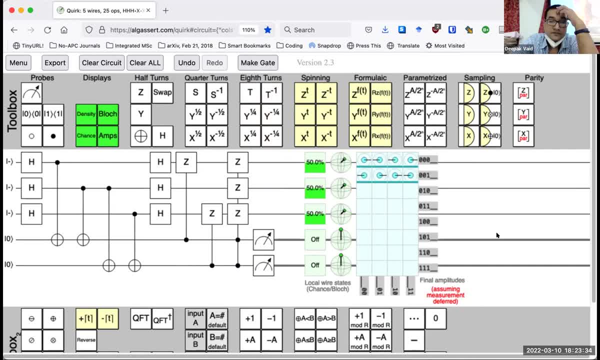 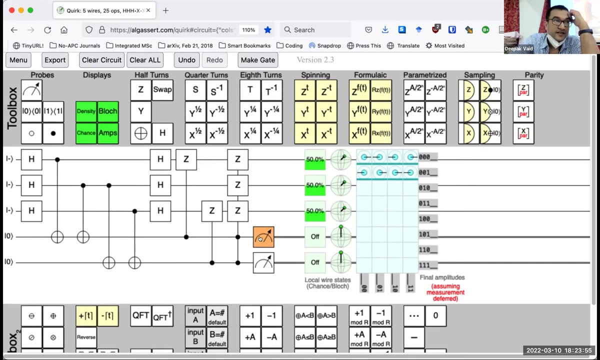 if there is any doubt, please ask me. um swetha are you? are you following what's going on? uh, you have any any doubts? please ask me. that's a great. that's a great question, right? this is a great question because the principle of deferred measurement 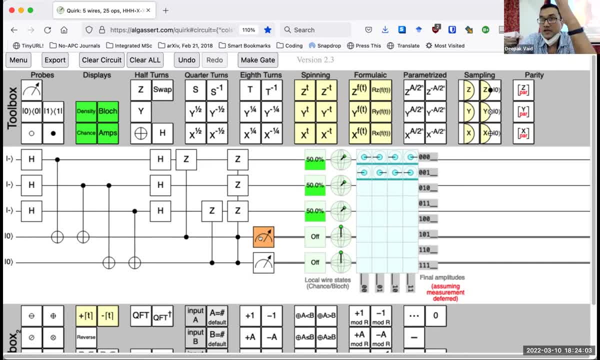 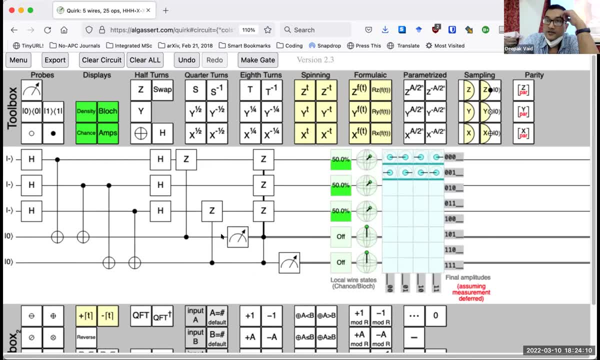 says that, if it's correct, you should be able to move even one of the measurements. i should be able to move it here, right, so i'm moving it between the right here and the left here, just as you said, right so? or i could put it here: 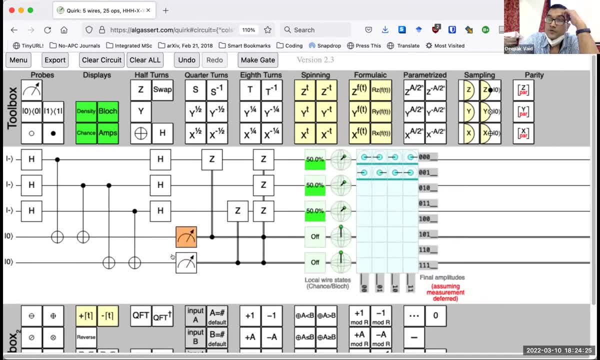 now the first. so here, in this case, what i'm doing now is i'm performing the measurement and then turning all my parity check qubits into class qubits. right, let me just uh, make this plus minus minus. this gets converted into minus minus minus, it's. 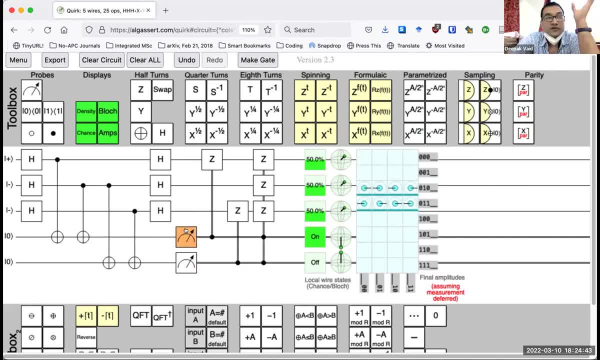 working in the principle of deferred measurement, I should be able to take the measurement on individual qubits and translate that There should be no restriction. So again, this is a very good point. I should be able to take the single measurement and I should be able to put it not just at: 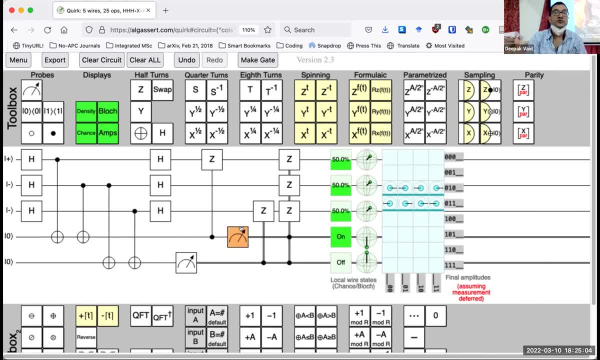 the end, but I should be able to put it anywhere in between also. So I take this one measurement and I put it in between. My code is still working. I take this second measurement and put it here. My code is still working. So I have minus plus plus. minus plus minus gets converted to minus, minus, minus. 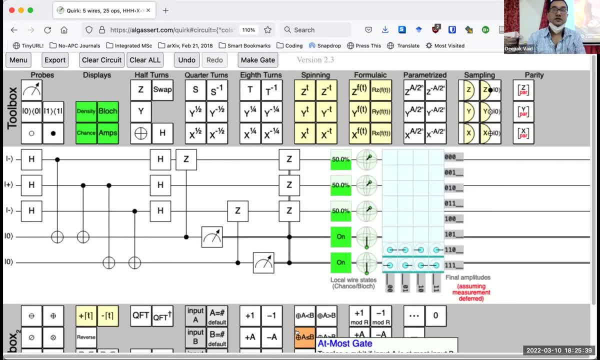 So the principle of deferred measurement is also a linear statement. That means you can apply it to different subsystems individually. It obeys linearity. If it didn't obey linearity, we would be in trouble. Any other doubts? I don't know if this clears the 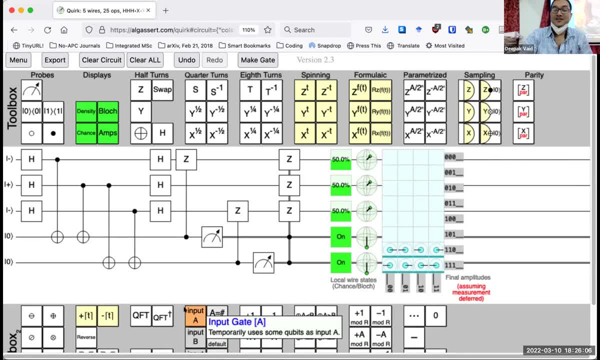 No, because if you move it to the beginning then your CNOTs will not have any effect. These are CNOT gates. CNOT gates are quantum operators. If you move your measurement to the beginning, then you will collapse. these ancilla qubits. 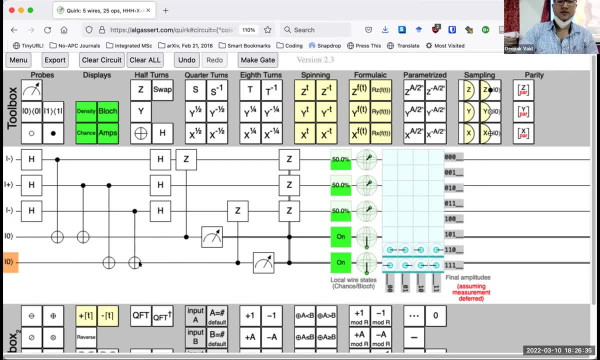 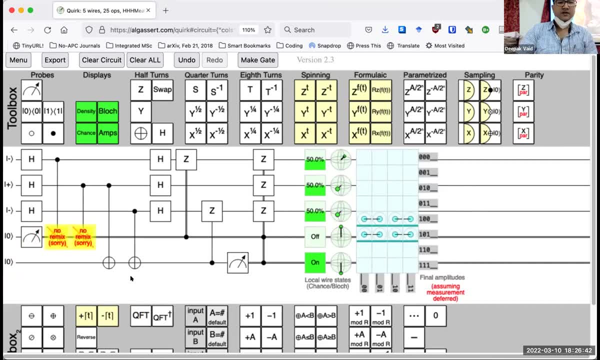 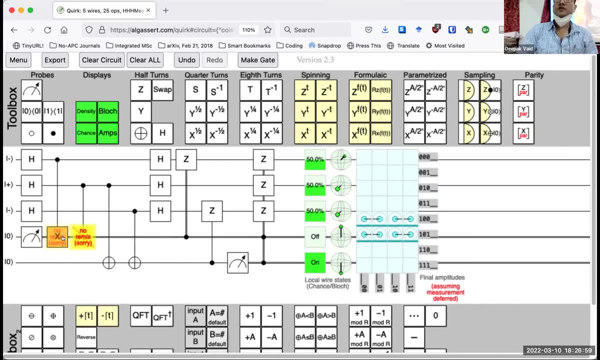 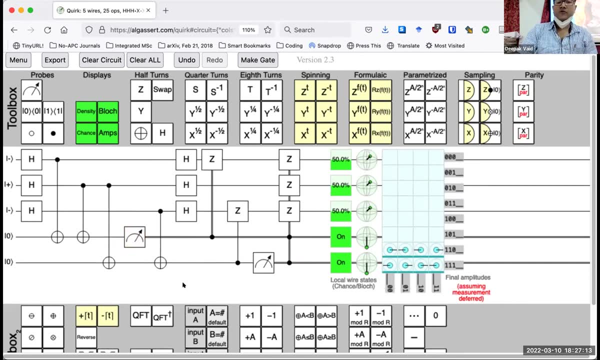 us to do this operationally. So what if I put this measurement here? Does that work? No, it works. But again, the reason it works is because I am already done with the first qubit. The first parity check is already done, So I can always measure it here. So these are. 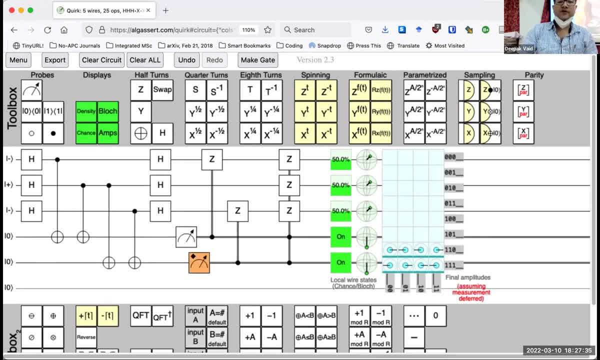 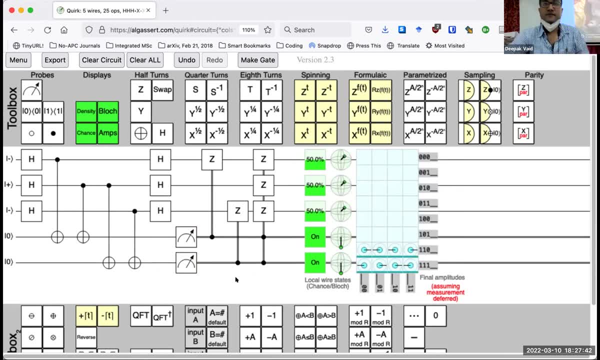 all kinds of very interesting and non-intuitive things that one can do in quantum mechanics, and these are all the consequence of the linearity of quantum mechanics. Does this clarify your doubt? I mean, do you have any other doubts? Please ask, because this is really. 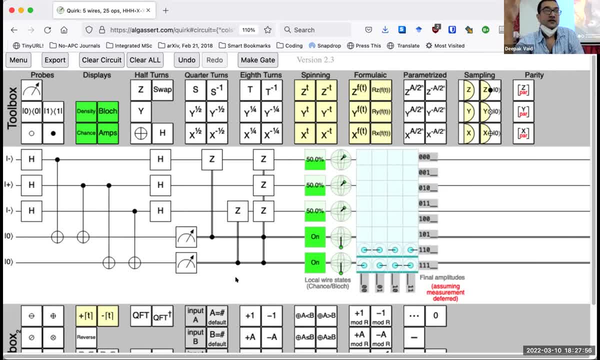 good Anybody else. Well, it is a conditional, That's all. It is a conditional. there is a little device.